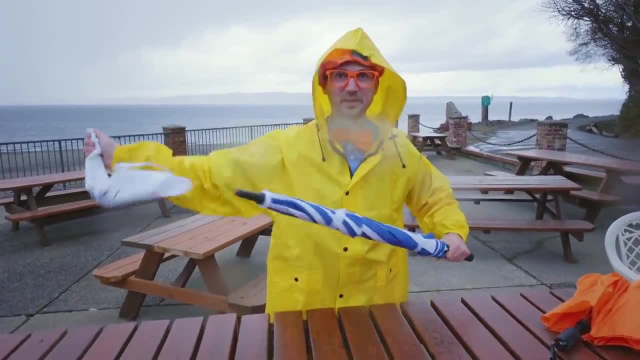 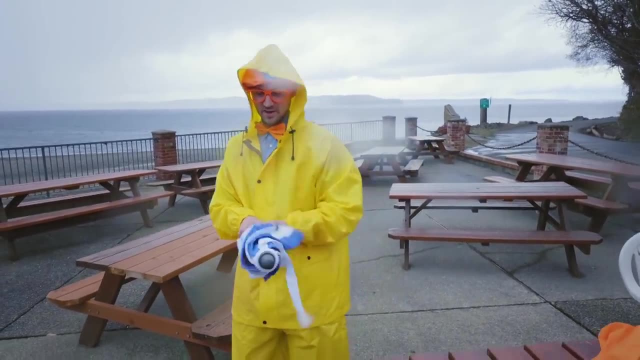 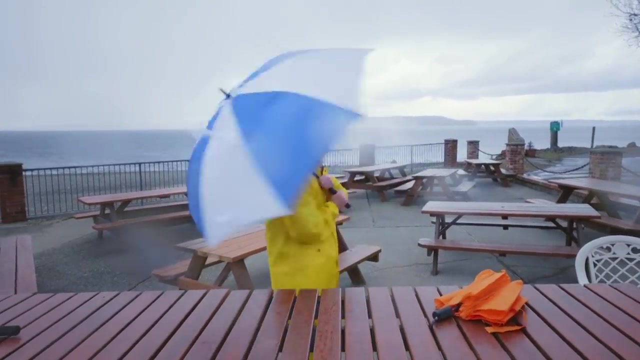 What's this next one? Yeah, the first umbrella. The first umbrella was really small And this one, whoa, is so big. Whoa, Whoa, Check it out. Whoa, Woo-hoo, What color is this umbrella? 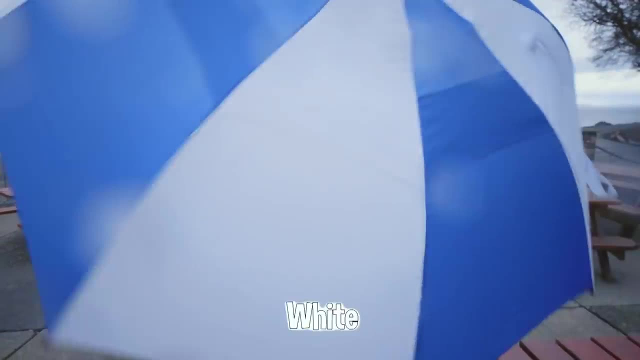 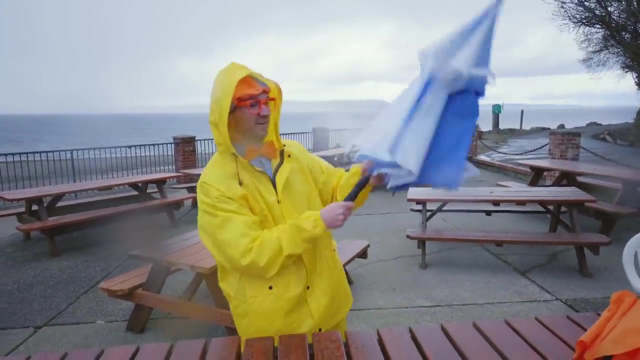 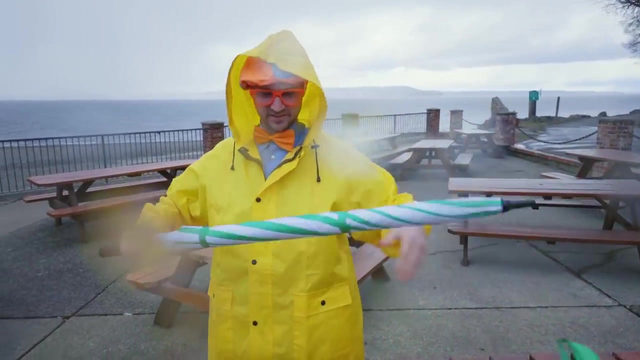 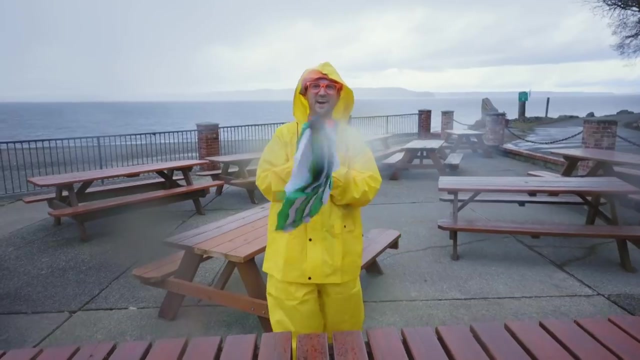 Yeah, Blue and white, Woo-hoo, Whee. Okay, let me put this down before I fly away. Okay, and for this umbrella, whoa, Check it out. Yeah, another big umbrella, And the colors of this umbrella are: 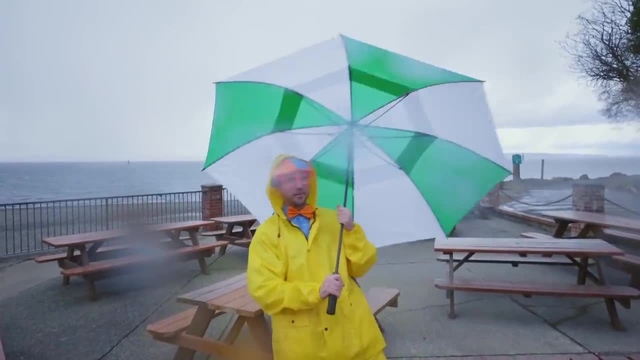 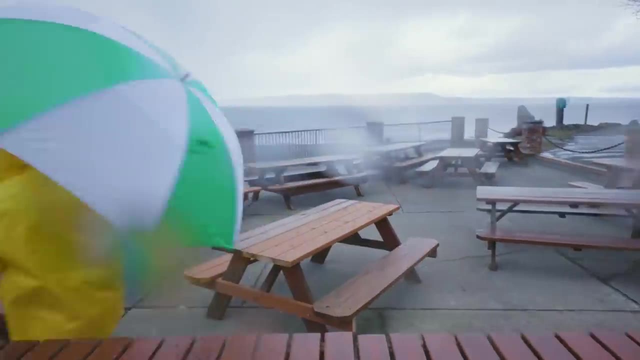 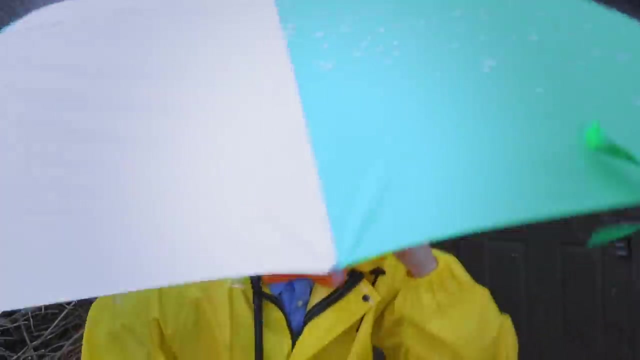 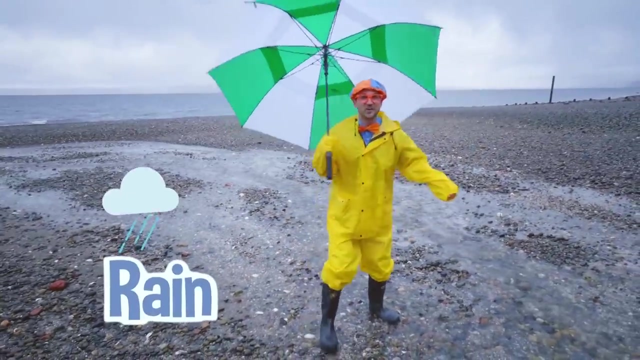 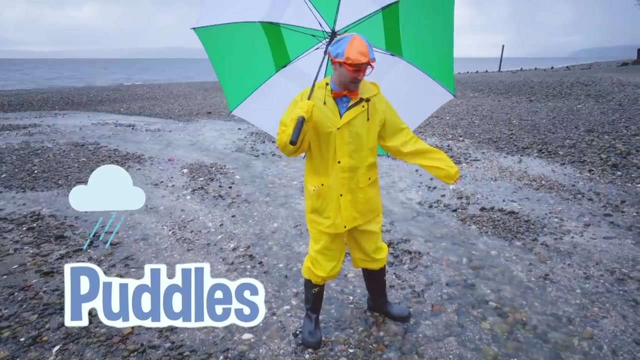 Whoa, It is so stormy out. Yeah, It is white and green. Woo-hoo, Let's go. Wow, I love the rain. The cool thing about rain gear is you can even splash in the puddles and streams that were created by the rain. 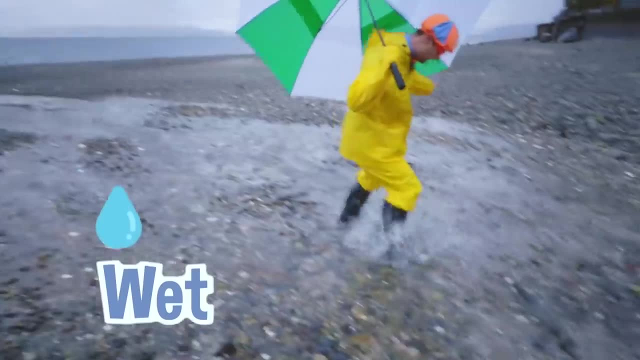 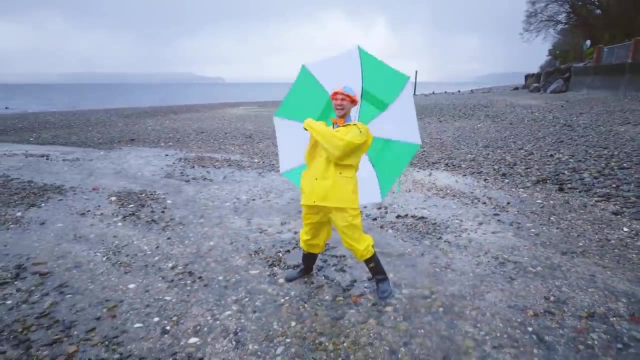 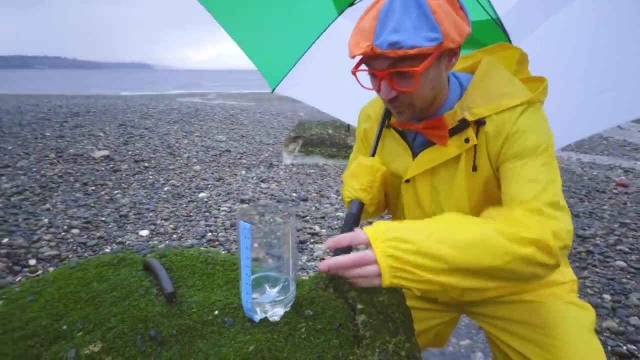 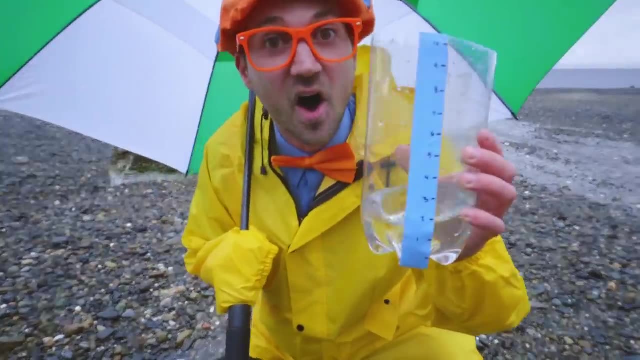 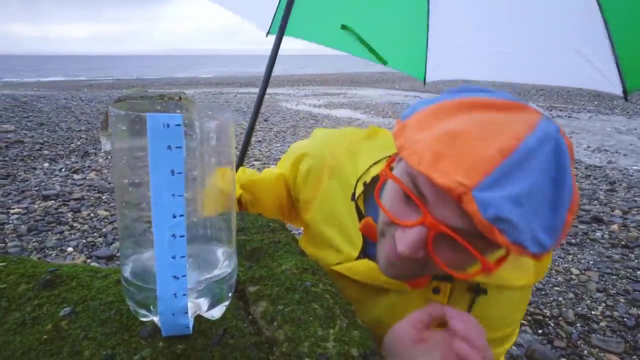 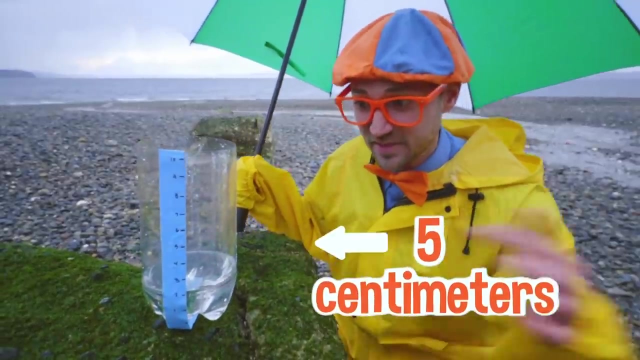 Wow, Do you see this? Yeah, this is my rain collector. I set this out earlier, before it started to rain, And then all this rain collected from the top. Do you see how much it says? Wow, Yeah, it says about two inches. Yeah, that's just over five centimeters of rain. 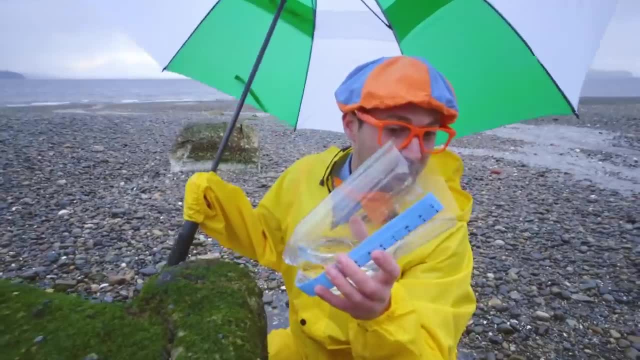 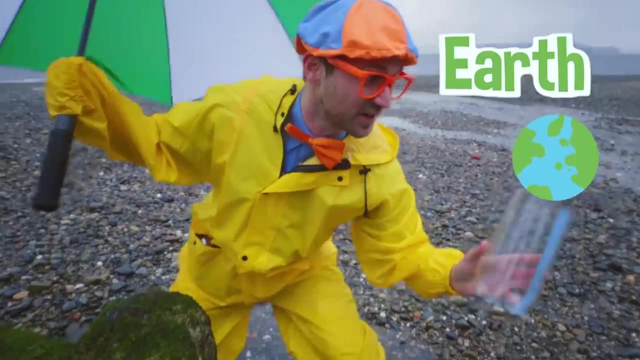 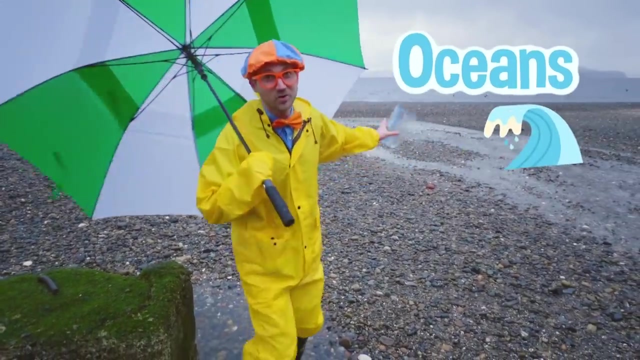 Wow, That's a lot of rain. Okay, I'm gonna pour it back onto our planet Earth, because when the rain falls on our planet, it's really good for it. It helps keep all the plants nice and moist and our oceans nice and full. 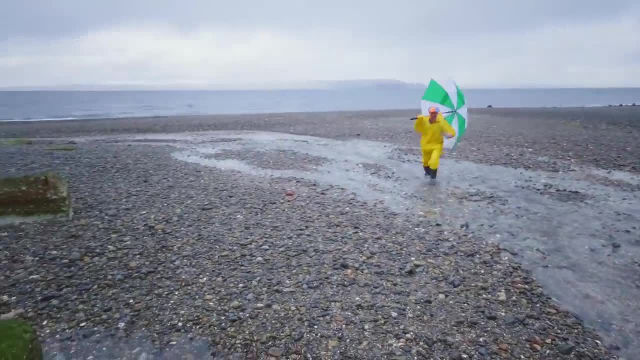 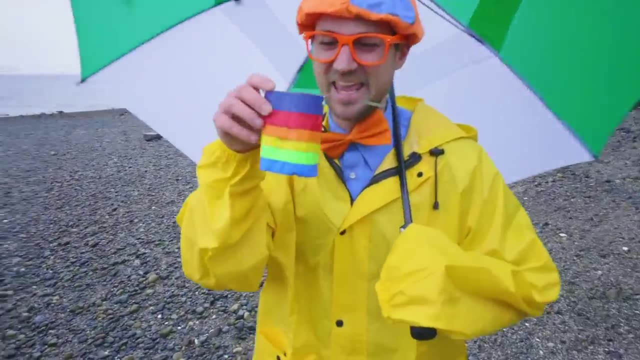 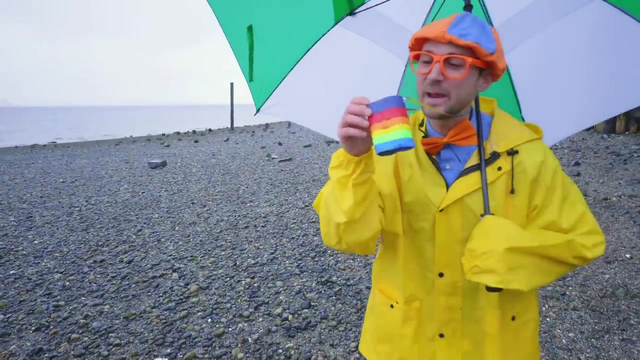 Woo-hoo, Woo-hoo. Okay, Hey, Check it out. yeah, these are my rainbow oculars. Yeah, isn't that cool. Yeah, they're the colors of the rainbow. Have you ever seen a rainbow before? 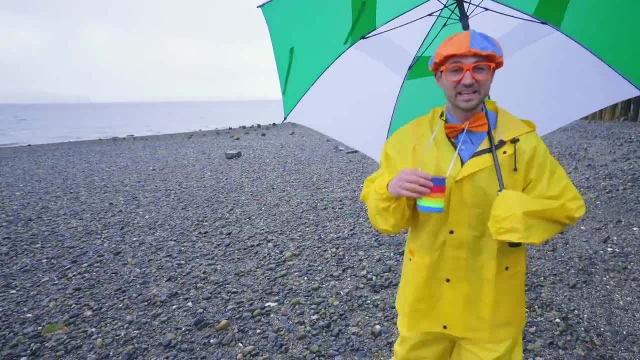 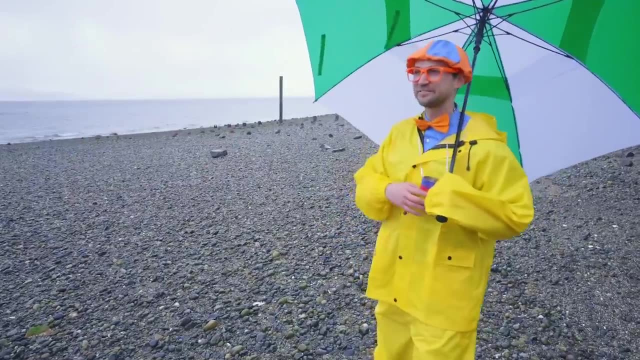 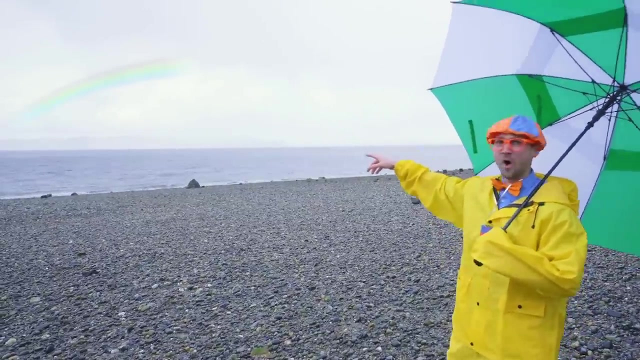 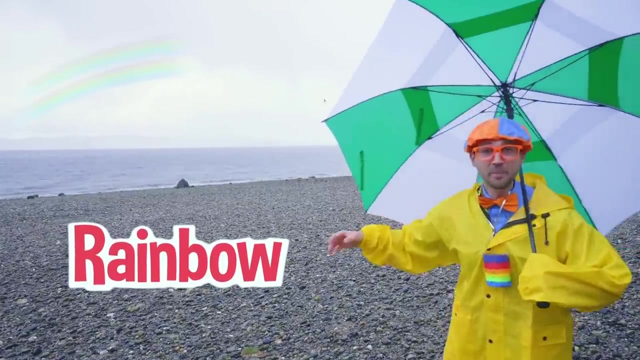 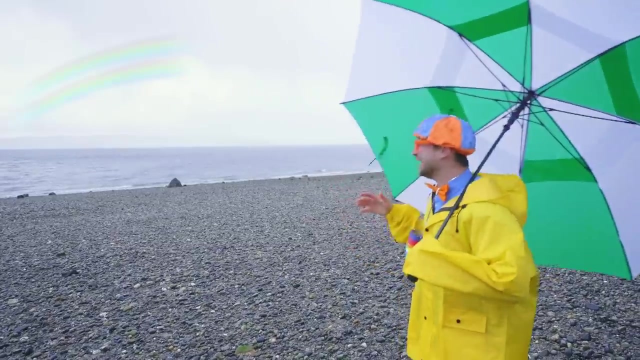 Yeah, they love to come out after it rains. Yeah, a rainbow is an arch of colors made by light and water. Let's see if we can find one. Oh, oh, oh, oh, oh rainbow, oh, a double rainbow, oh, oh, oh. it's full on, oh, oh. 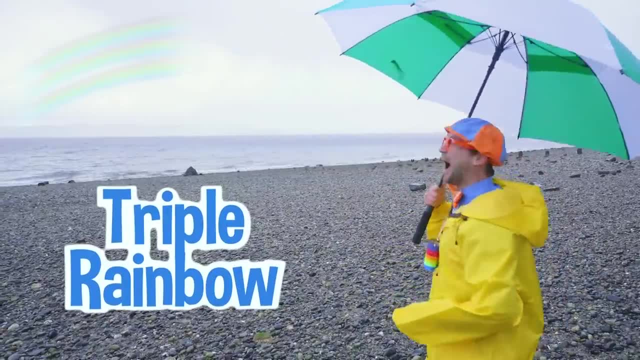 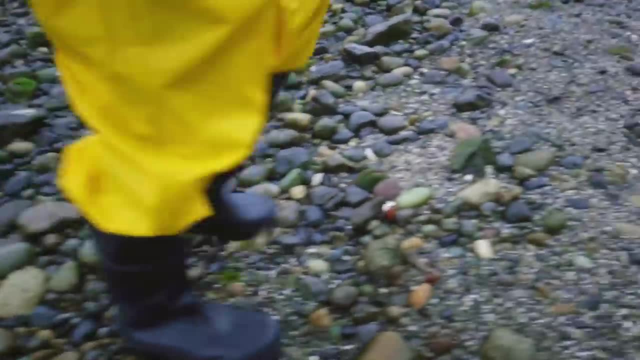 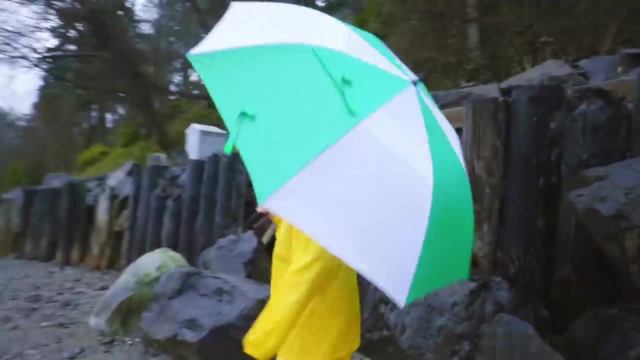 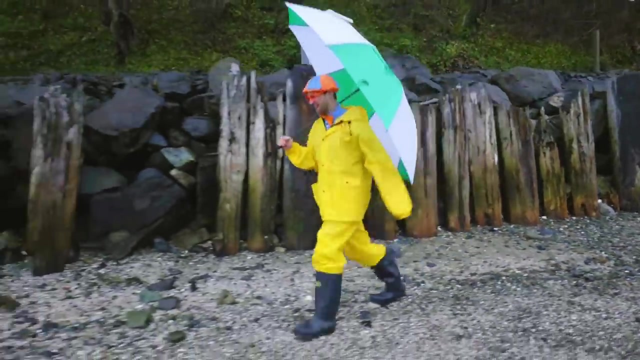 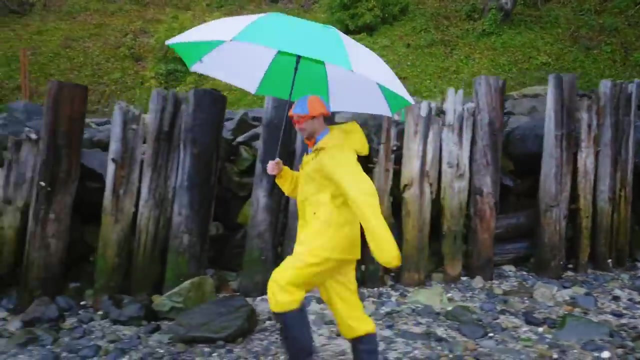 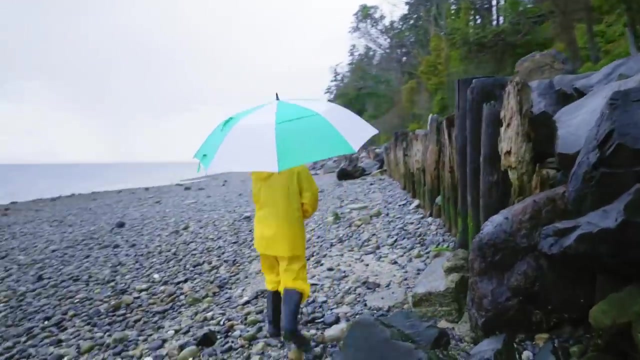 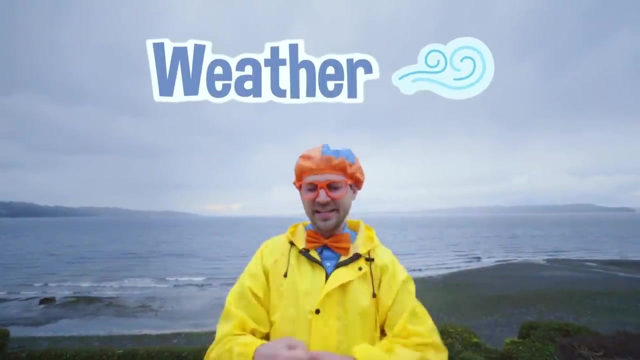 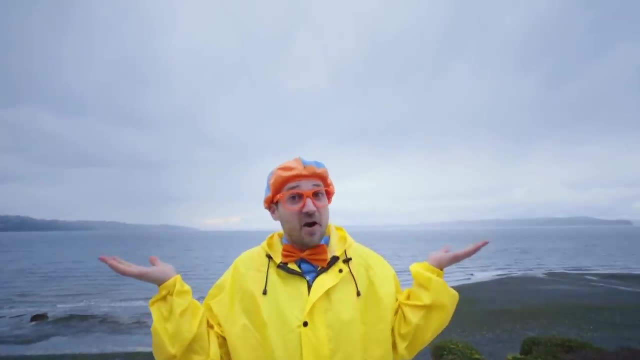 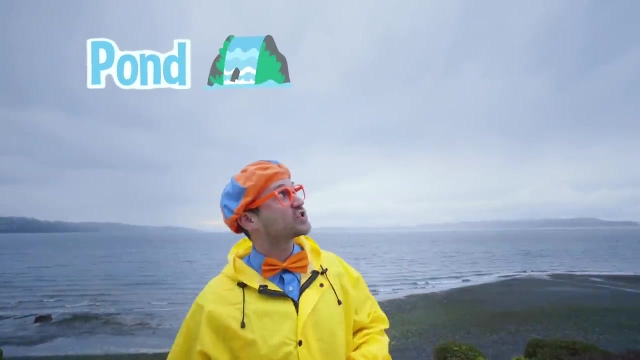 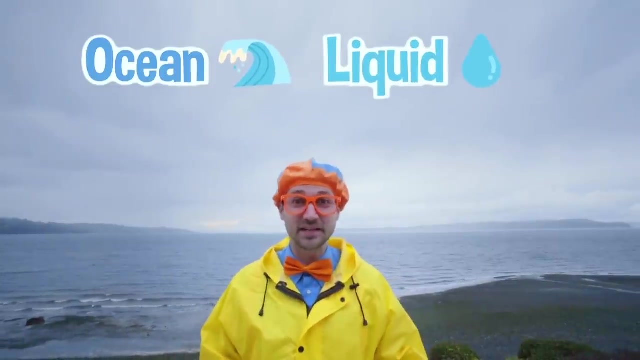 Hey, have you ever wondered: where does rain come from? Well, let me tell you. Okay, let's start with water in a pond or a stream or the ocean. Yeah, water is a liquid at this time and place. And then water goes, what's called evaporation. 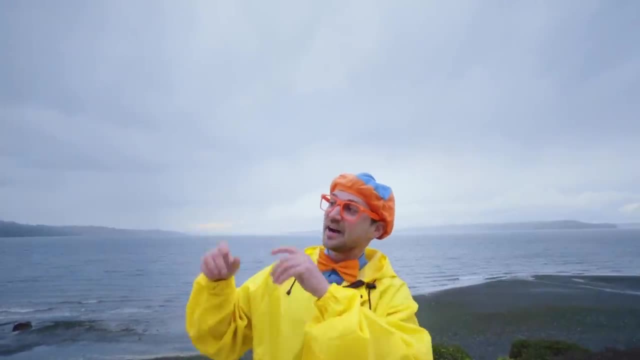 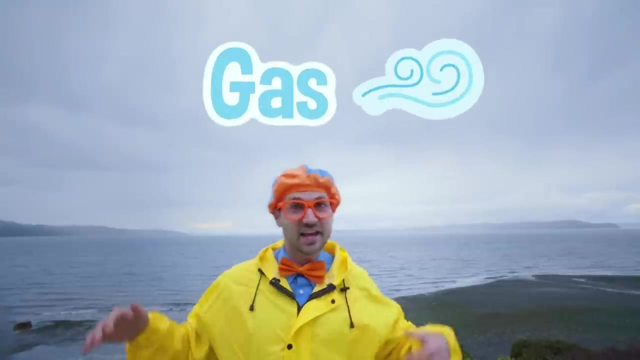 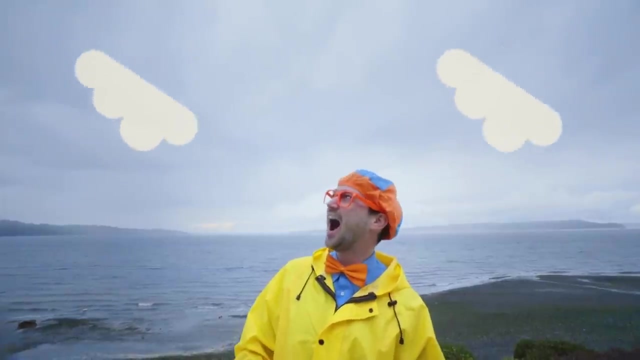 Yeah, evaporation is when the water becomes these little tiny particles and goes up in the air. Yeah, it turns into a gas, goes up in the air and then turns into some clouds. Whoa, yeah, clouds are awesome. Whoa, look at that cloud. 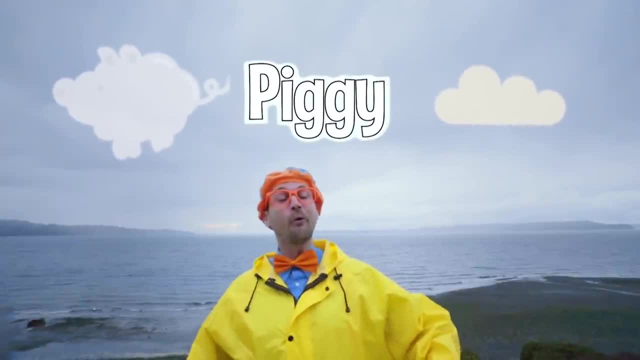 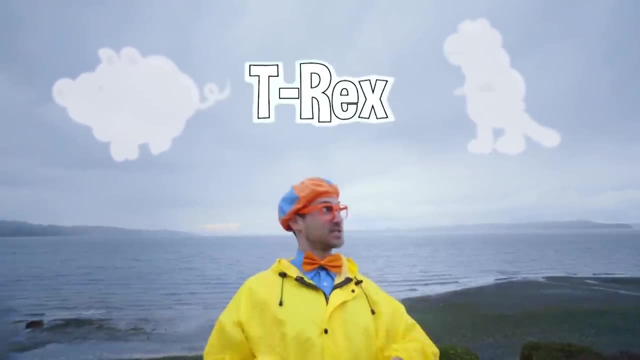 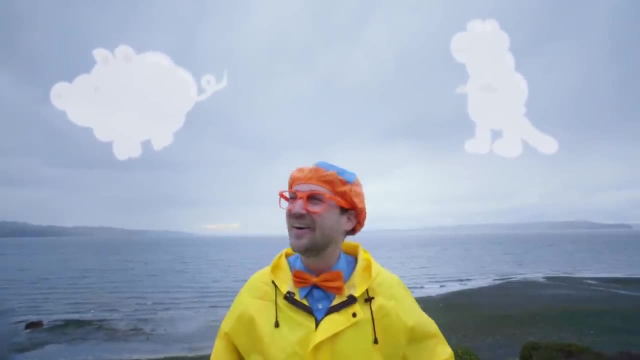 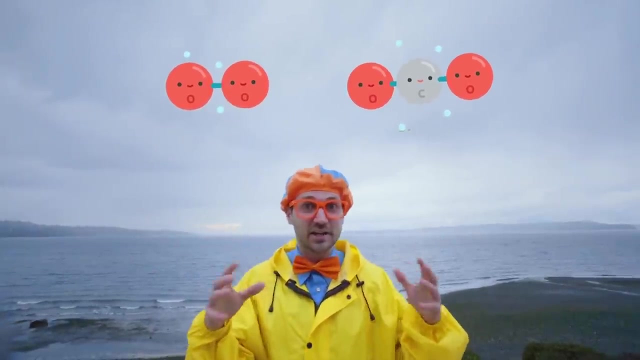 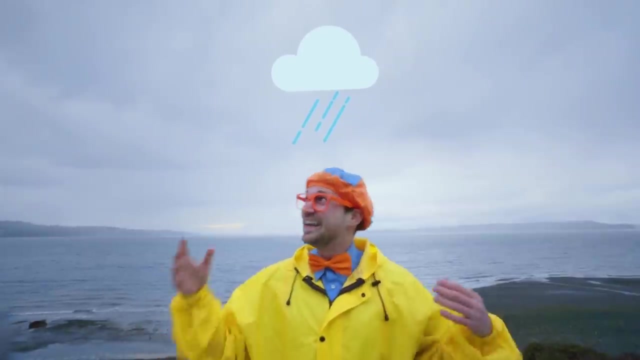 Wow, wow, Ha, ha, ha, wow. And then all this gas water starts to come closer and closer and closer, Yeah, and those clouds start to form into liquid water again, Yeah. and then rain starts to fall. Whoa, yeah, it's raining. 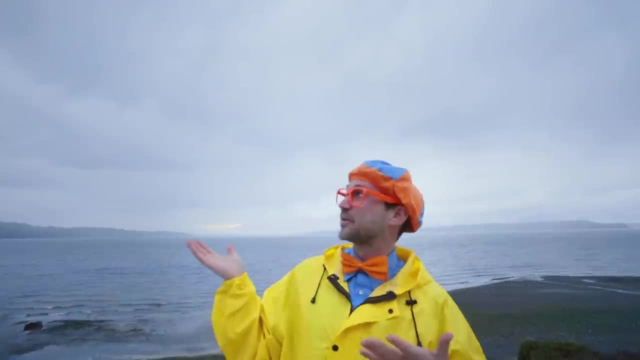 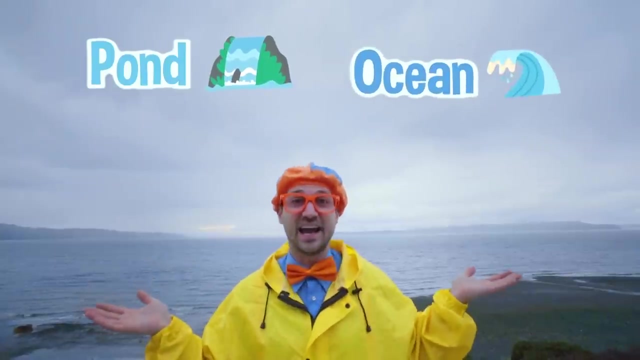 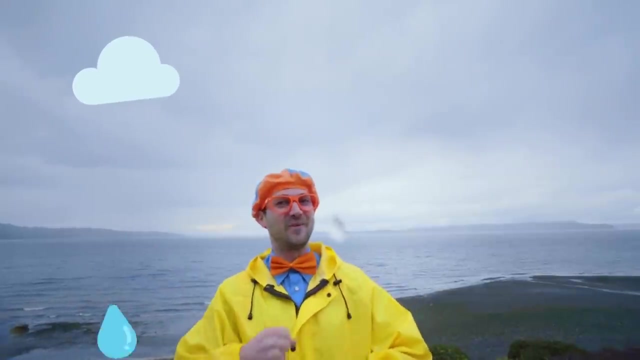 Whoa. And then they create puddles and streams and ponds and the water goes back into the ocean again. And then the cycle goes over and over and again and again. Wow, that water cycle is so great. Woo hoo, Ha ha. 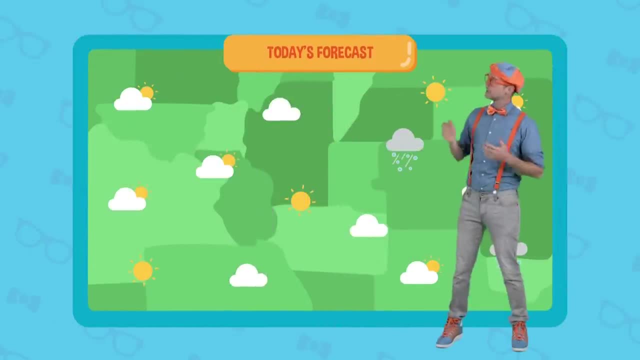 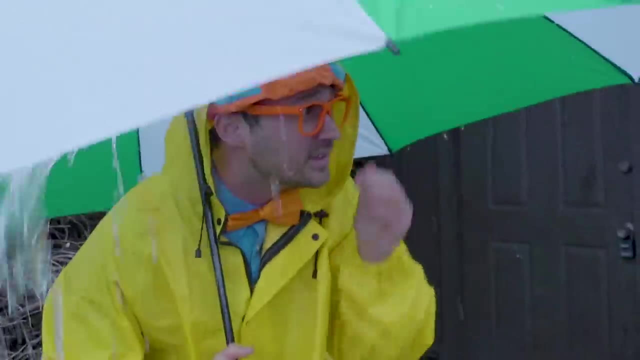 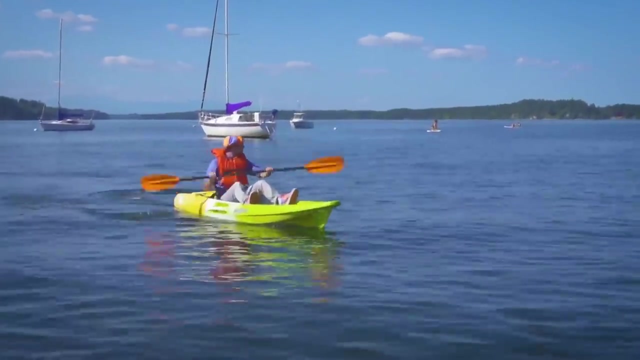 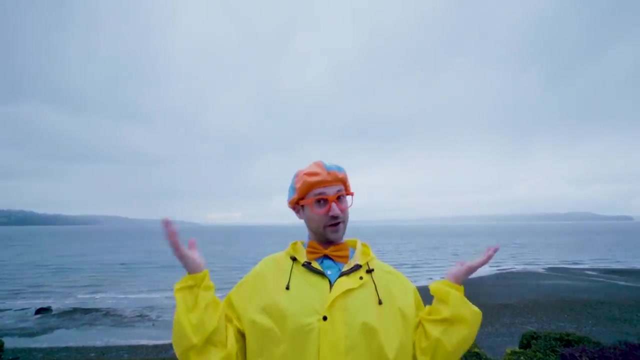 Today's weather forecast: sunny skies in the morning, followed by storms in the afternoon. Don't forget your umbrella. The morning looks nice- lots of sunshine, clouds of white and a bright blue sky- But the sky's turning gray. there's wind and some rain. 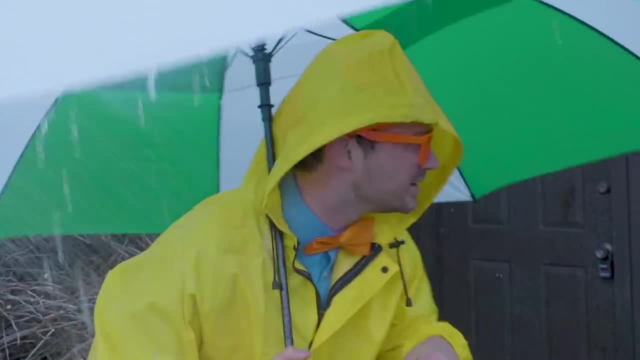 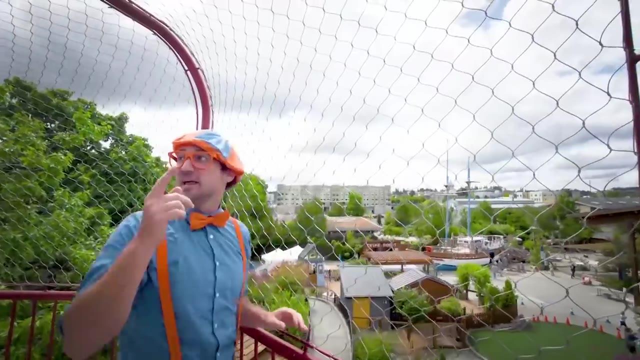 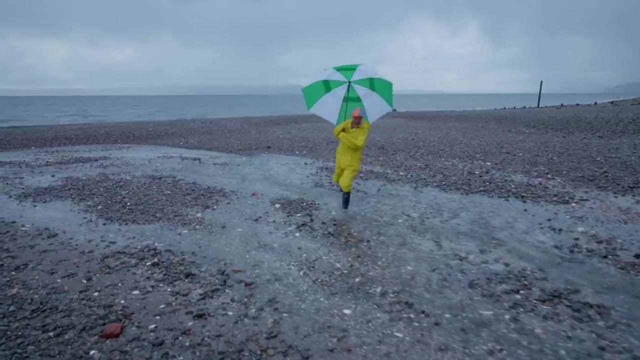 It looks like it's gonna be a stormy day. Weather weather- all kinds of weather like sunny, breezy, cloudy, warm, pleasant days. Weather weather- all kinds of weather like windy, rainy, stormy, hot, muggy days. 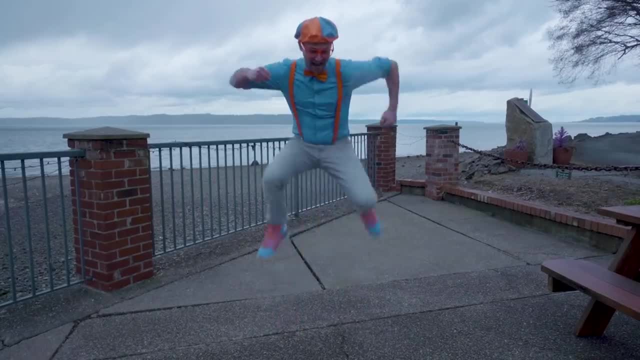 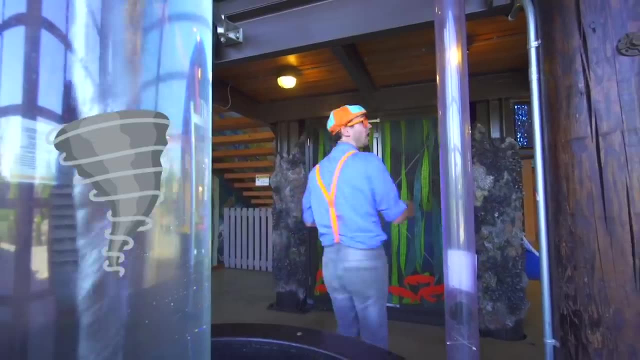 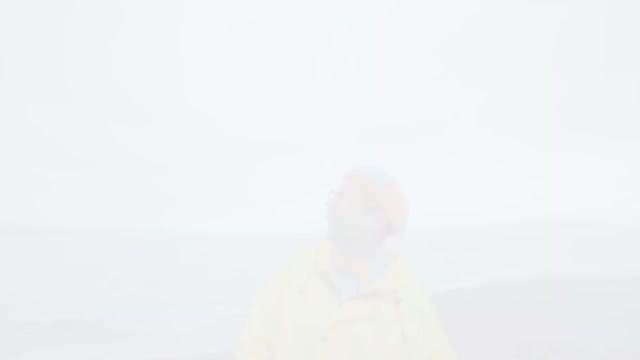 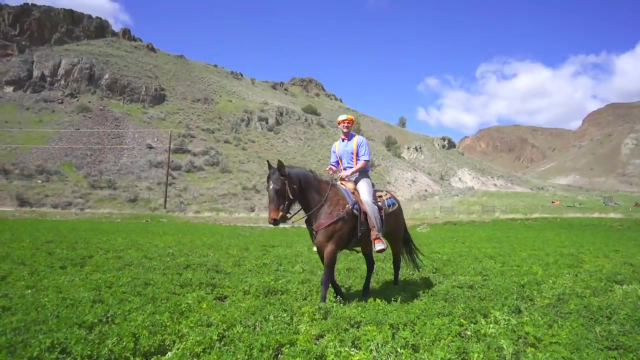 A lightning bolt, that thundering sound. There's a storm coming any moment now: Tornadoes, hurricanes and floods. Sometimes weather can be dangerous Weather weather, all kinds of weather, like sunny, breezy, cloudy, warm, pleasant days. 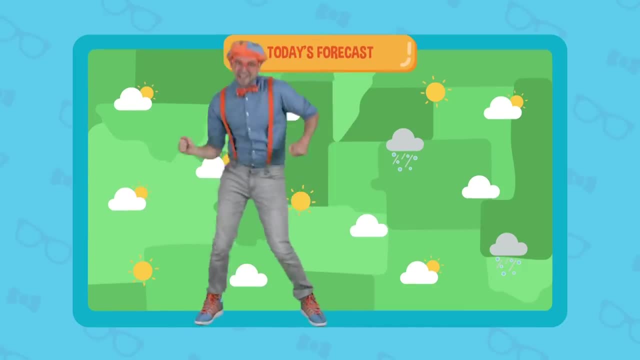 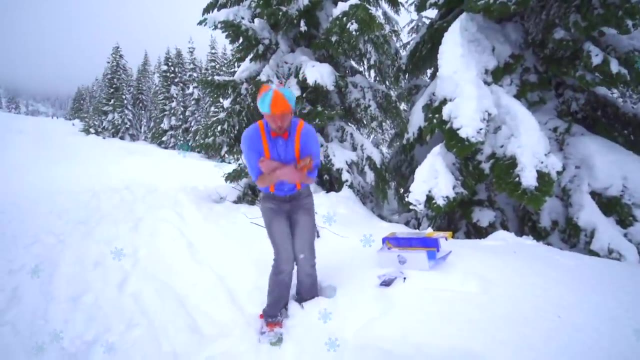 Weather weather. all kinds of weather like windy, rainy, stormy, hot, muggy days And, when it's really really cold, Snowflakes, winds and storms. Snowflakes will fall from the sky. Snowflakes will fall from the sky. 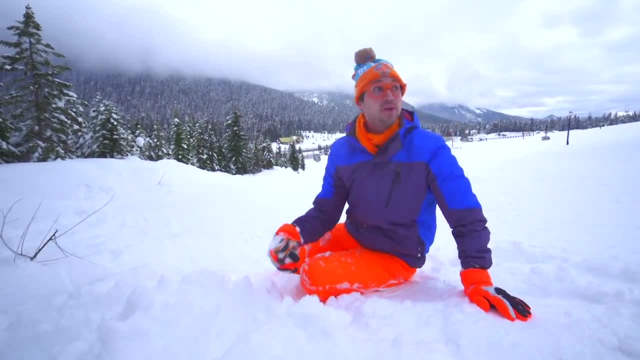 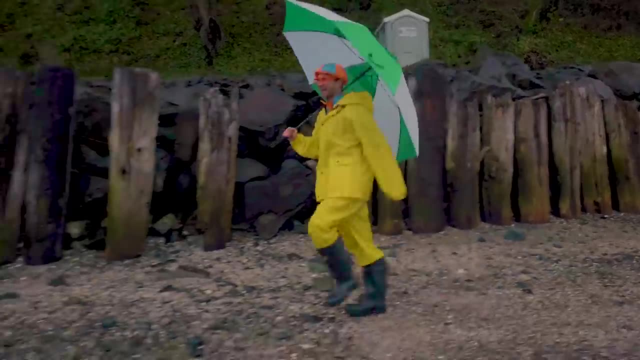 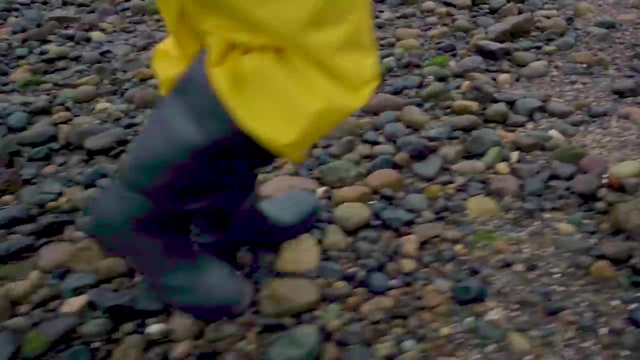 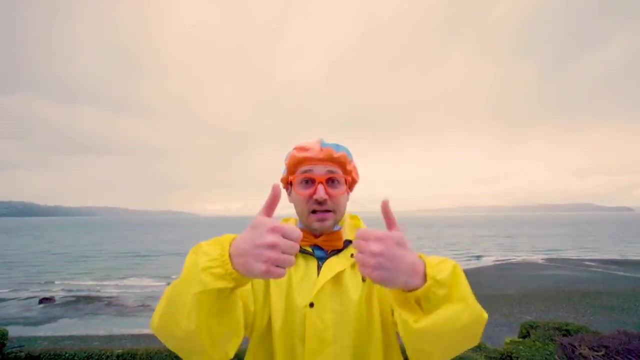 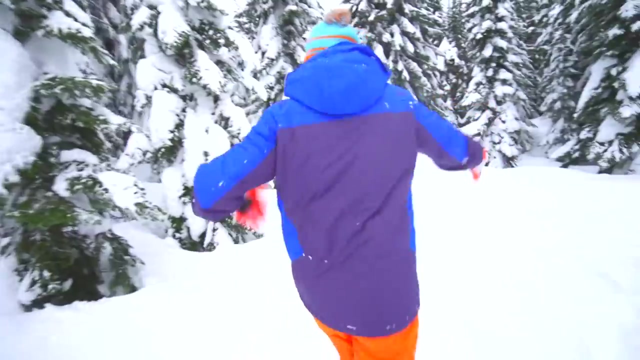 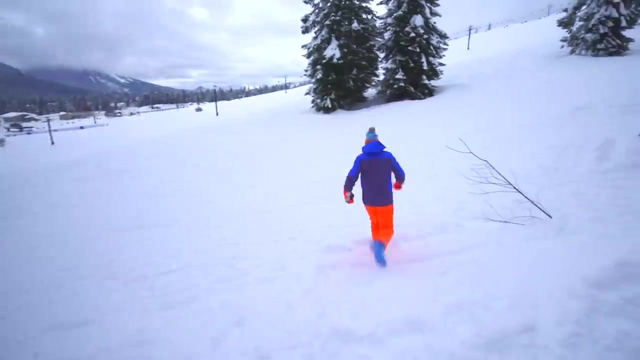 Everything goes quiet and everything is covered in white. Hey, the rain has stopped and the sun's shining again. plesh. Weather weather- all kinds of weather, Like snowy, icy, blizzard, cold, frigid days. Weather weather- all kinds of weather. 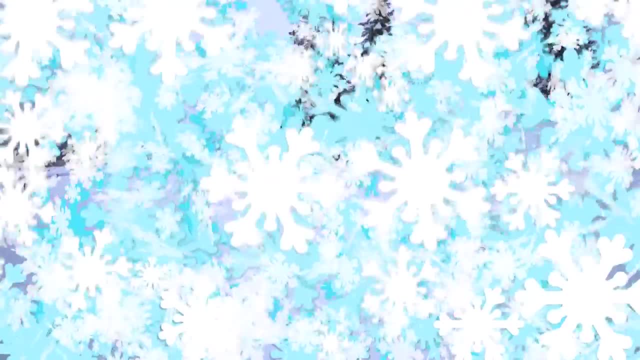 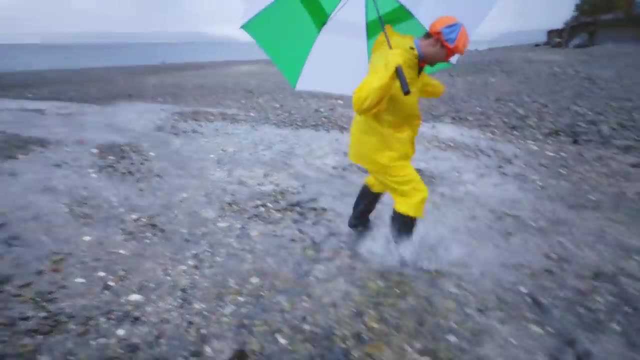 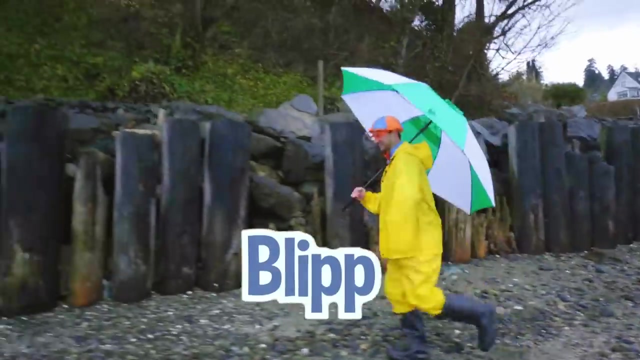 Well, this is the end of this video, But if you want to watch more of my videos, all you have to do is search for my name. Will you spell my name with me? Ready B-L-I-P-P-I, Blippi, Good job. 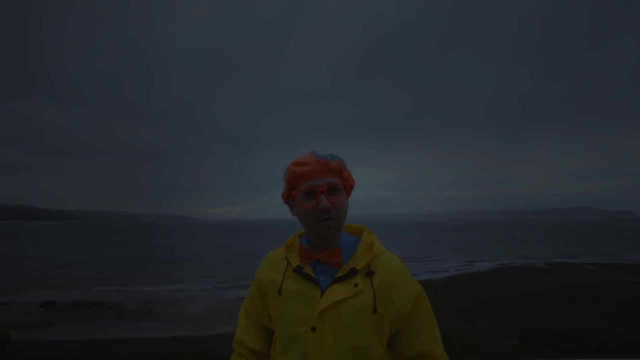 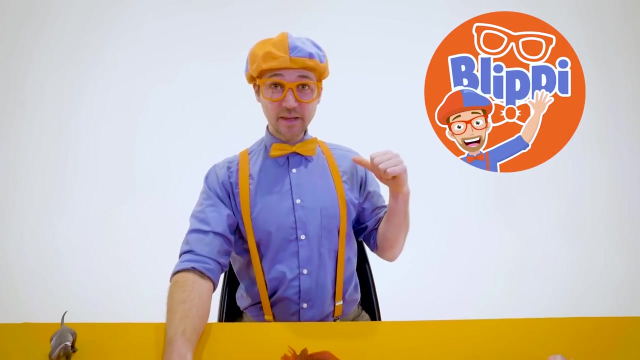 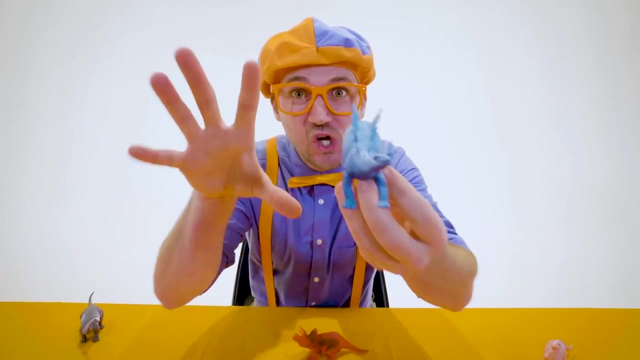 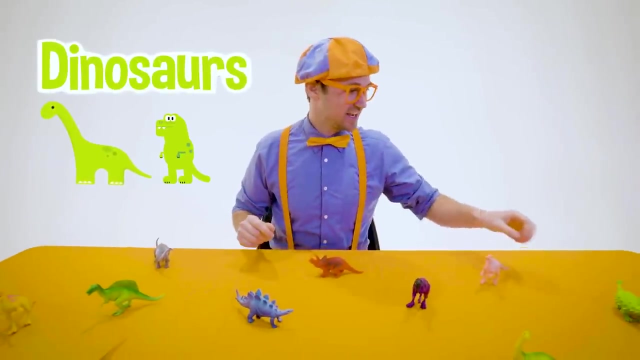 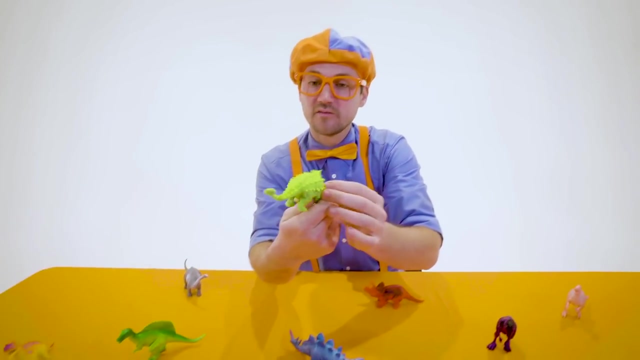 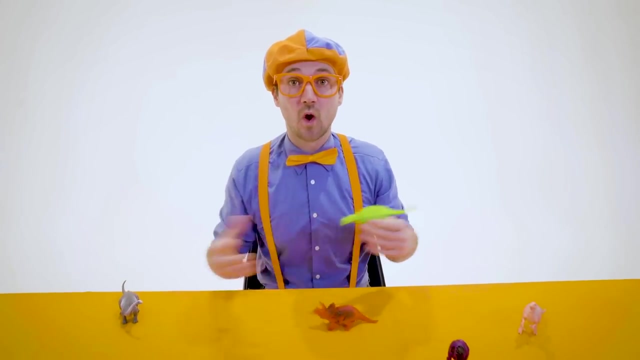 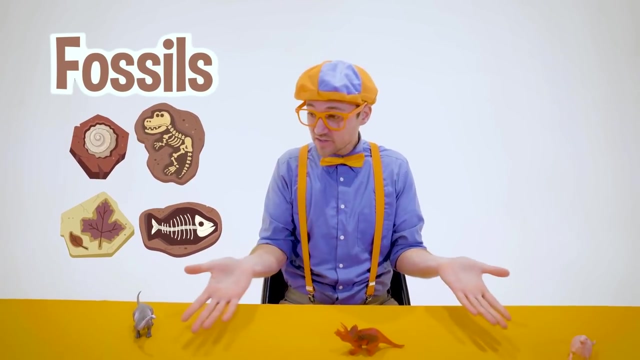 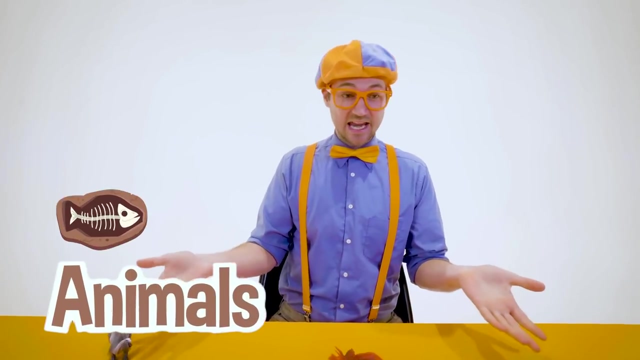 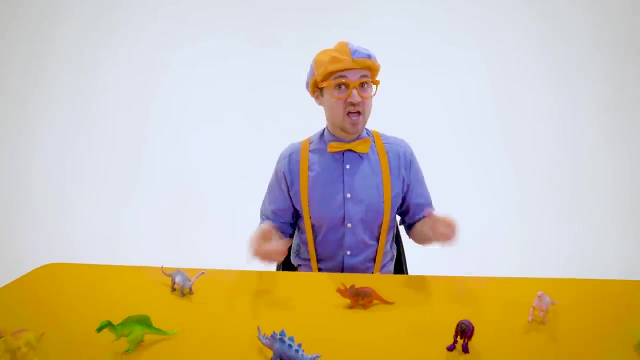 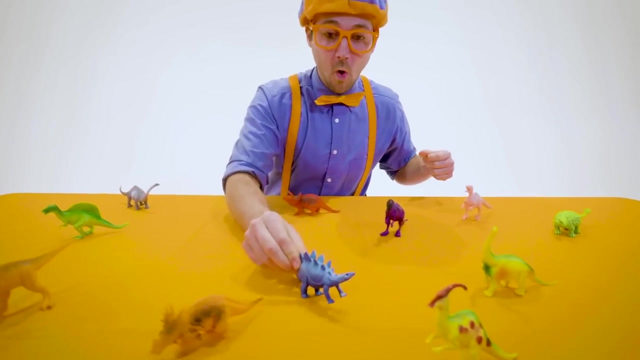 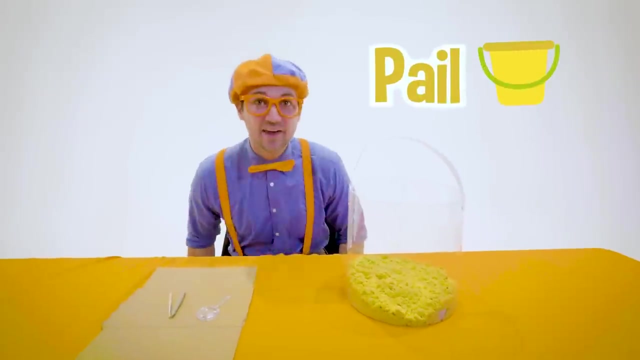 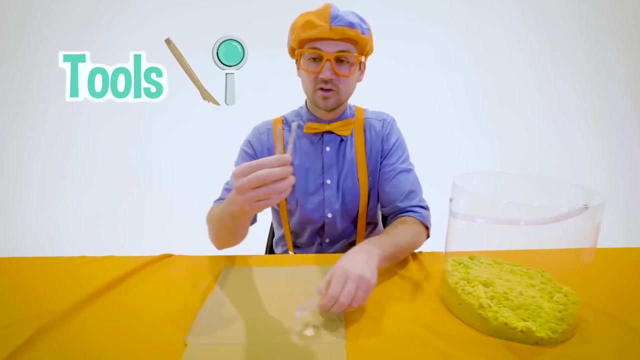 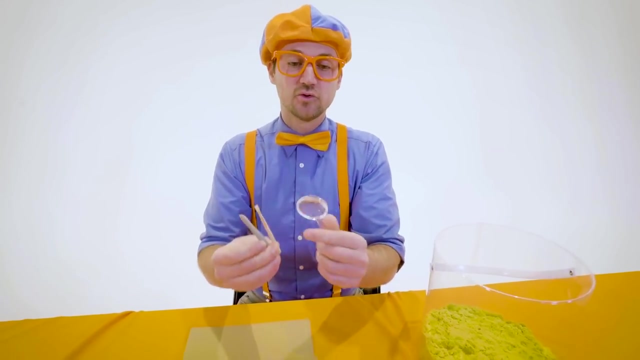 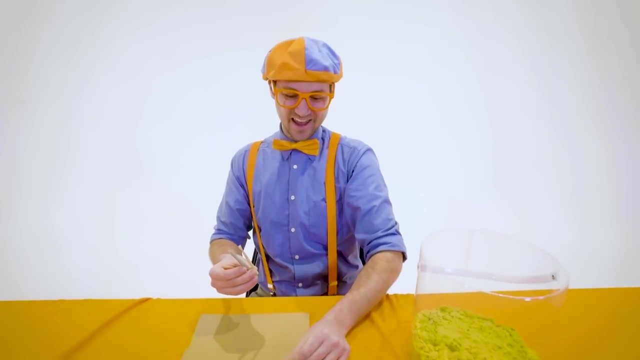 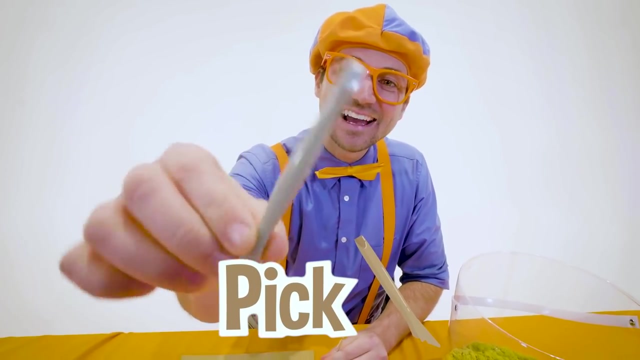 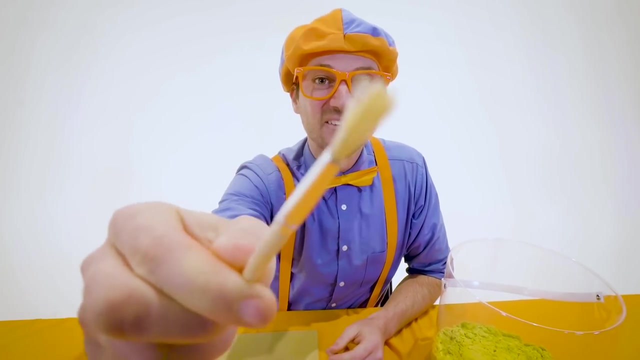 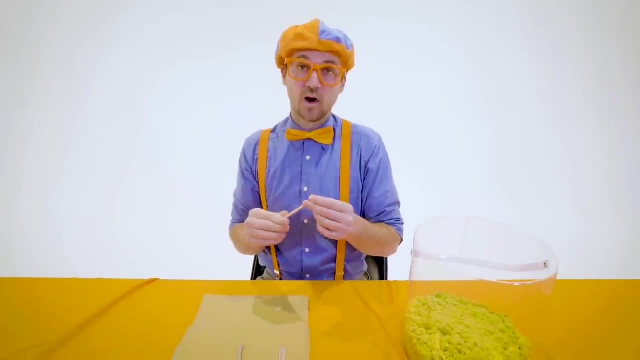 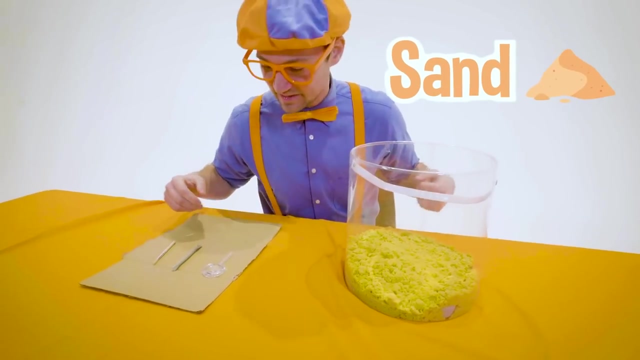 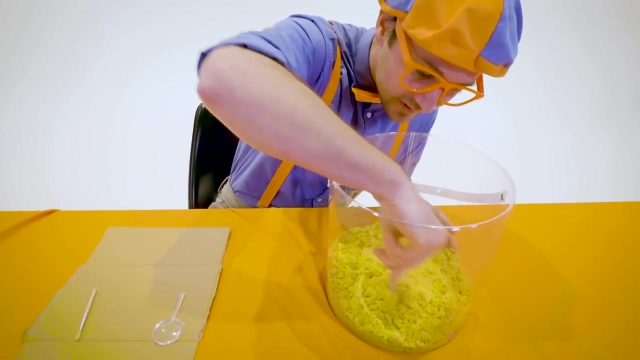 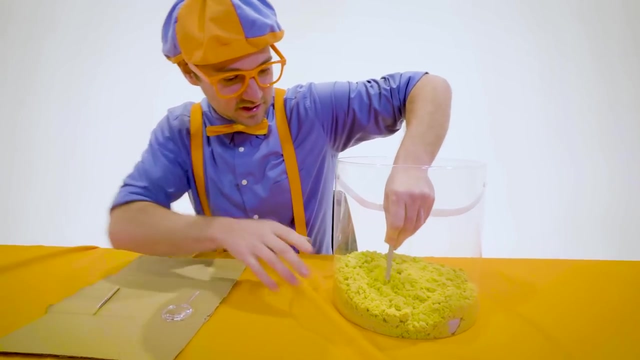 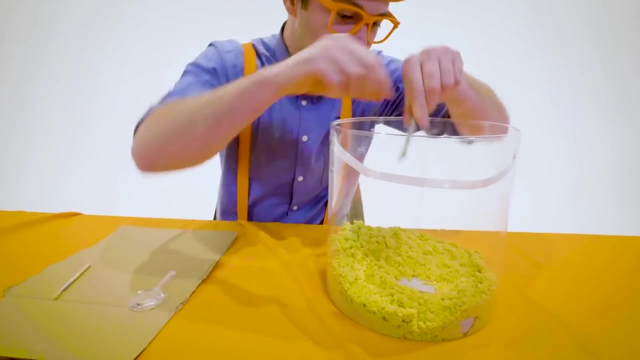 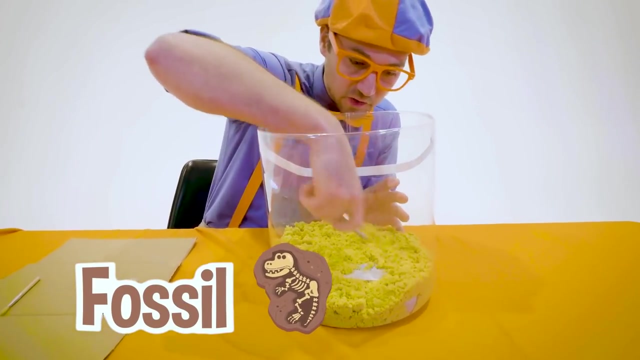 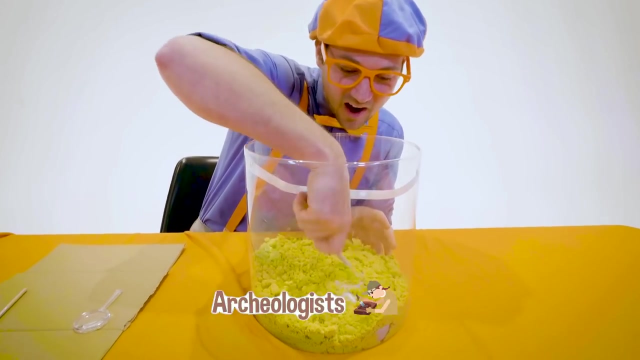 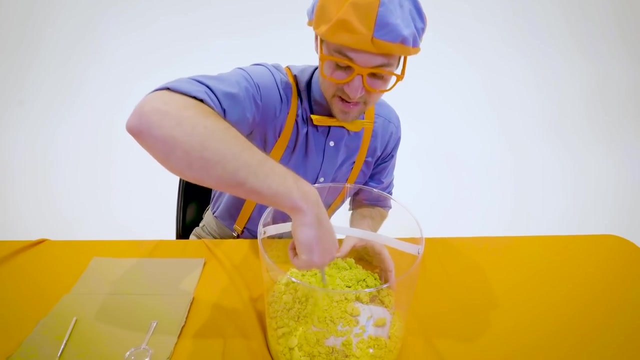 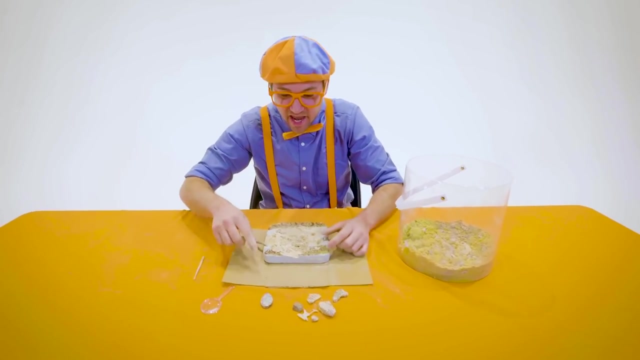 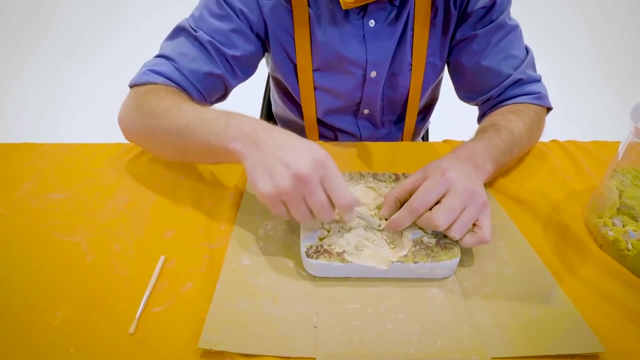 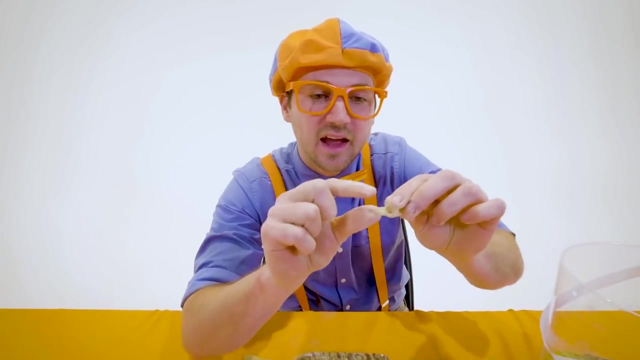 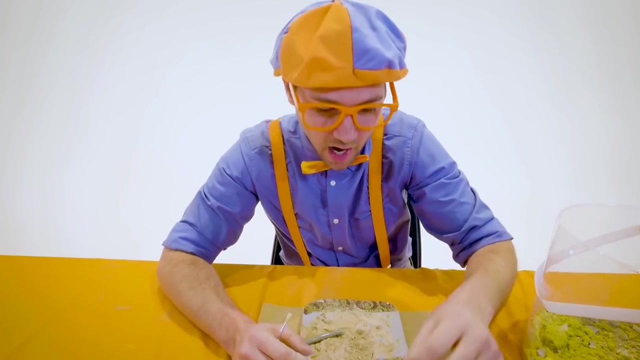 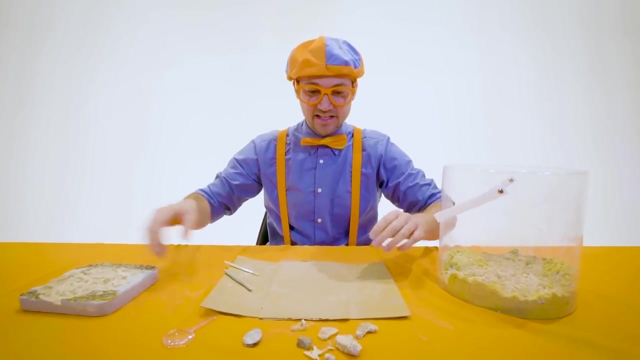 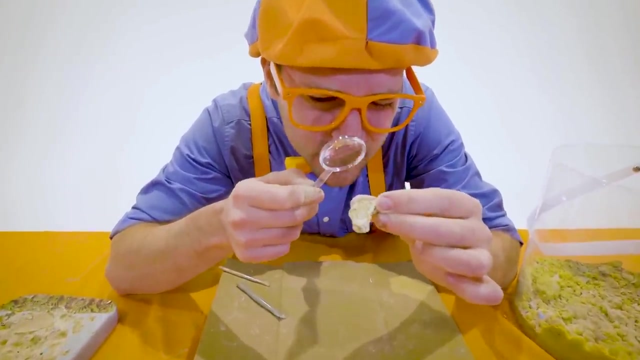 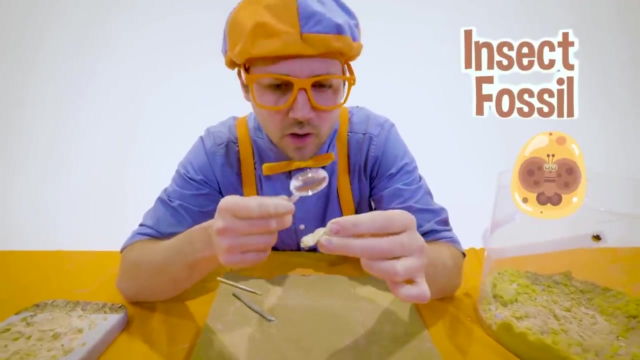 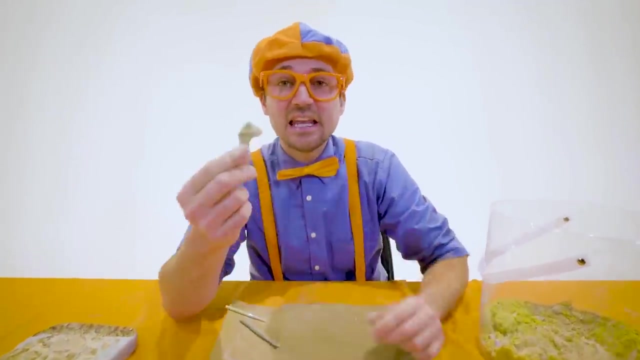 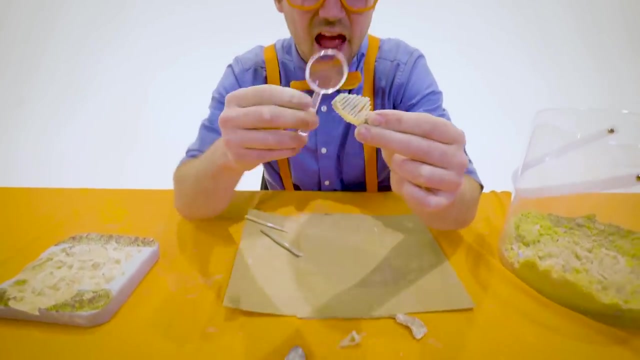 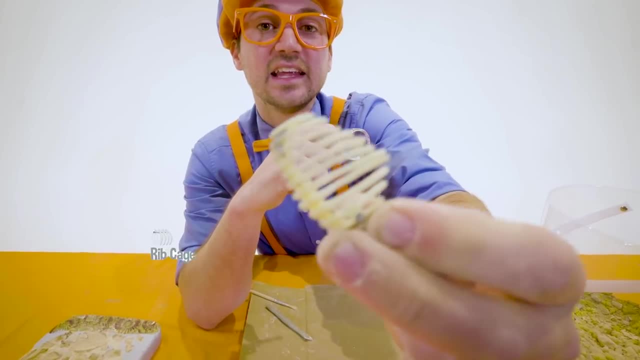 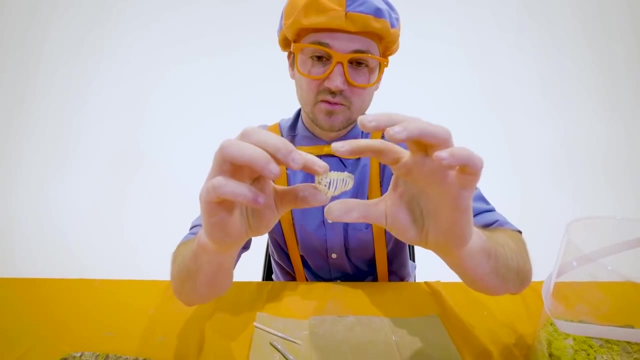 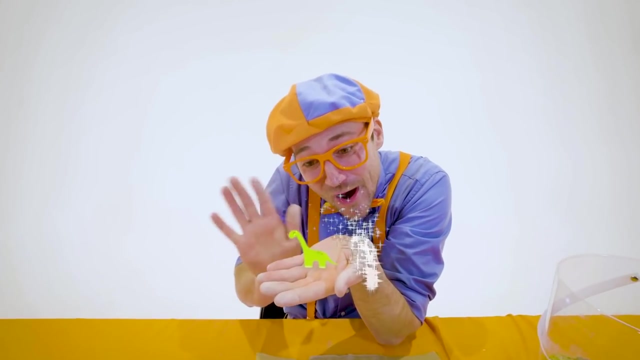 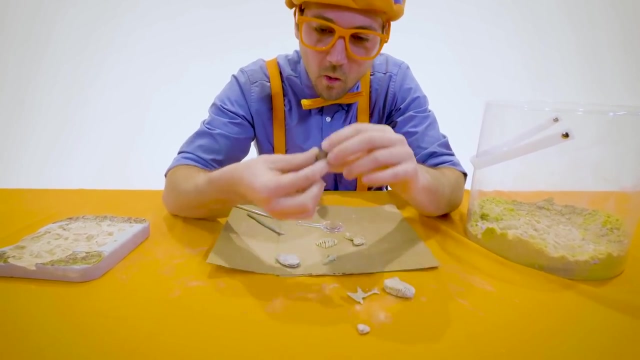 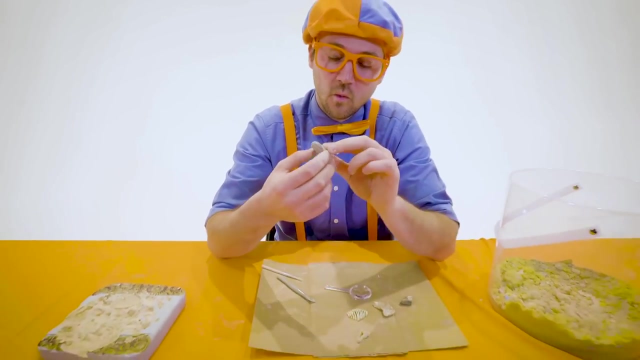 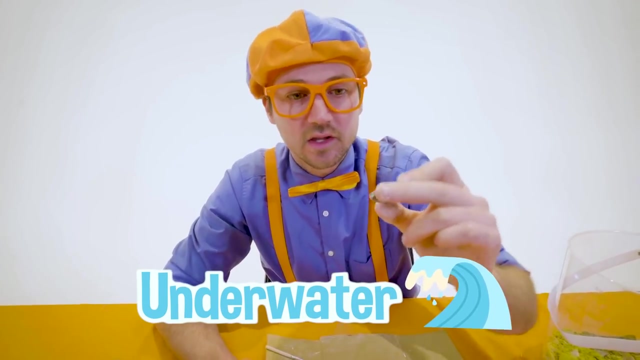 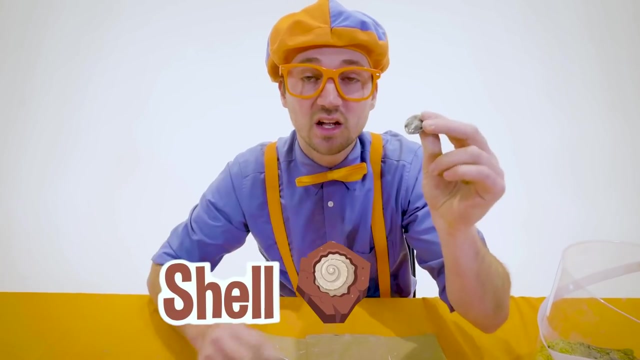 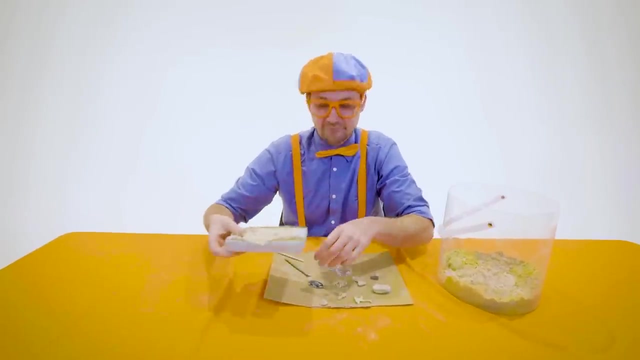 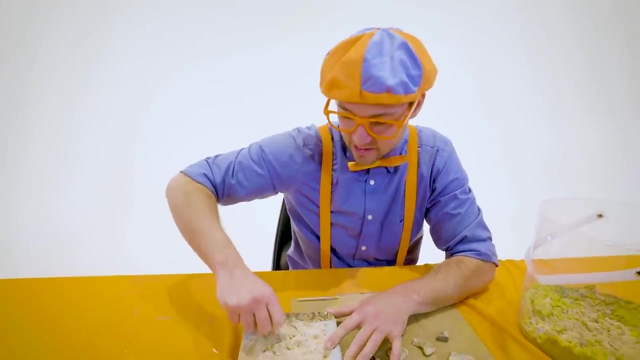 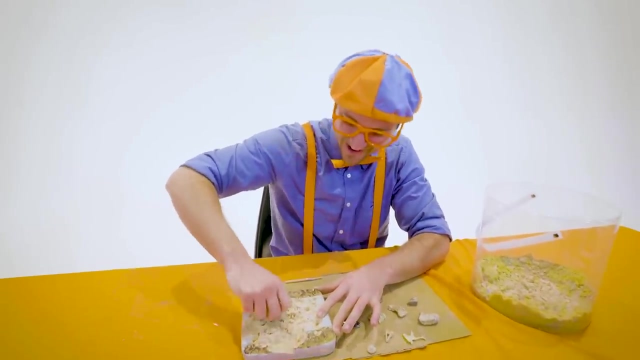 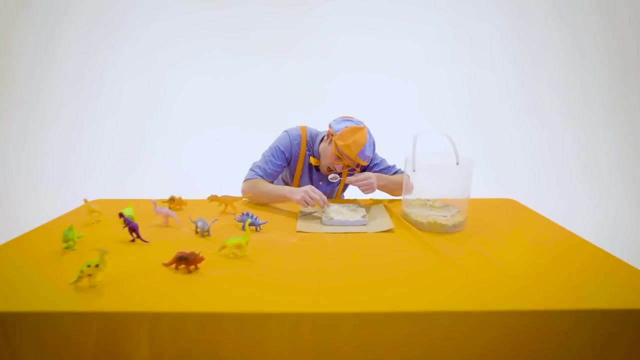 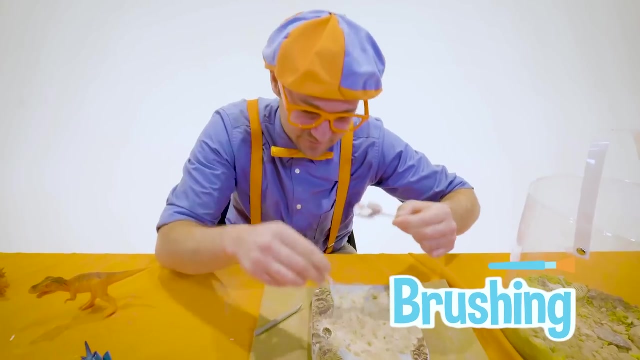 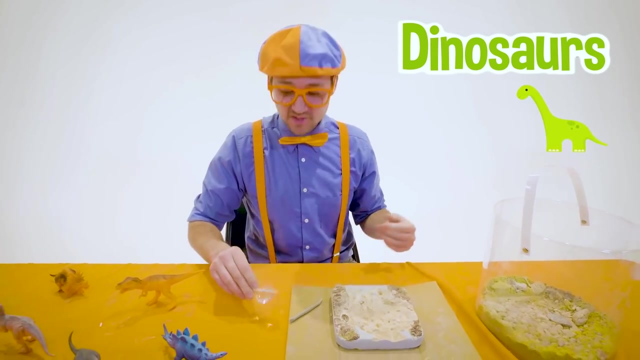 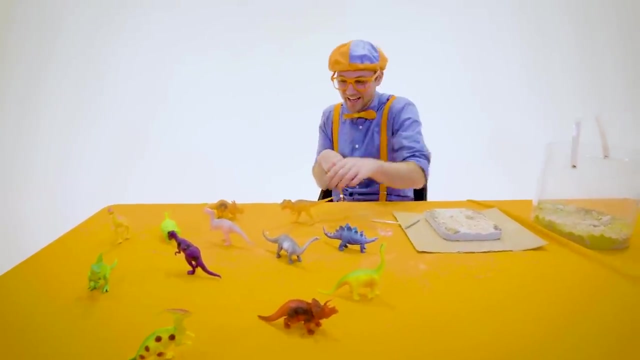 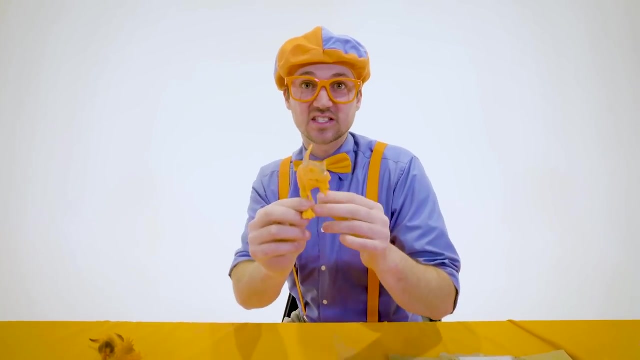 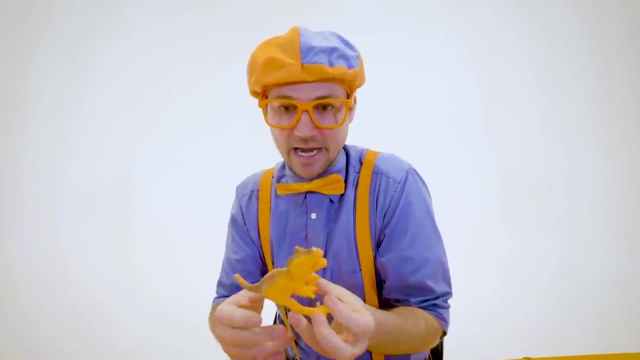 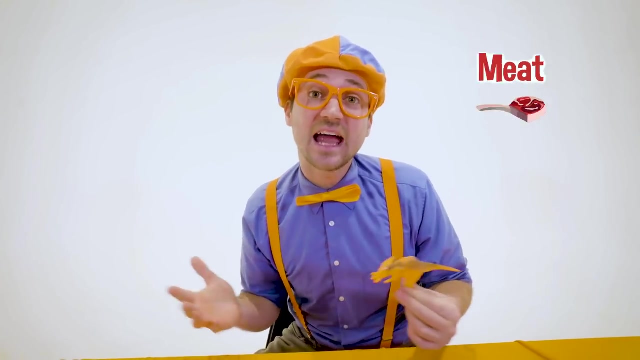 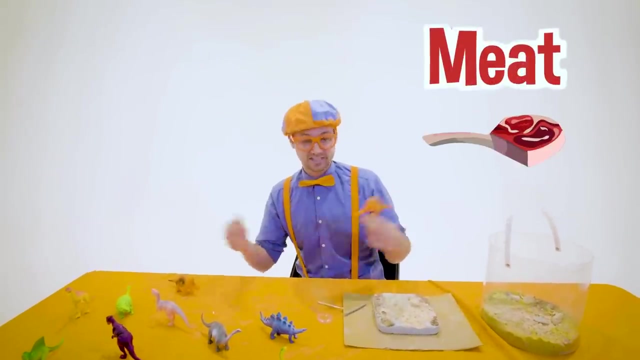 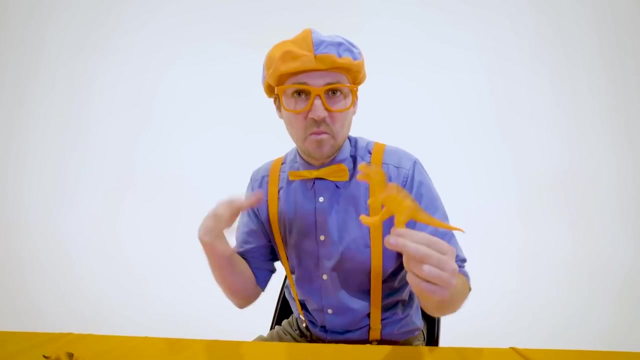 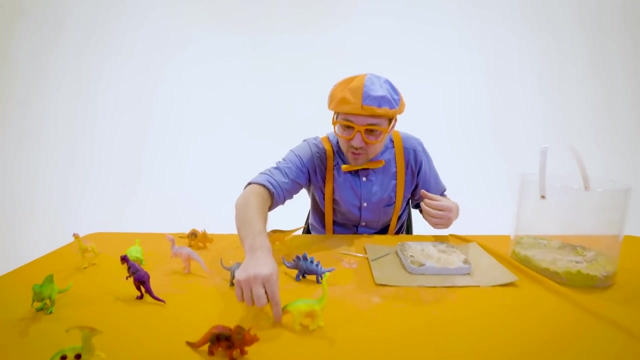 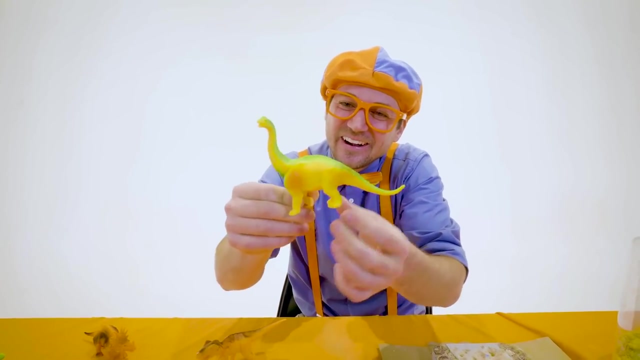 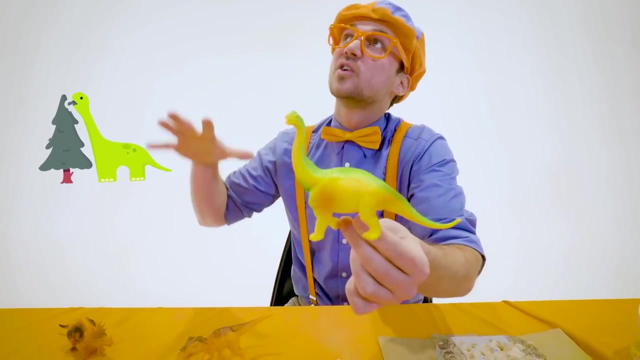 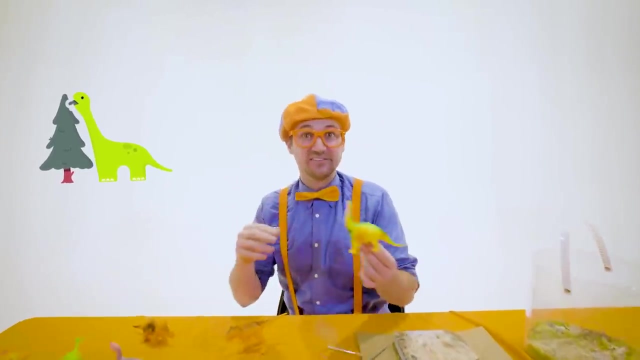 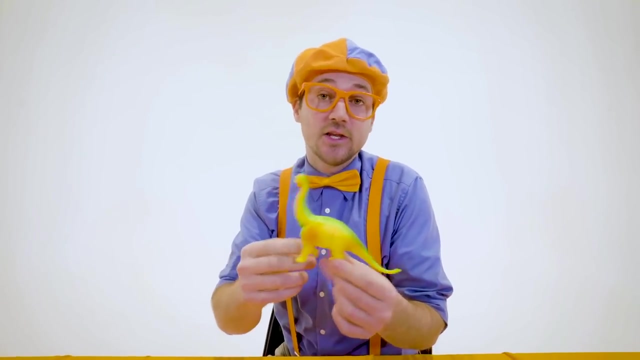 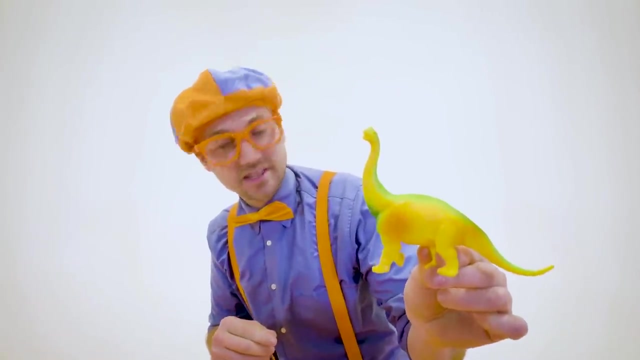 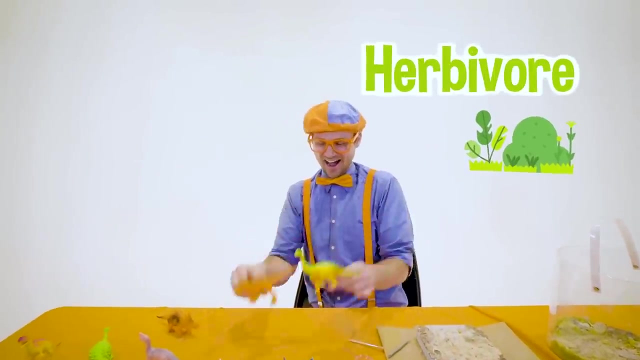 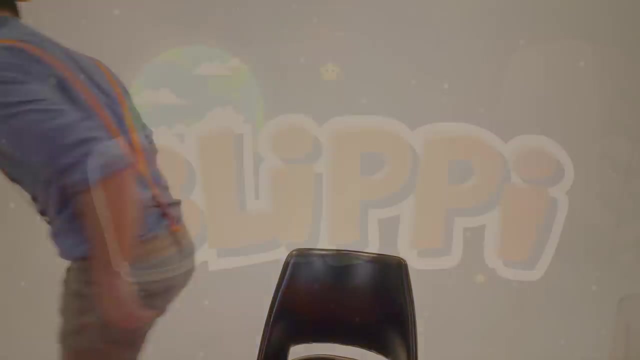 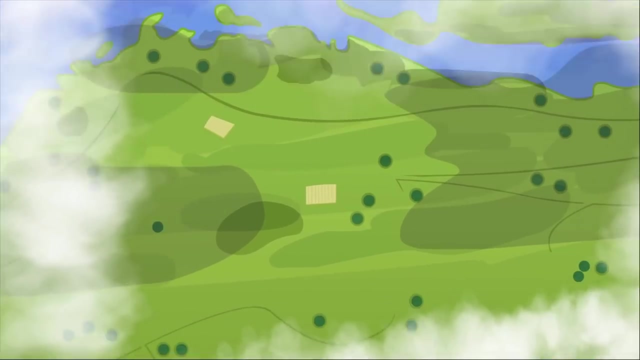 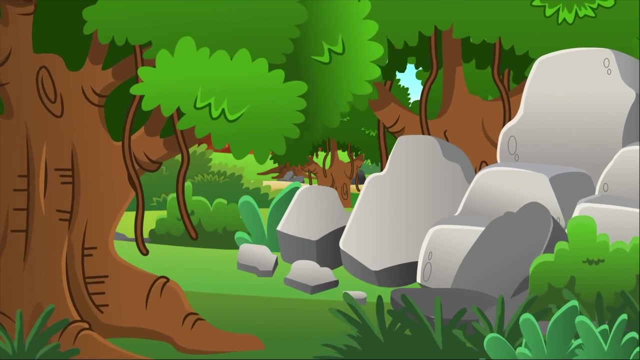 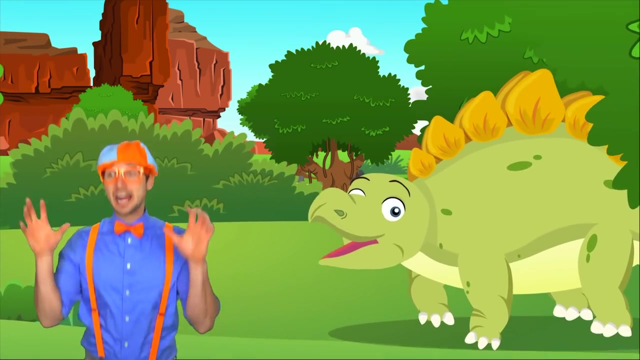 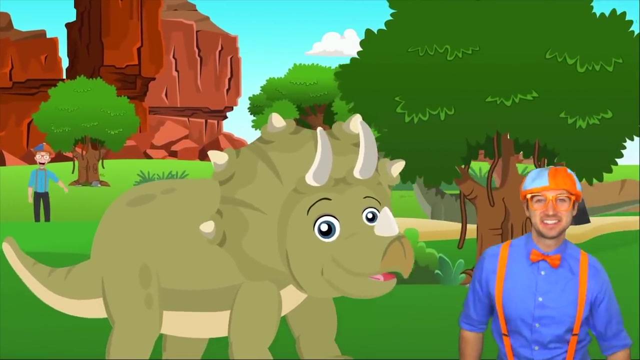 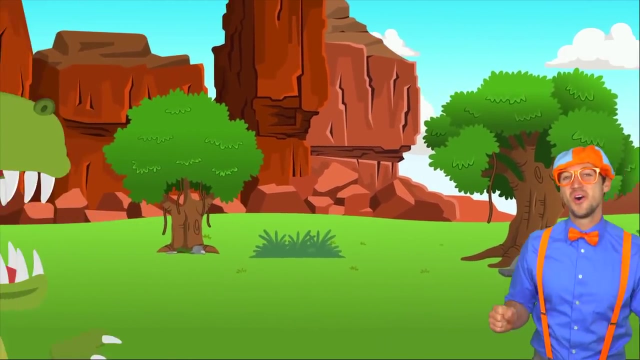 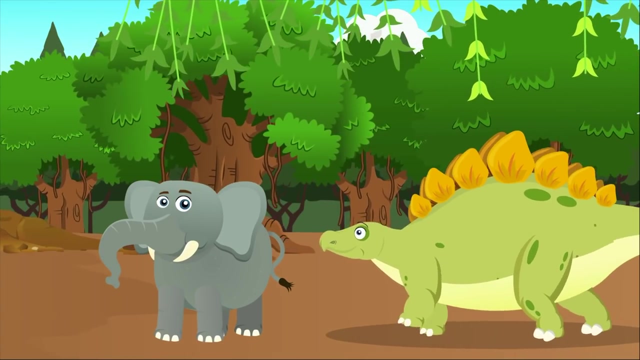 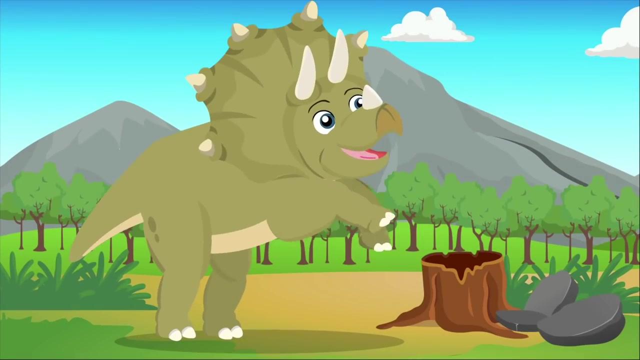 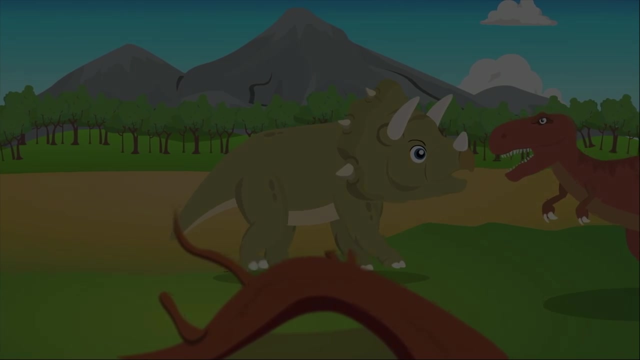 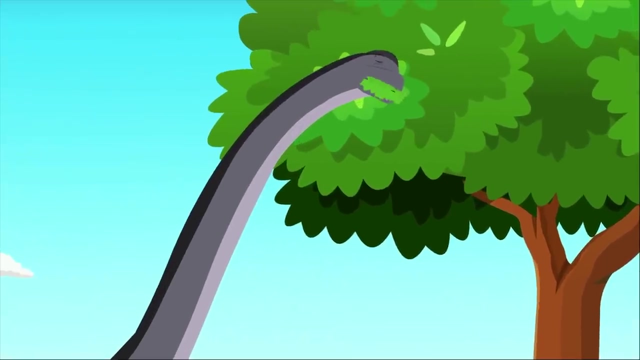 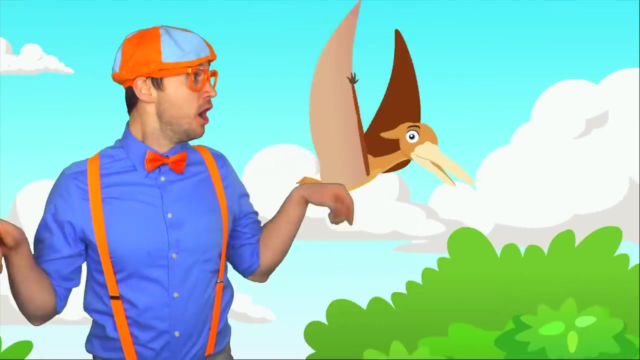 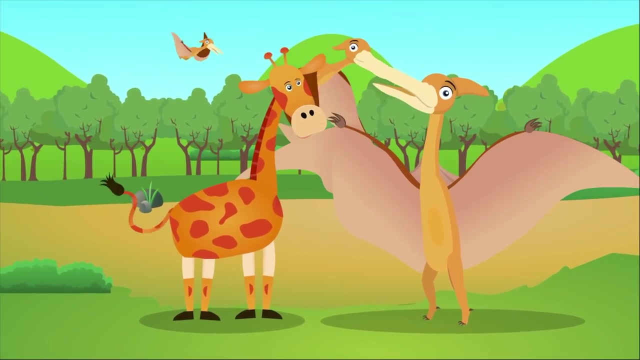 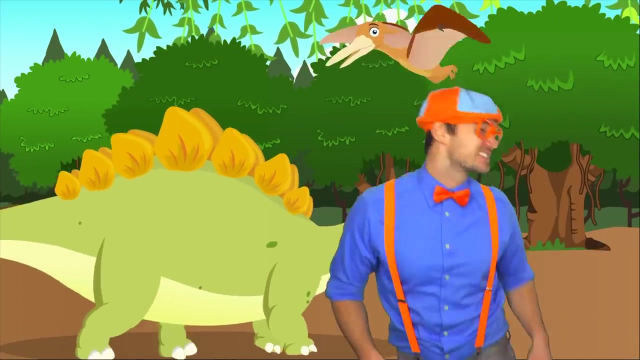 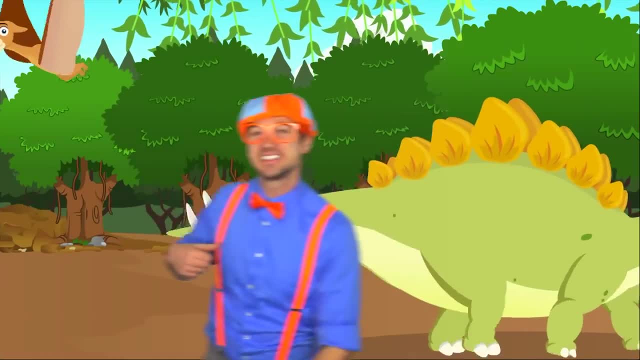 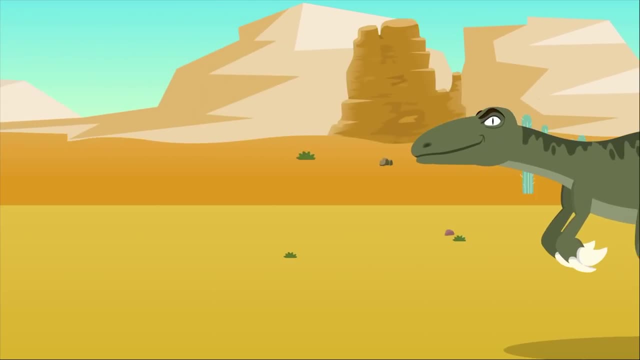 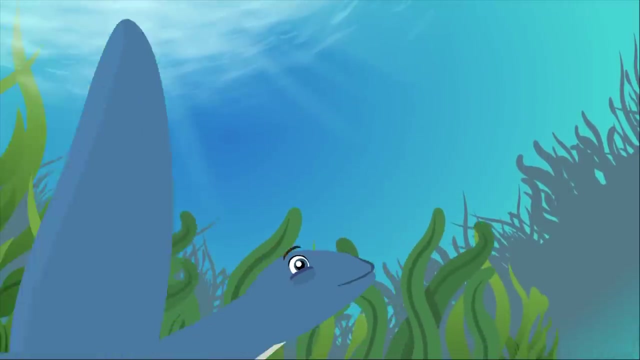 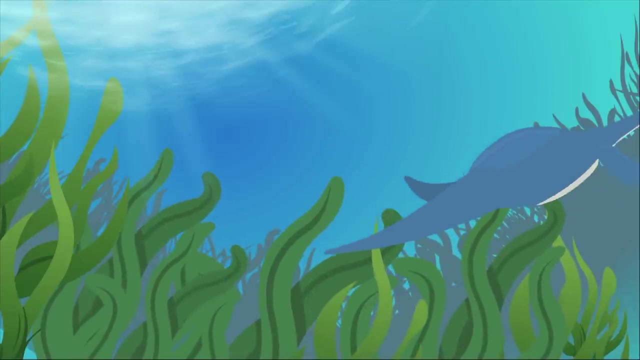 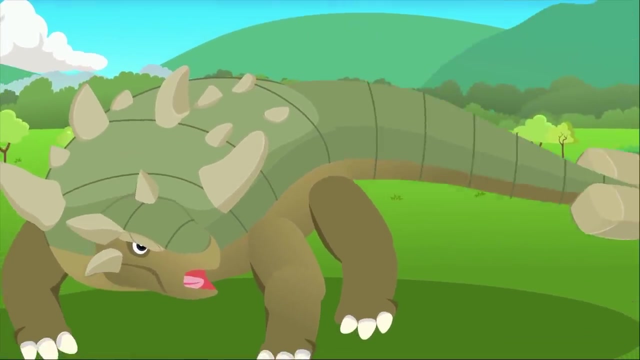 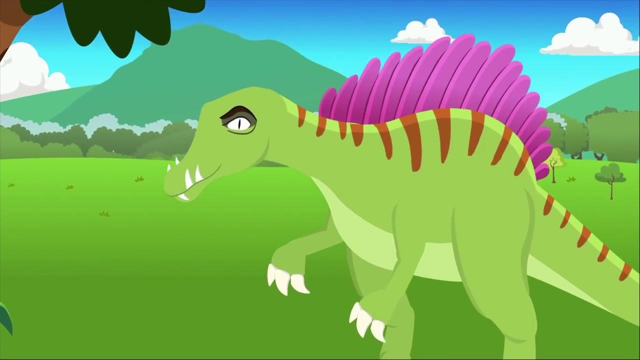 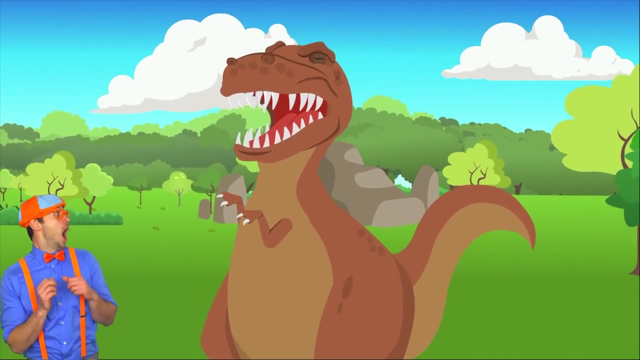 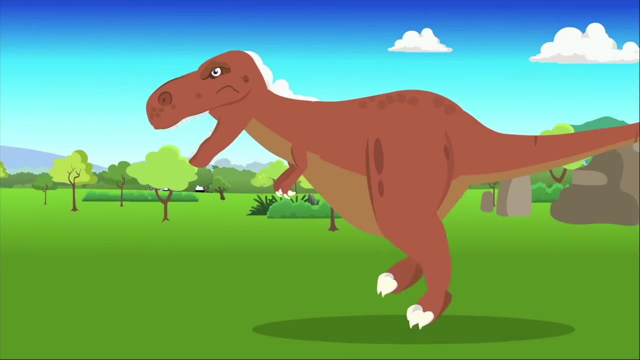 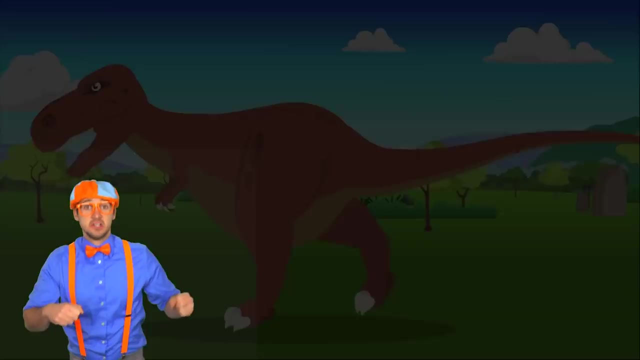 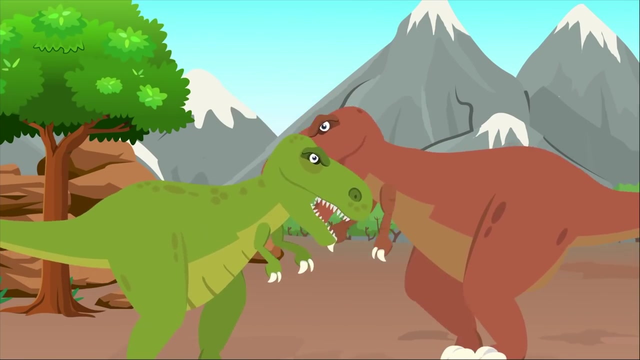 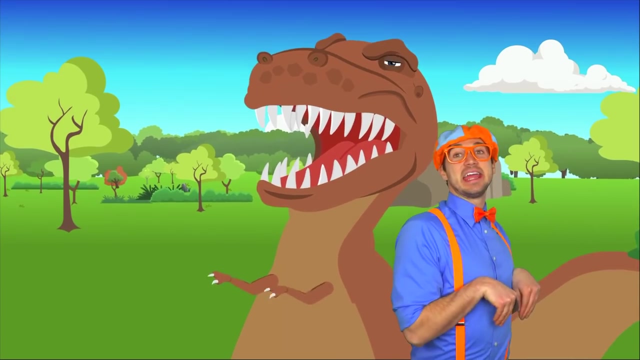 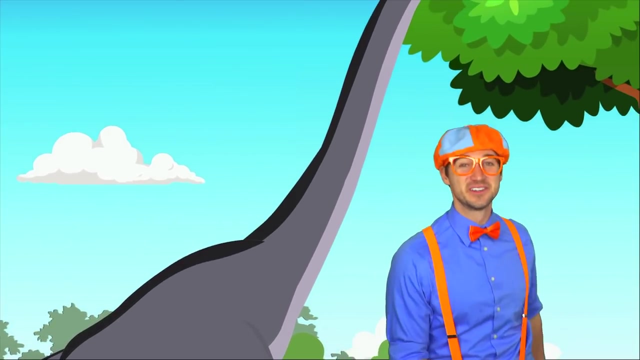 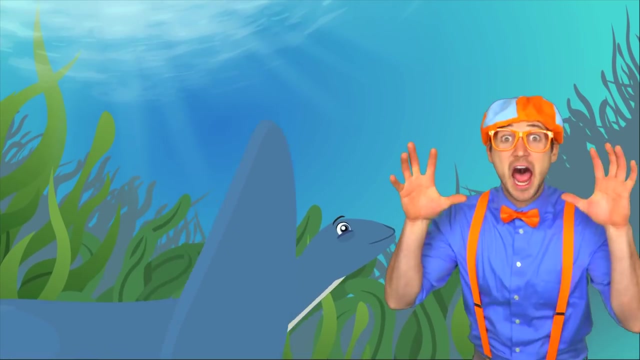 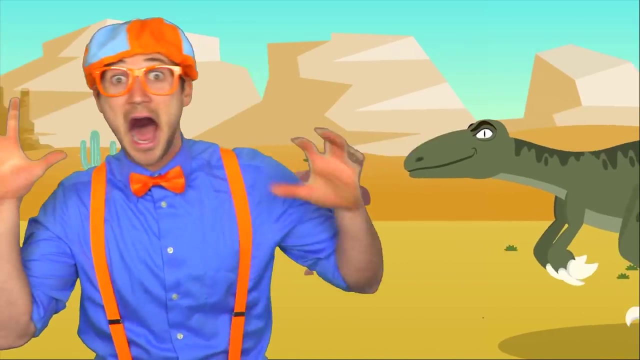 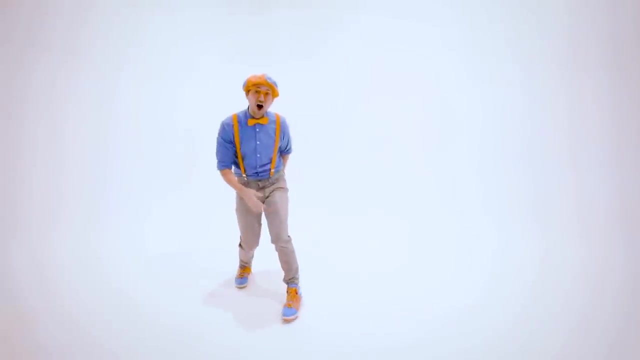 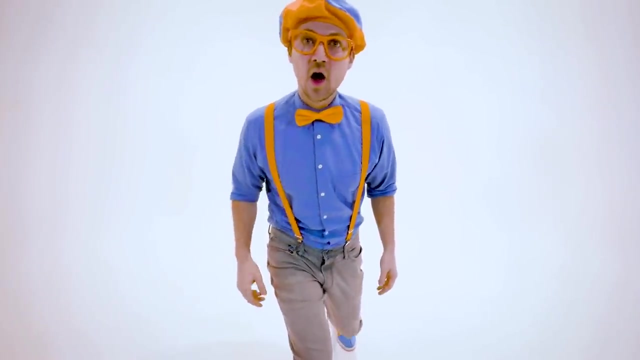 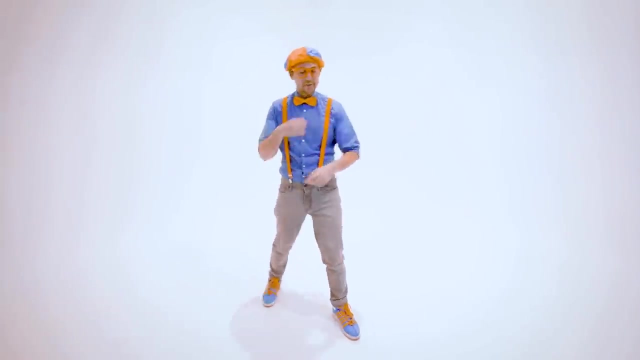 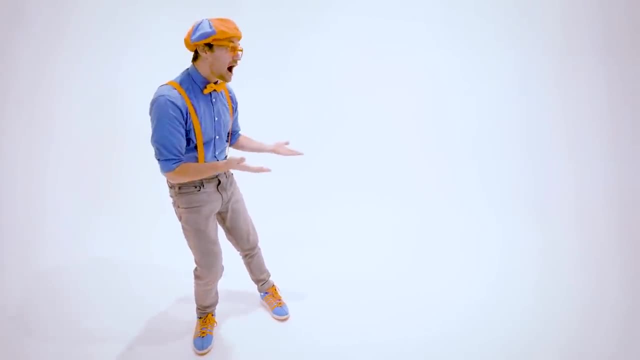 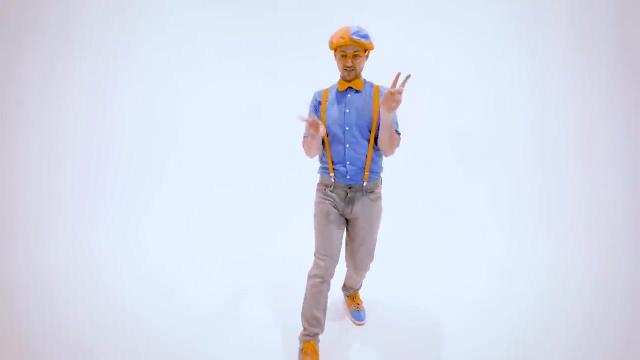 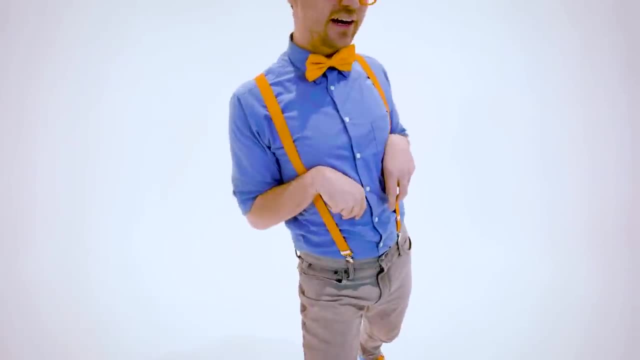 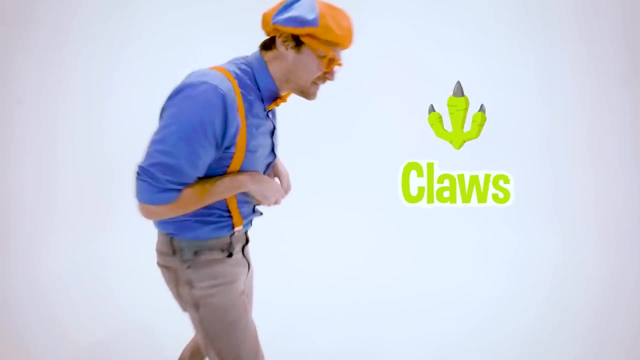 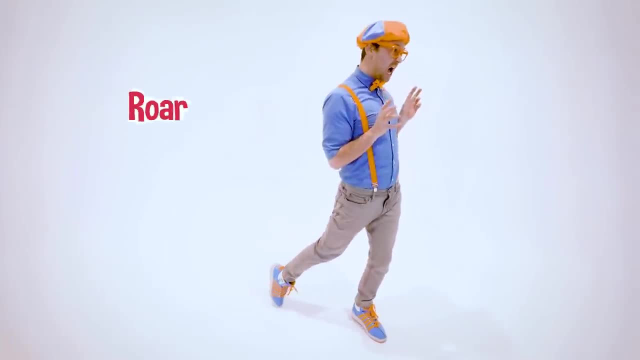 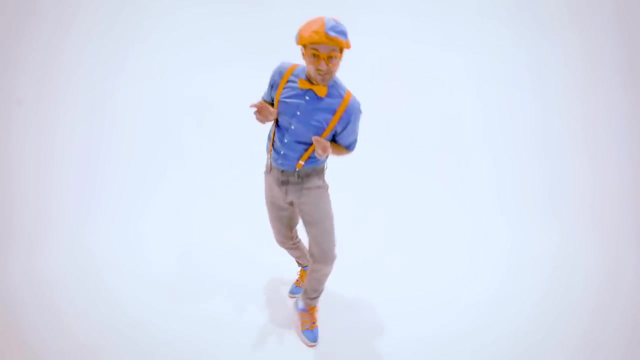 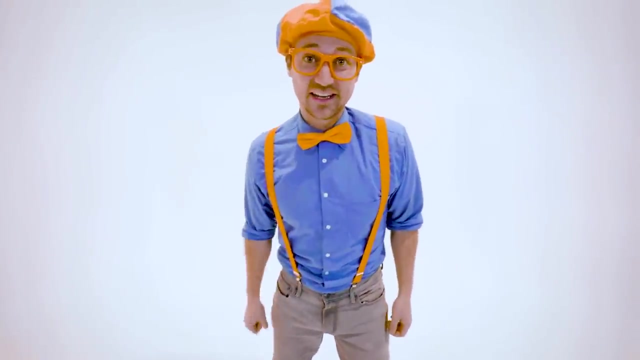 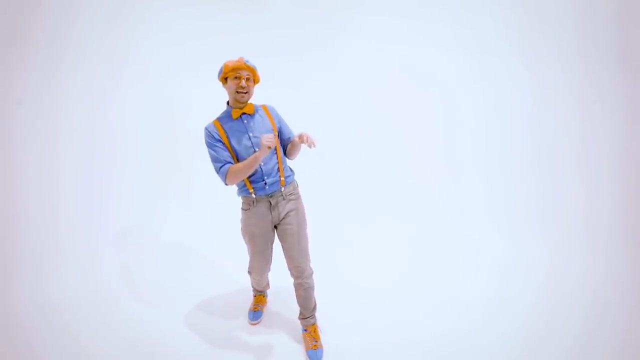 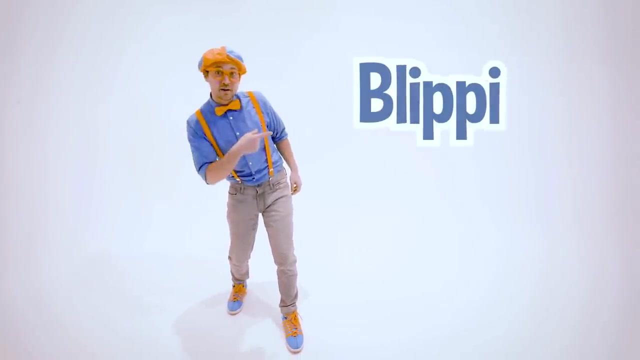 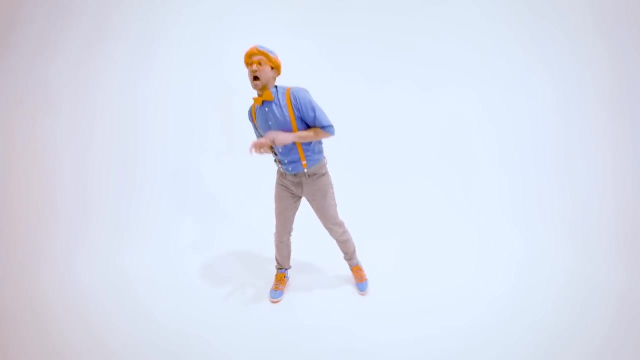 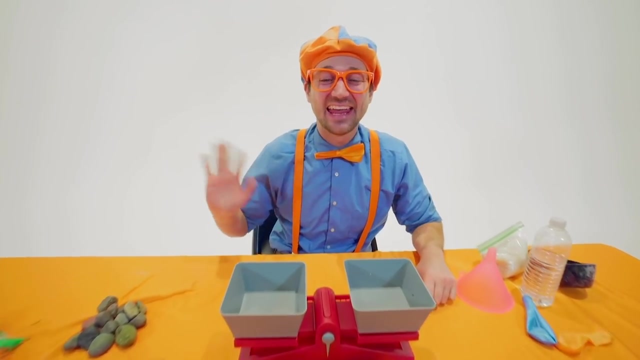 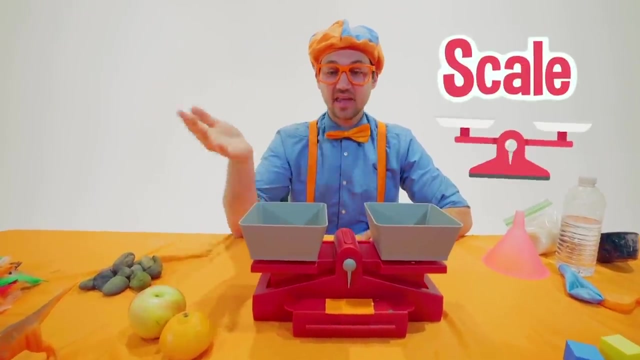 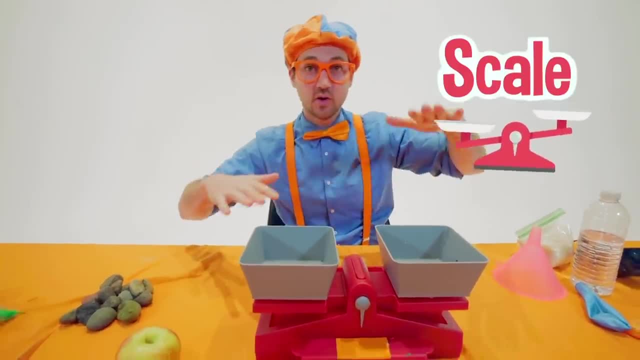 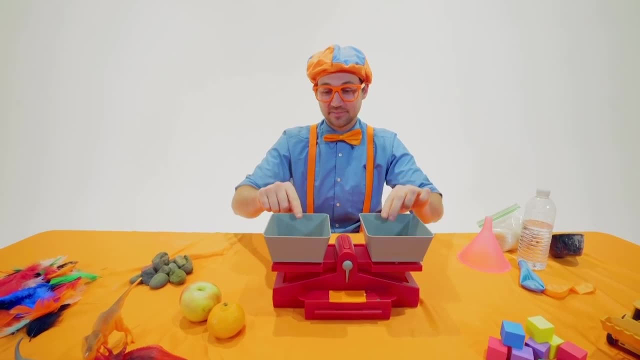 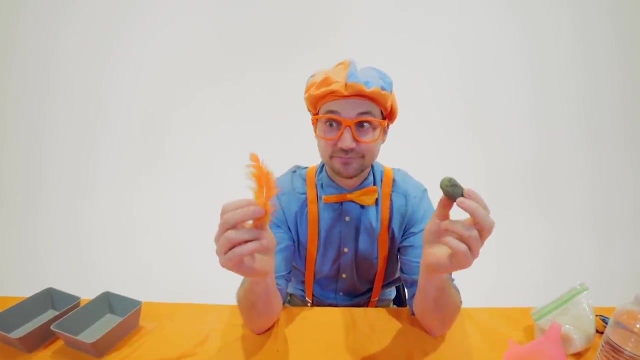 and whatever way it tips, will tell you what's heavier and what is lighter. Okay, let's try a really easy example. Okay, I'm going to take these. What do you think is heavier and what do you think is lighter- A feather or a rock? 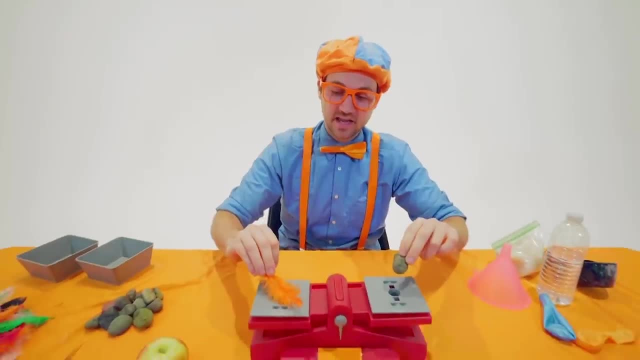 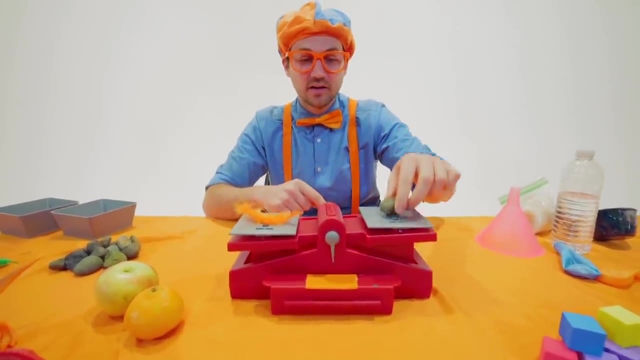 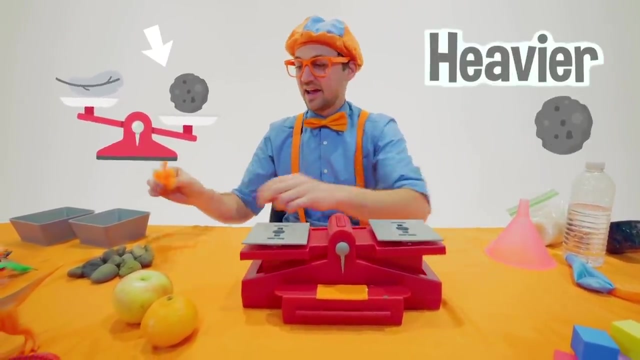 Yeah, I bet. Yeah, the rock is going to be heavier than the feather Ready. Yeah, Do you see how the rock is lower? Yeah, because this side is heavier. Okay, I have another idea. Yeah, How about a bunch of these feathers? 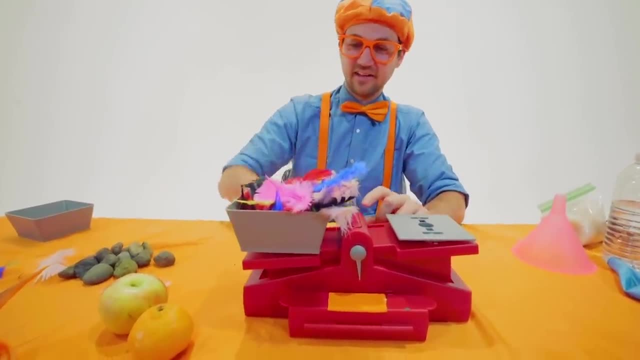 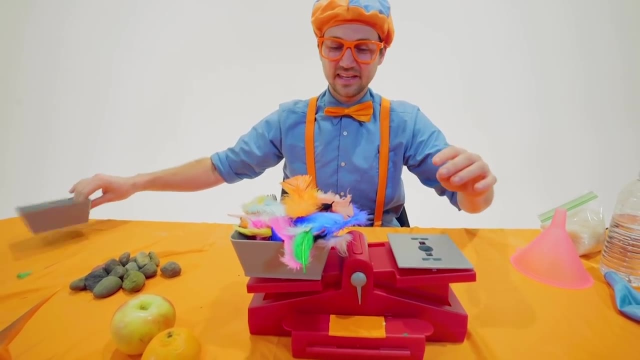 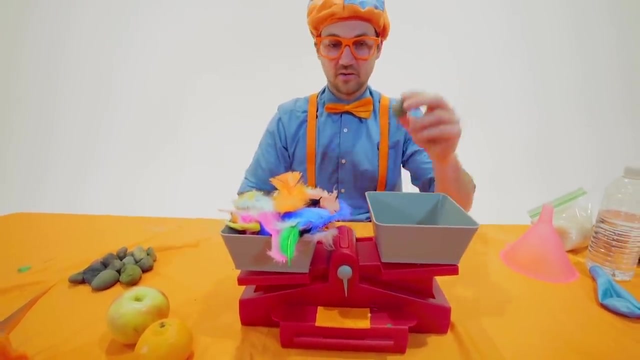 Whoa, Yeah, That's a lot of feathers, Whoa. and the feathers are so colorful And to make it even, we need to add the carrying case on this side too. Okay, now let's see if all these feathers weigh more or less than this rock. 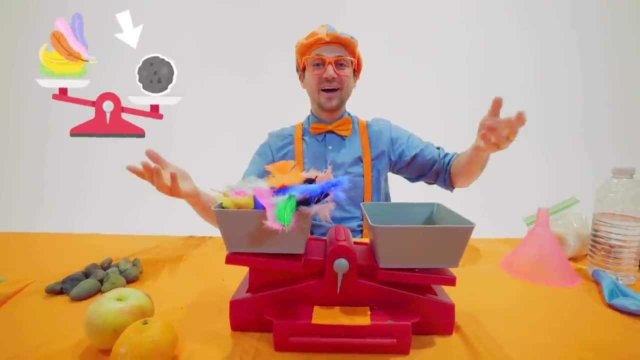 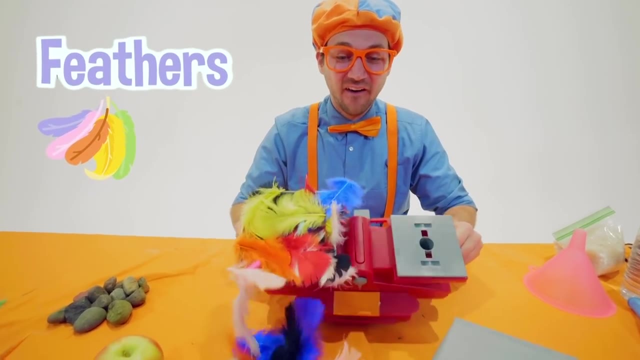 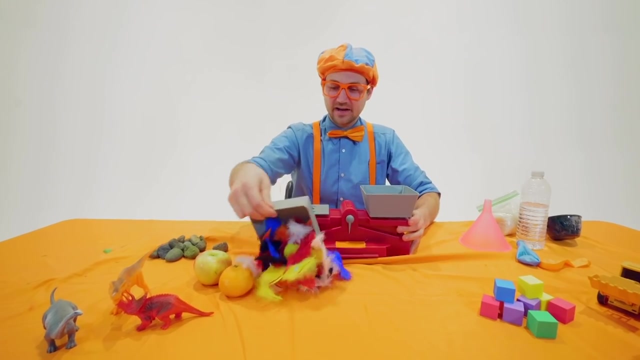 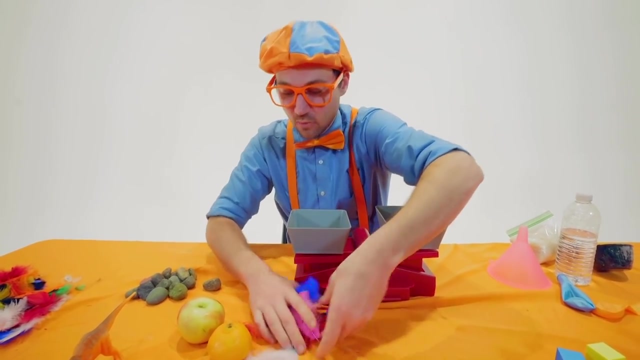 Ready. Oh, that one rock is heavier than all of these feathers. Whoa, Whoa. That is so cool. Okay, let me put that rock over there. Put this back up here. Wow, We have to stay nice and clean and organized because we have a lot of things to weigh here. 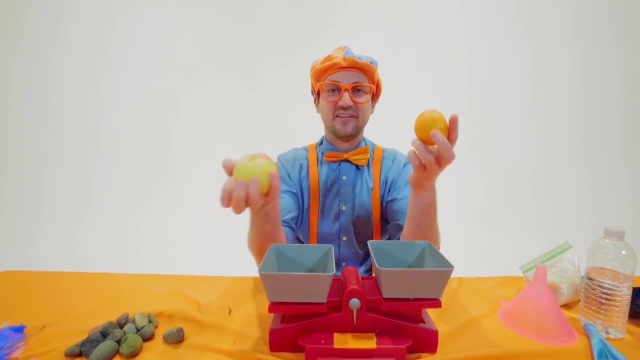 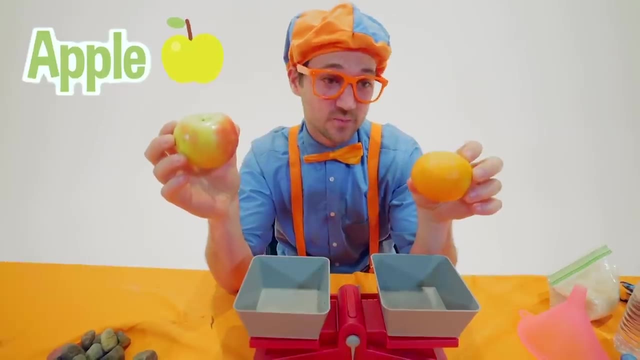 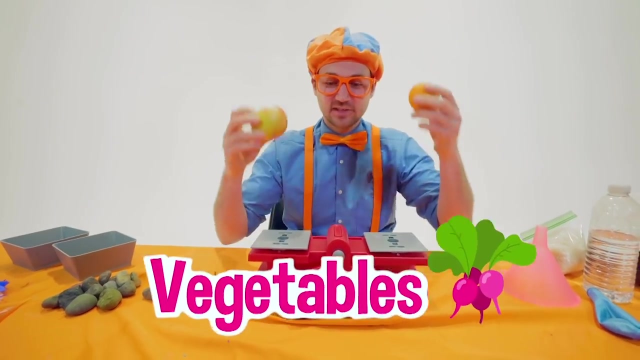 Hey, all right, Hey, check these out. What kind of fruit are these, Do you know? Yeah, This one is an apple And this one is an orange. Yum, Haha, I love fruit And I love vegetables. 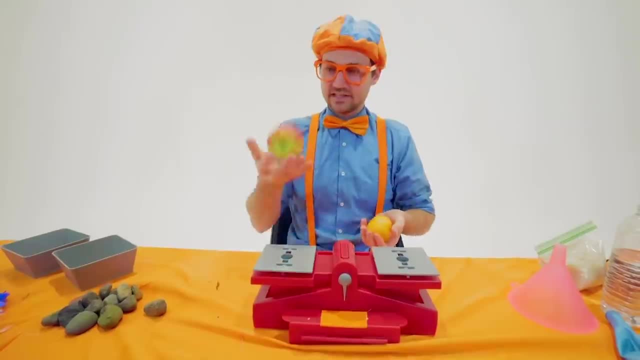 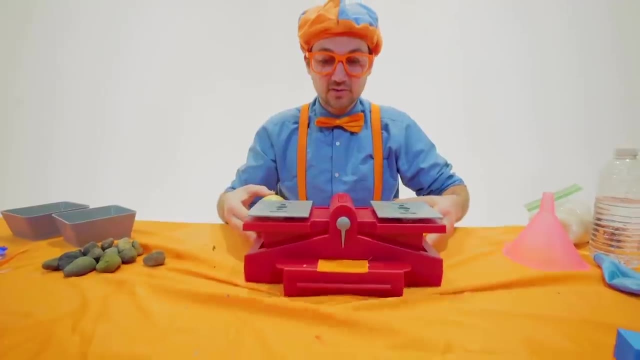 Okay, let's see. Huh, they weigh roughly the same. I wonder what one's going to be heavier and what one's going to be lighter. Ready Three, two, one, Whoa, Do you see that Yeah? 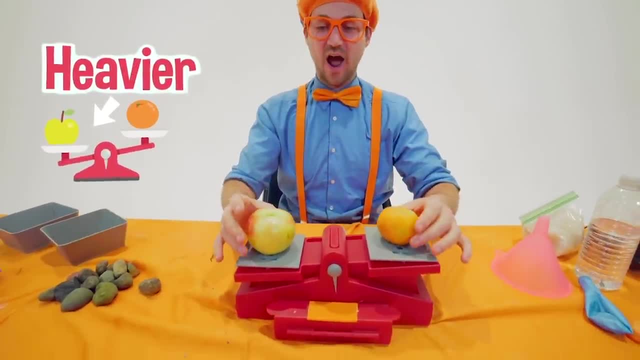 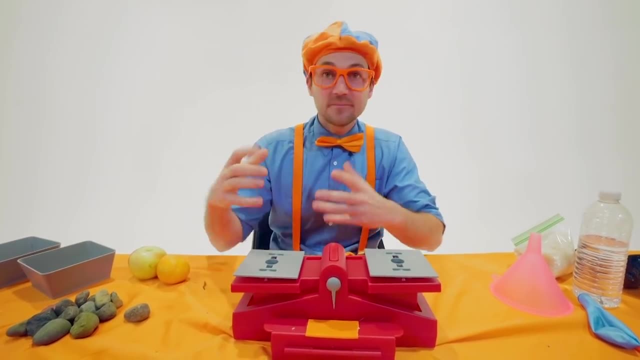 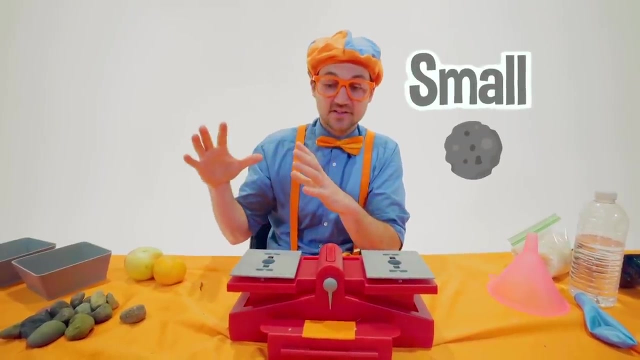 The apple is heavier, Wow, Haha, and it's bigger, But that isn't always the case. remember, Yeah, the feathers were so big And then the rock was so small, But the feathers, yeah, were lighter than the rock. 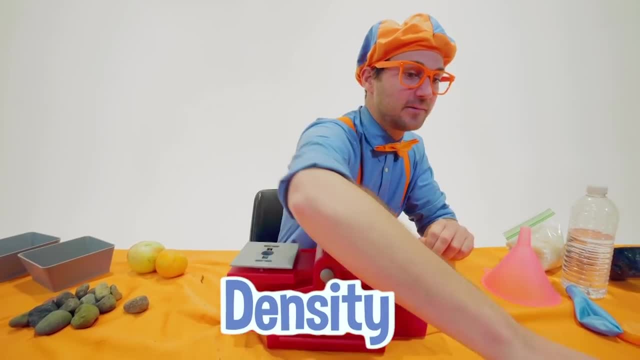 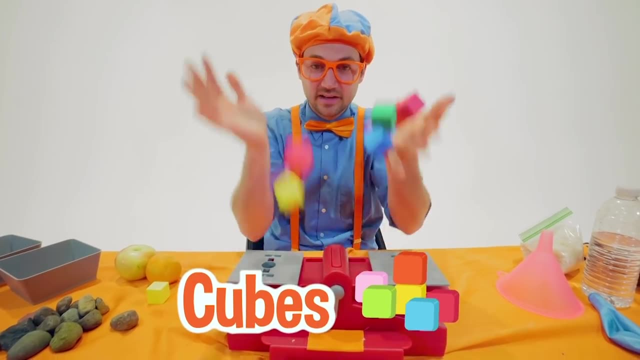 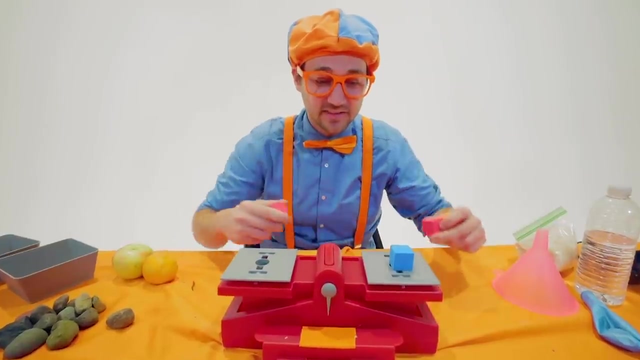 So it's all about density. Yeah, let's see here. Ooh, look at these. Haha, Wow, These are cubes And they actually are pretty whoa light. Haha, wow See, even one barely even tipped the scale. 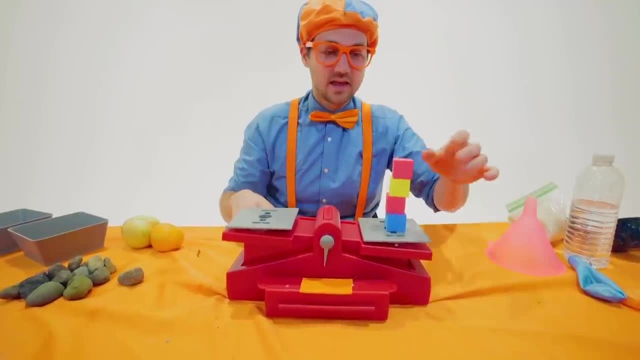 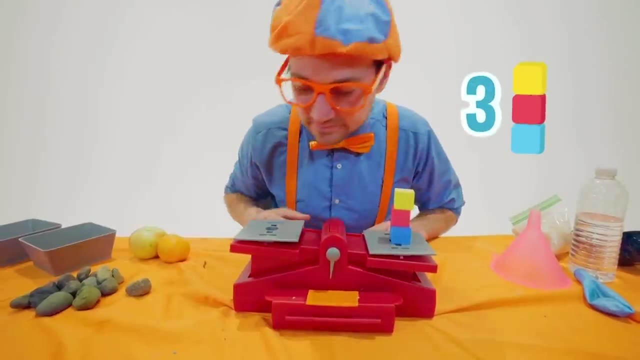 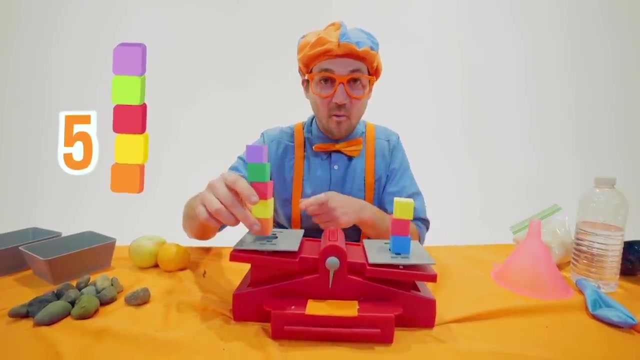 Okay. so let's go like this: Okay, there are four on that side. Actually, let's do three. Okay, now the same cubes on this side. Let's do five. What one do you think will be heavier? Yeah, you're right. 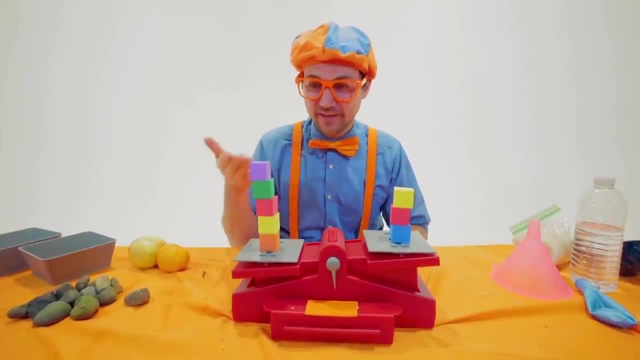 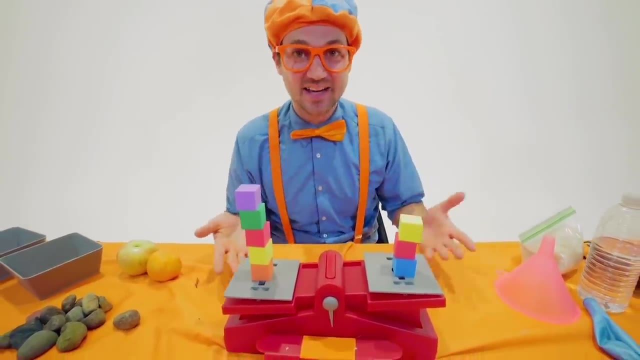 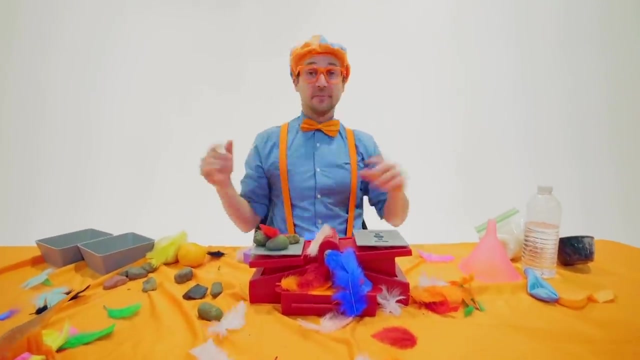 Five cubes of the same size and same weight is heavier than three cubes of the same size and weight. Haha, whoa, Okay, alright, let's get back to weighing things. Okay, let's put these rocks over here. Let's gather up all the feathers. 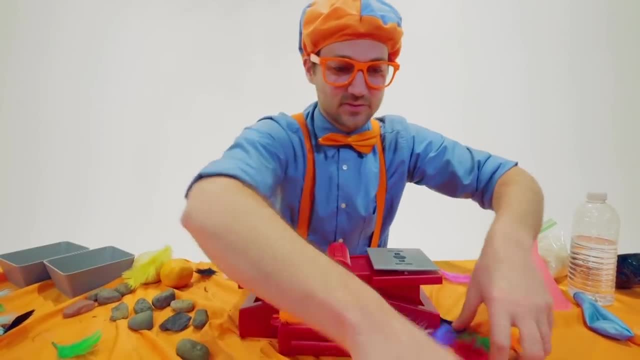 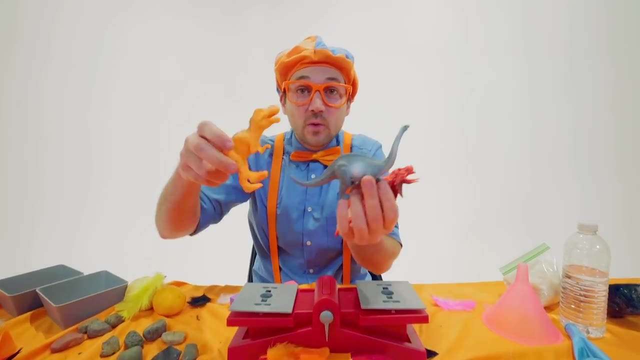 We need to pick up after ourselves. Alright, put those right over there, Haha, although they're so cute and pretty, Haha, okay, alright, Now we have some dinosaurs. Haha, whoa, We have a T-Rex. 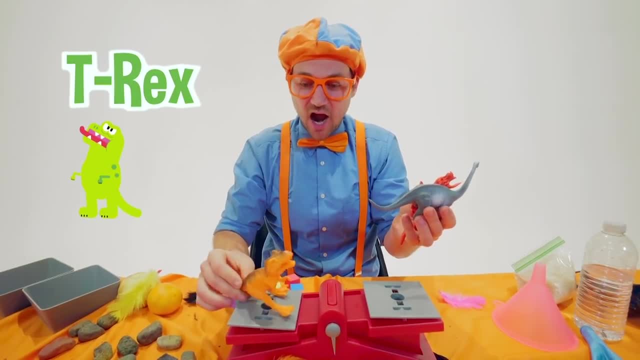 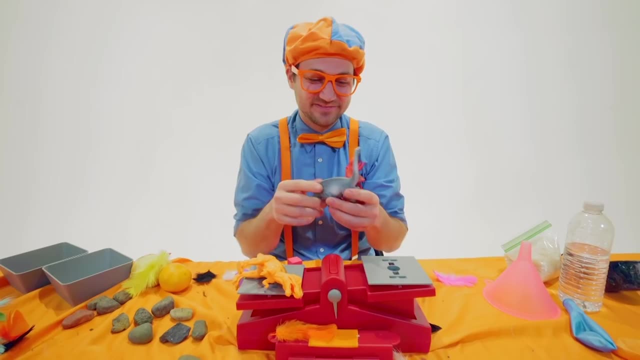 Okay, you can stand right there. How about you just take a nap, Just like that, Haha. and then we have a Triceratops. Haha, whoa, You're right. Haha, whoa, Whoa, whoa. 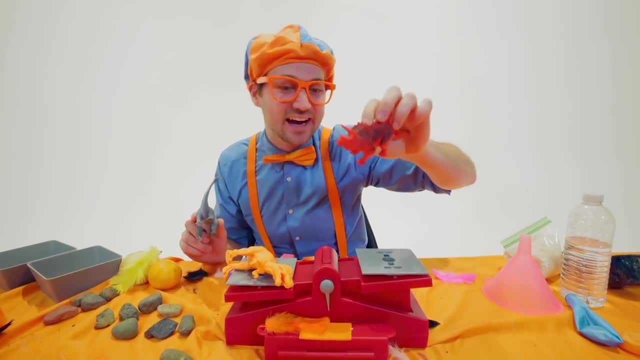 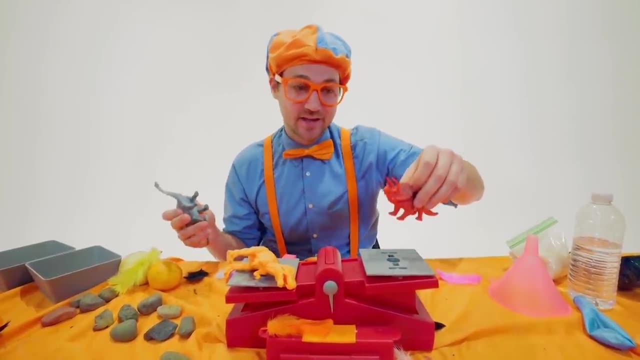 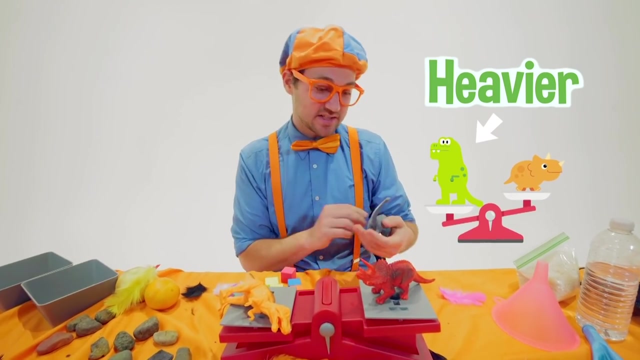 Haha, whoa. Okay, let's see what toy weighs more. I don't know the actual dinosaur weight, but just for these toys. yeah, this T-Rex is heavier than the Triceratops, But what if we added a Brontosaurus to it? 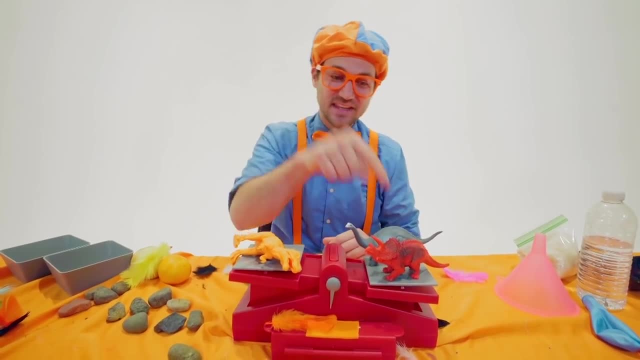 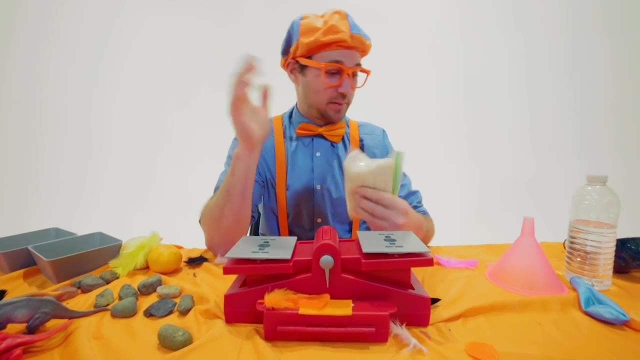 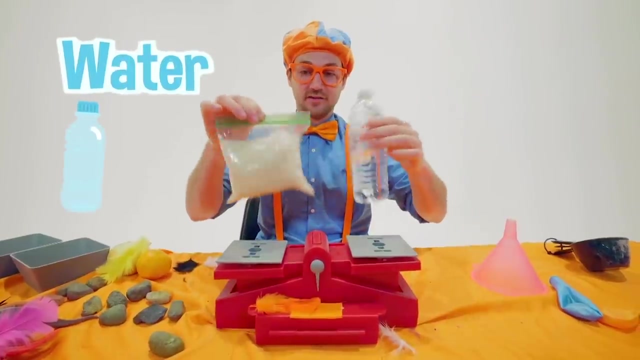 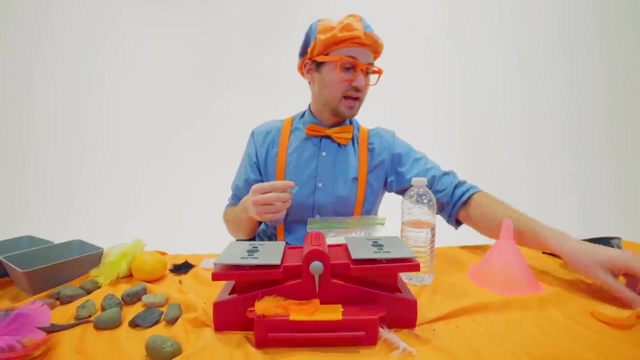 All right, are you ready? These are definitely heavier. Okay, we'll put those aside. All right, now we have an experiment. Okay, we have rice and we have water, So let's put the same amount of rice in a balloon compared to the water, the same amount. 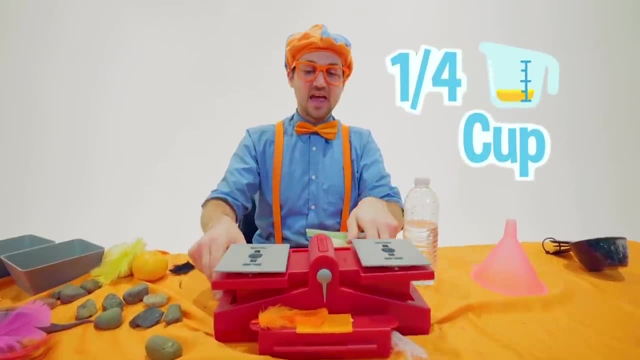 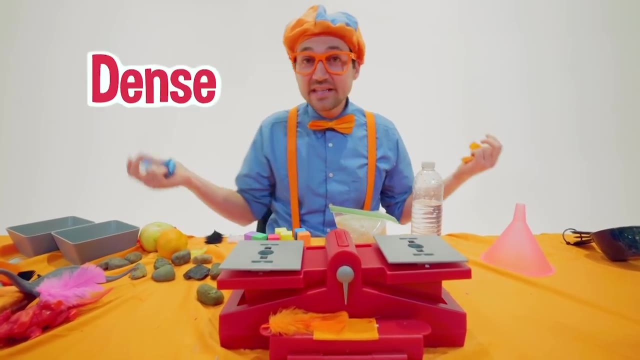 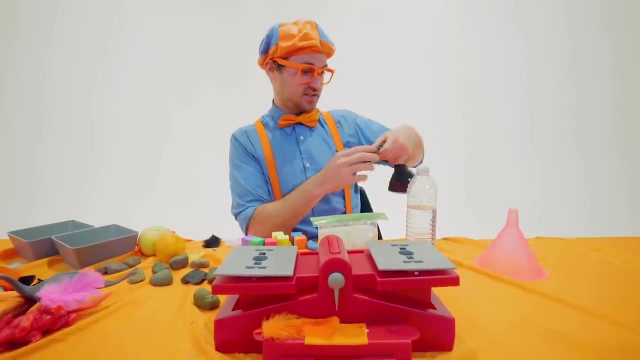 Let's do a quarter of a cup And then we can see what one is heavier, which means which one is more, And then we can see which one is more dense, because they're actually going to be roughly the no, they will be the same size. 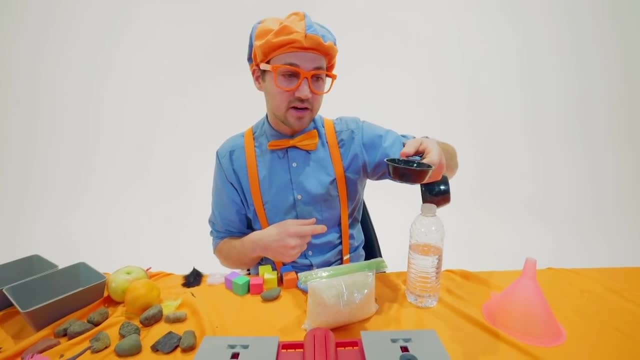 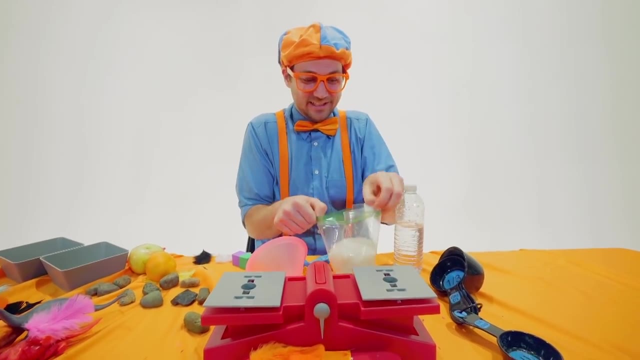 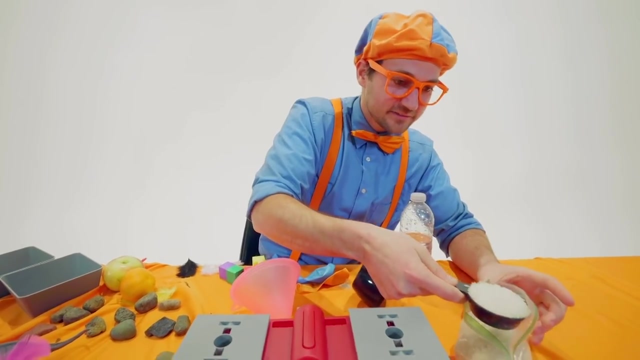 Yeah, because one quarter of a cup is volume. Perfect, All right. Sometimes it can be so confusing. Okay, all right, one quarter of a cup, Make sure it's nice And what? Perfect, Okay, Oh, got to set that down right here. 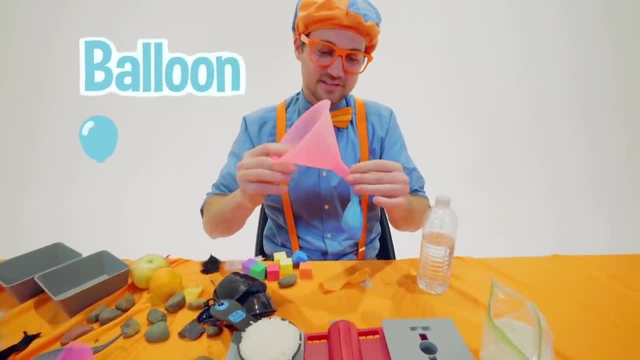 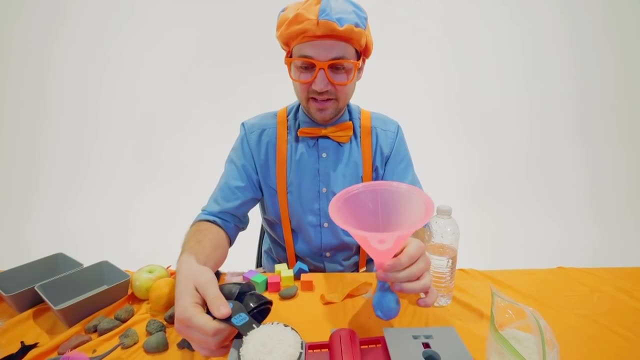 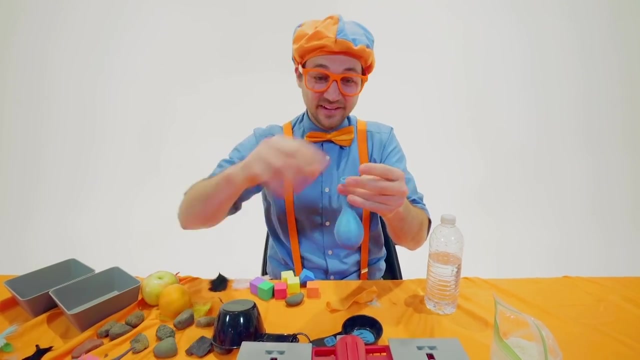 Need to prep my balloon first. Perfect, There we go. Okay, got to use the funnel or else it would be really dirty. Okay, here we go. One quarter cup. Let me tie it. Okay, now we'll do the water. 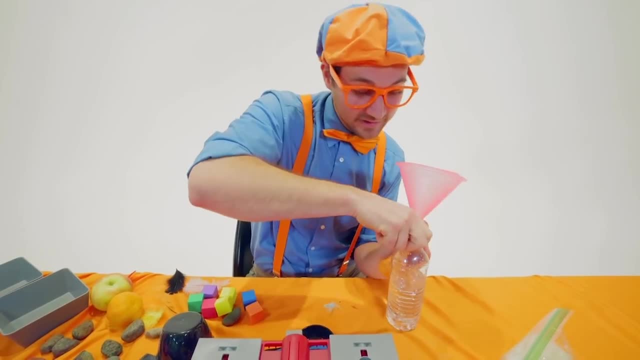 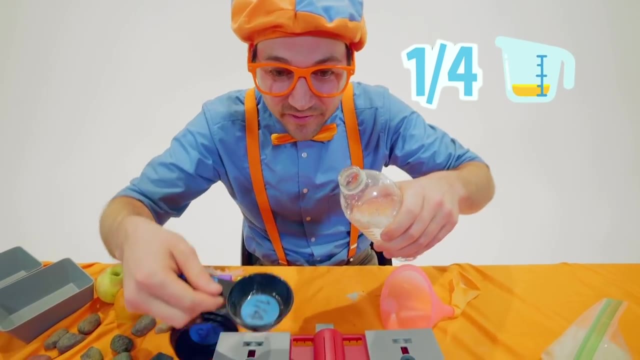 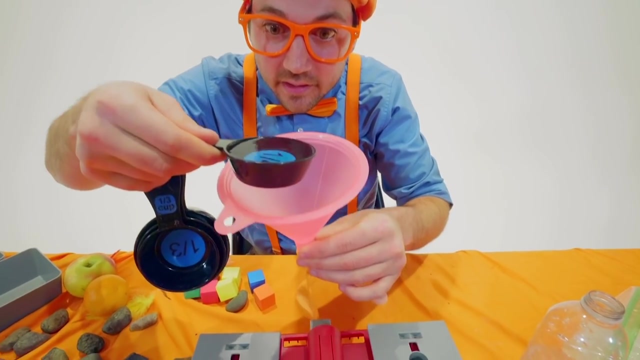 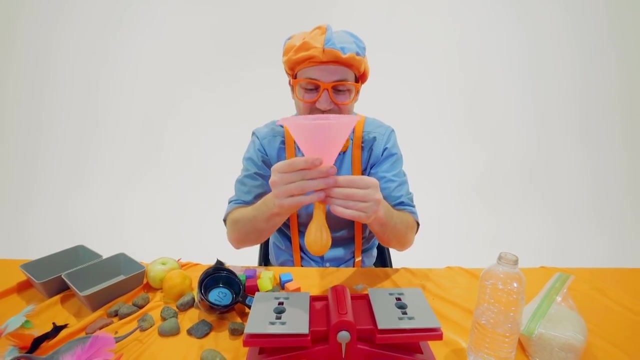 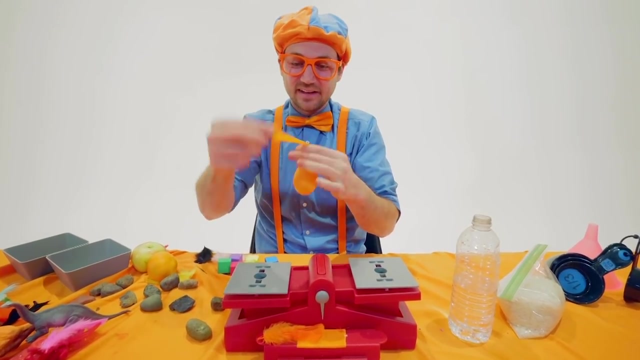 All right, Okay, now we need one quarter of a cup of water. Whoa, I don't want to spill Ready Ready. Ah, perfect, Okay, Stay nice and organized. Be sure to clean up. All right. now let me tie this. 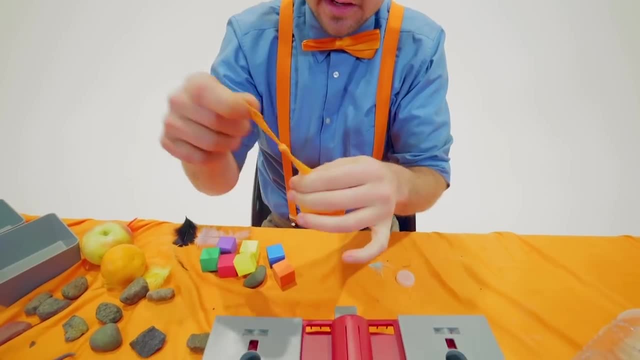 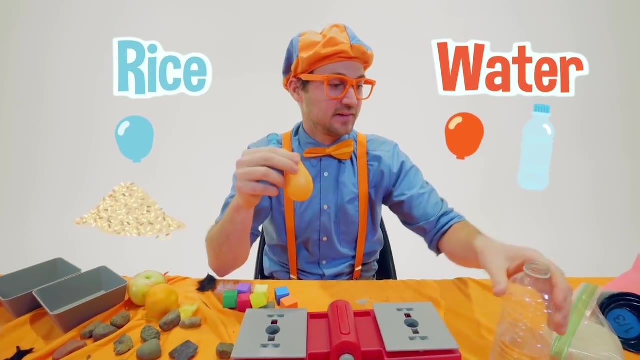 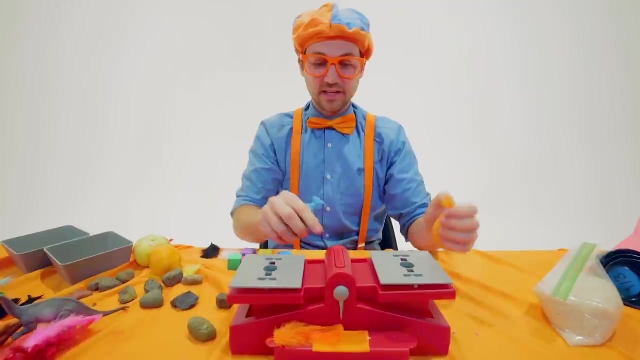 Okay, so we use the same amount of volume: one quarter cup of rice, one quarter cup of water. Okay, now we get to do the fun part. We get to put it on the scale and we get to see which one is more dense, which one is heavier. 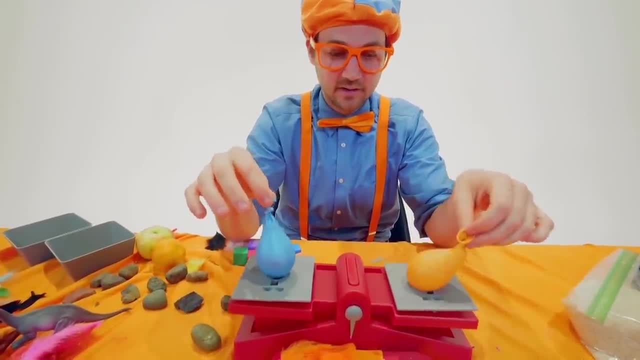 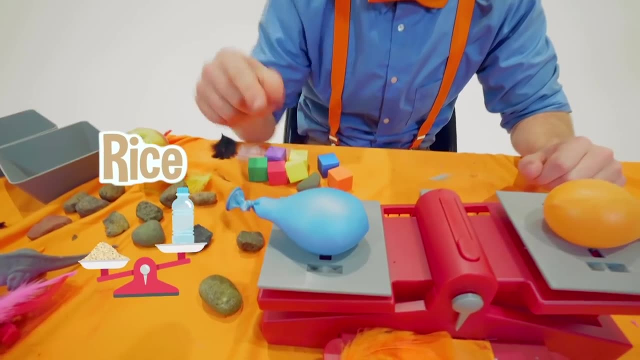 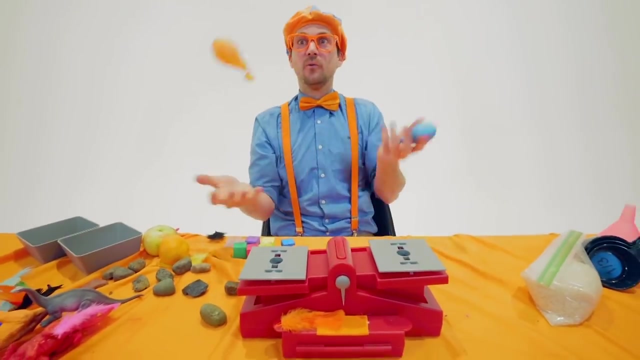 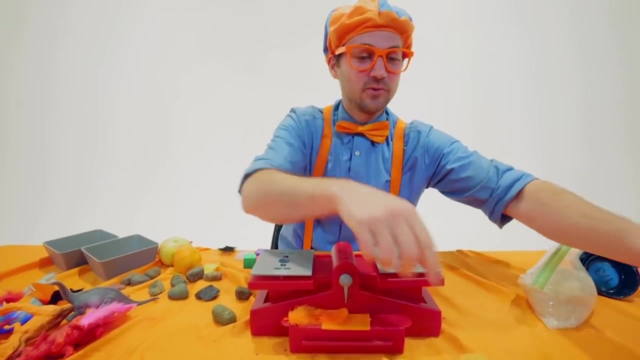 Ready? All right, here we go. All right, here we go. All right, here we go. Yeah, the blue was rice. Whoa rice is more dense than water. Wow, Hey, do you know what else is really heavy? 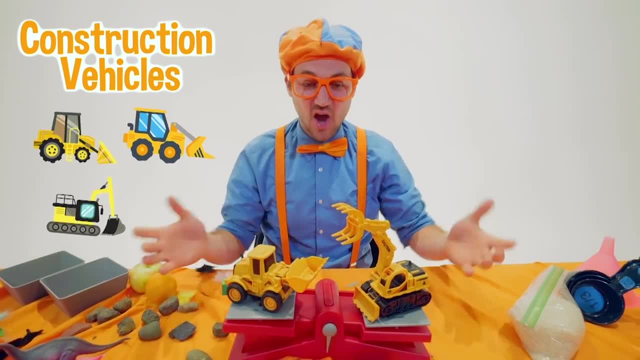 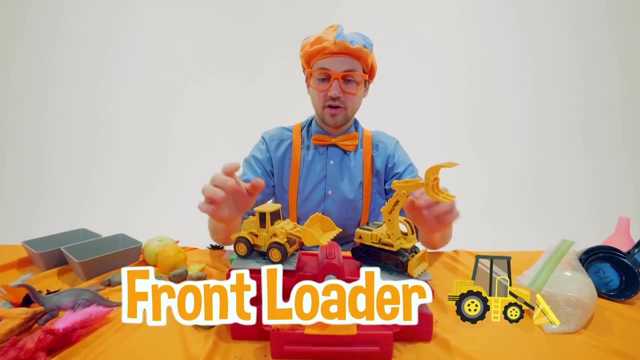 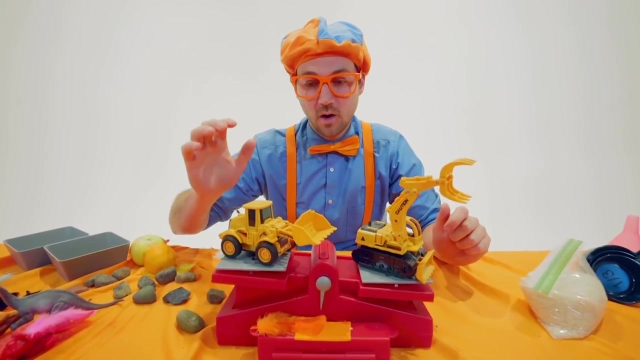 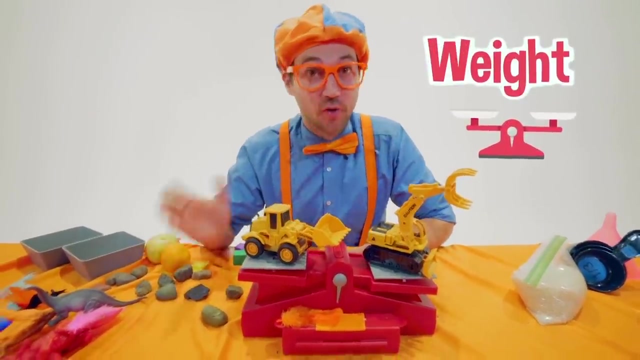 Yeah, construction vehicles are really heavy. Yeah, Like this exit road. Oh yeah, obviously, Excavator, or this front loader- Whoa, This excavator is actually heavier than this front loader toy. Oh Hey, I have an idea, since we're talking about weight and machines are really, really, really heavy. 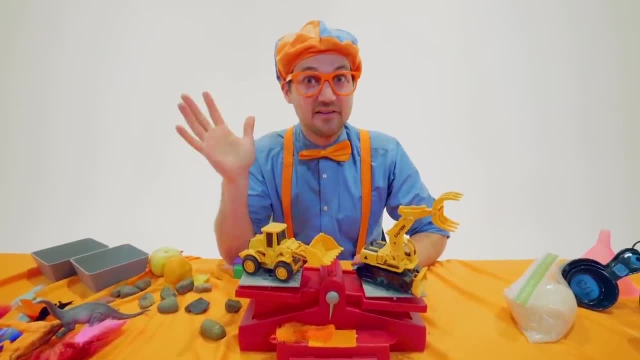 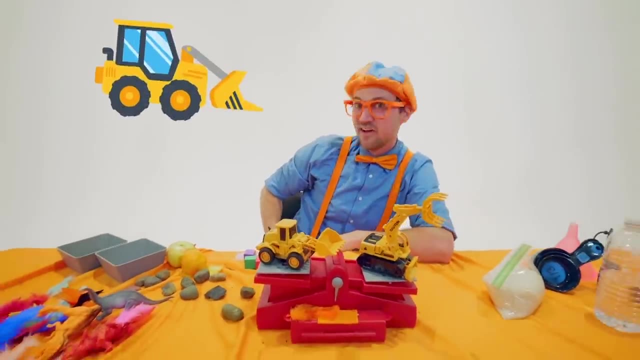 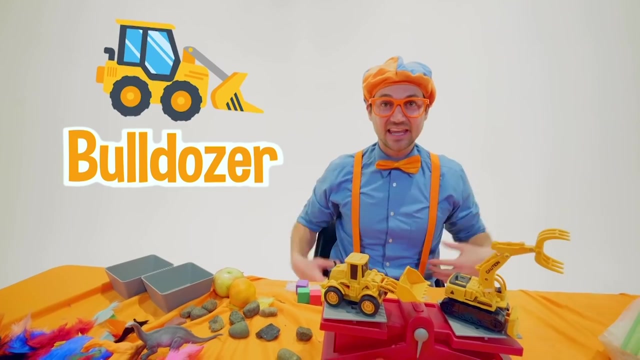 Let me think about a machine that is very heavy, low to the ground and can push Everything out of its way. Do you know what machine that is? Yeah, look at the big front blade on it. Yeah, that is a bulldozer. Hey, I think we should learn and watch the bulldozer video. 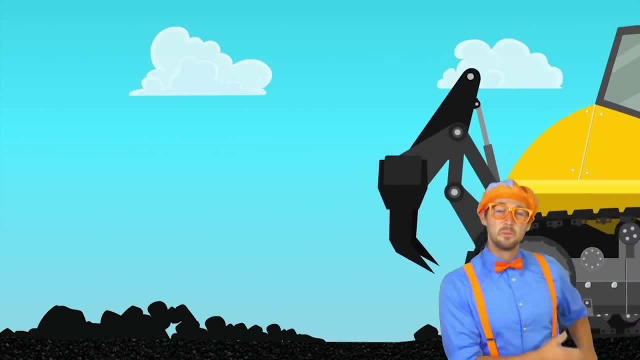 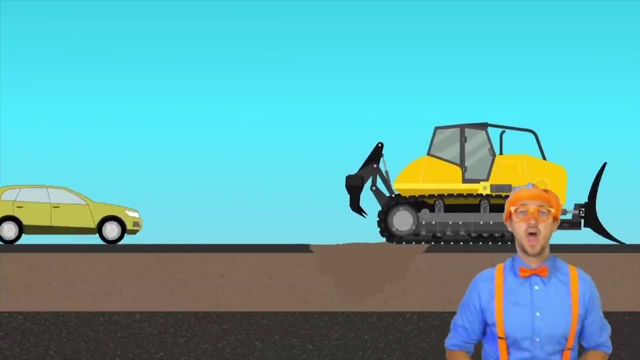 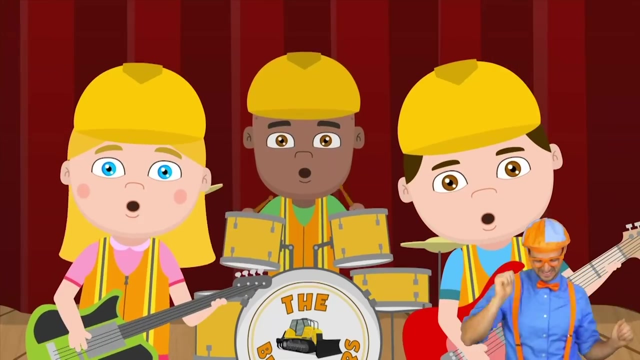 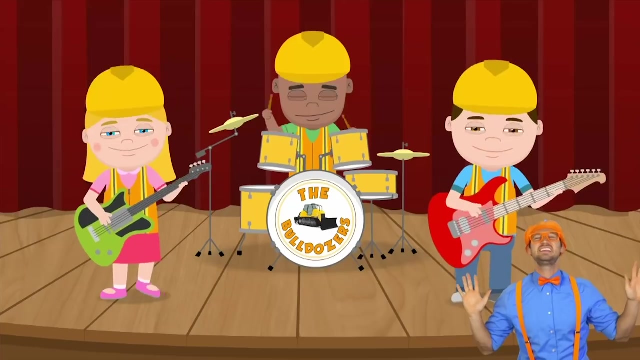 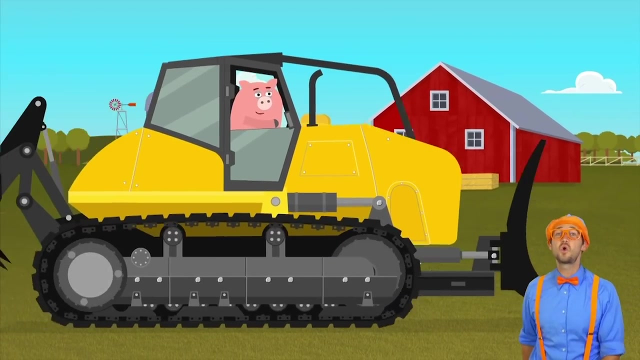 Bulldozer clear in the land. Bulldozer pushing rubble and sand. Bulldozer constructing the roads. Move-over, it's about to roll. It's a yellow tracked machine Found on mines, farms and factories. It can push most anything. Bulldozer stirring up debris. Bulldozers help the farmers work by breaking up rocks and digging in the dirt with the blade on the front. 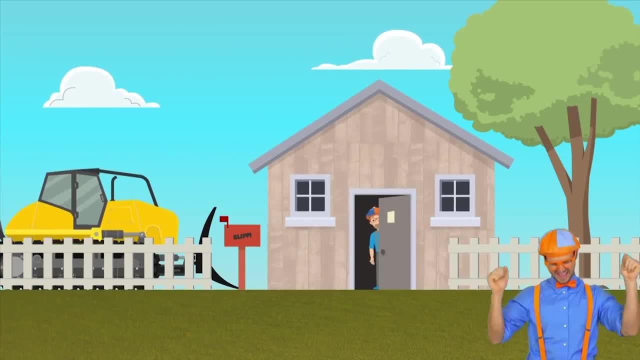 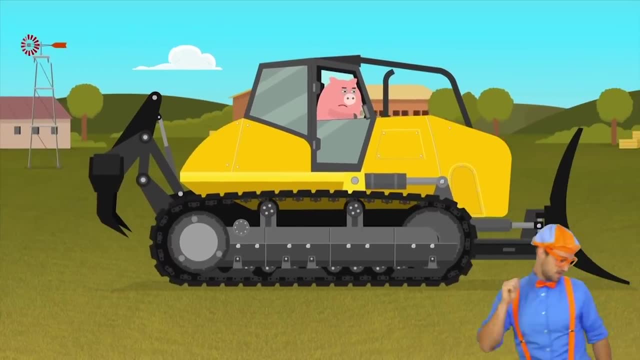 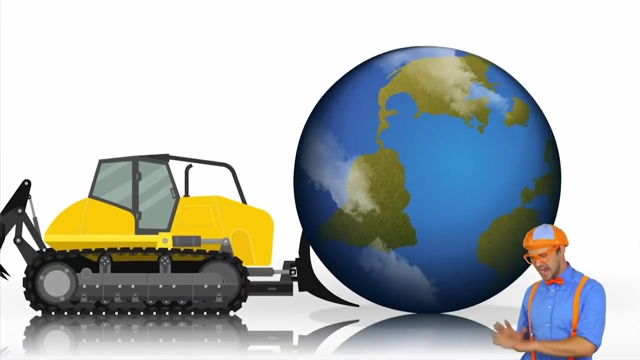 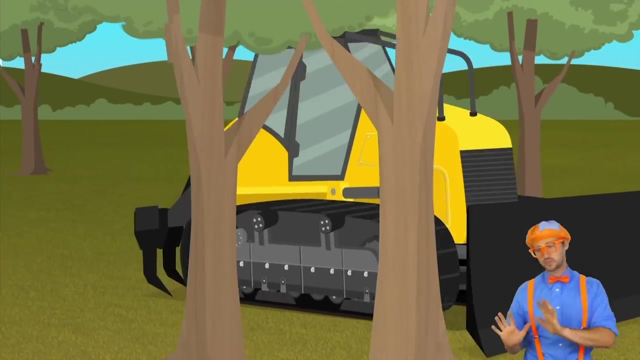 It can help you build a home just like that. It's on a roll Bulldozer And they can move through some rough terrain. They can move all kinds of things: Bulldozer clear in the land. Bulldozer pushing rubble and sand. Bulldozer constructing the roads. 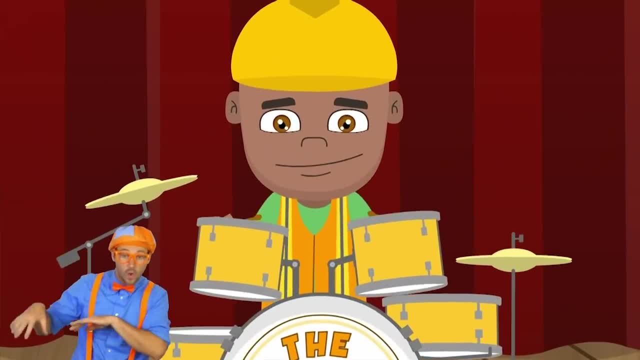 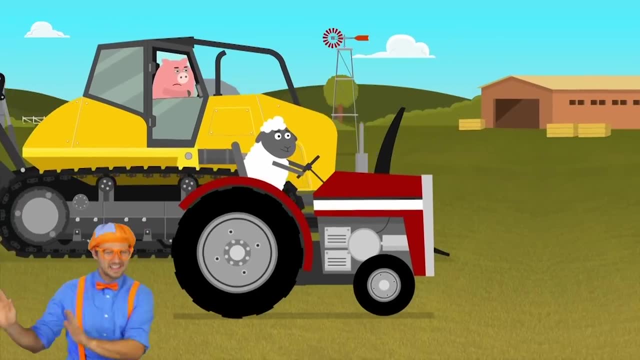 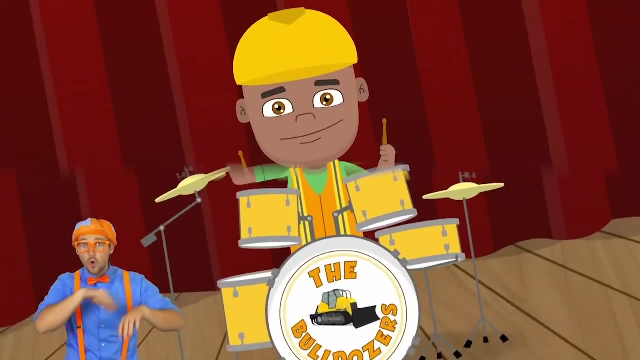 Move-over, it's about to roll. Bulldozer: clear in the land. Bulldozer pushing rubble and sand. Bulldozer constructing the roads. Move-over, it's about to roll, Roll, roll on bulldozer. You better move over. here comes the bulldozer. 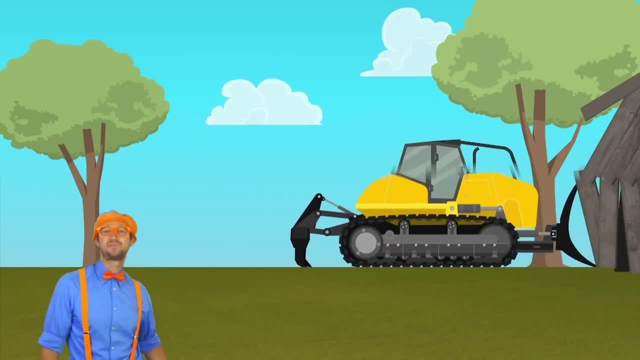 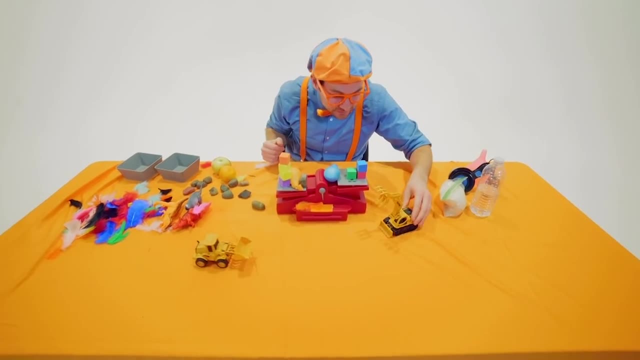 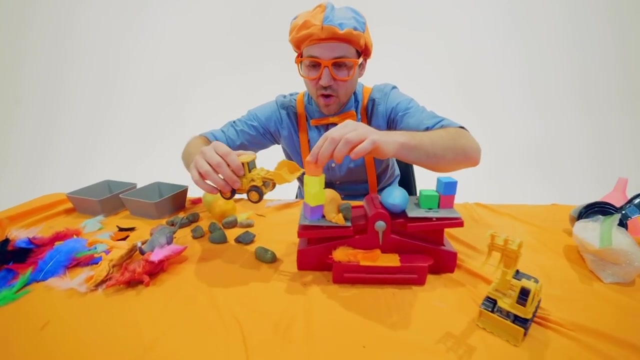 It's a yellow machine. Roll, roll on bulldozer. You better move over. here comes the bulldozer, It's a yellow machine. It's a yellow machine. Instead of Thyme Vroom, vroom, vroom, right foot in the blocks, here we go, go to the other side, dump them. 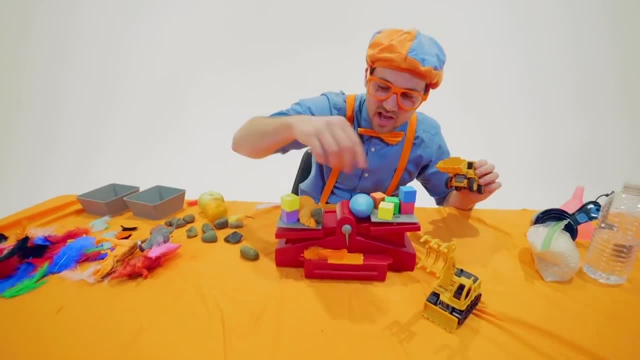 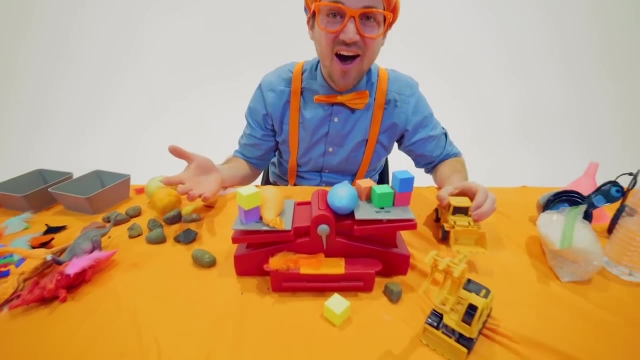 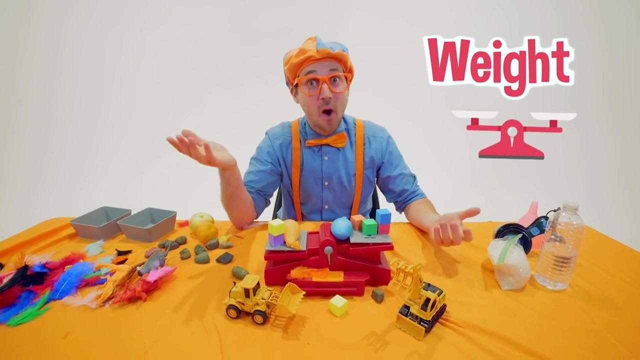 out there we go two more blocks on this side. hmm, let's see, maybe the rock will make it heavy enough. whoa, it for sure was heavy enough. wow, that was so much fun learning about weight with you. and also bulldozers- wow, those machines are so heavy. well, this. 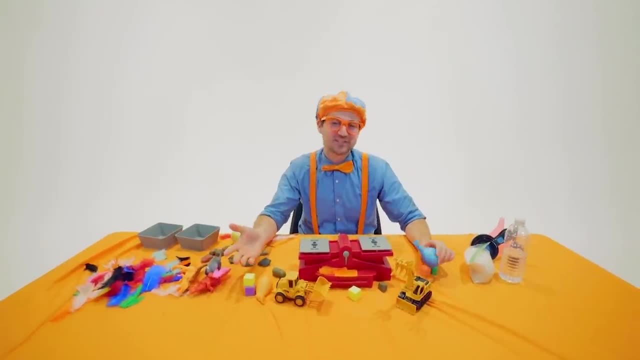 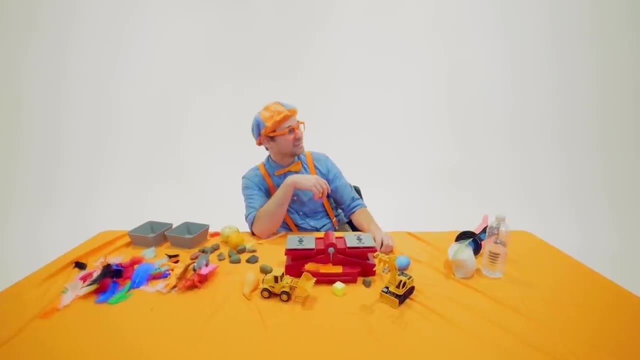 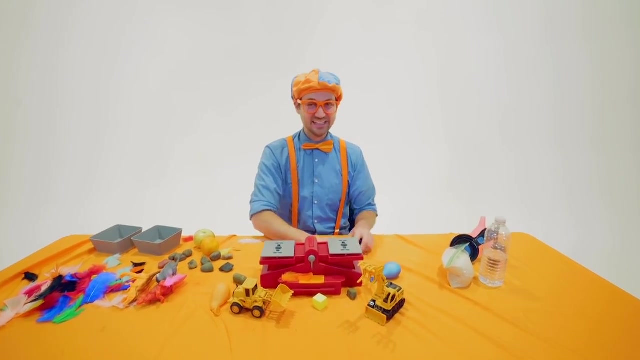 is the end of this video, but if you want to watch more of my videos, all you have to do is search for my name. will you spell my name with me ready? B-L-I-P-P-I. Blippi, good job. alright, see you again, buh-bye. 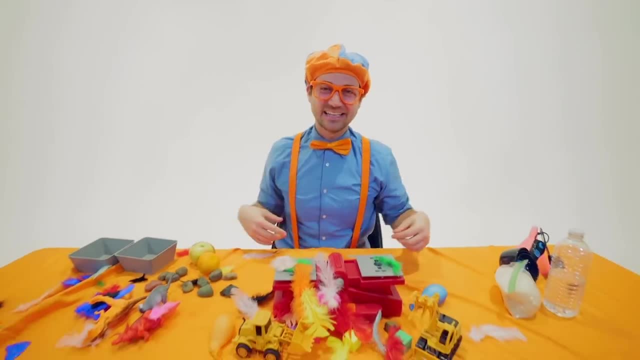 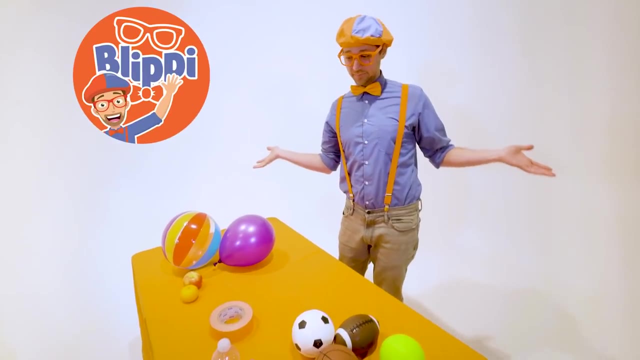 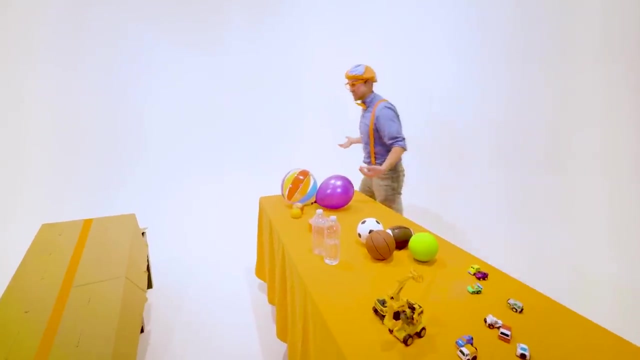 Okay, I'm going to clean up now. hey, it's me Blippi, and look at all the items that I have. whoa, so many random things. but hey, in this video we are going to do the Blippi. 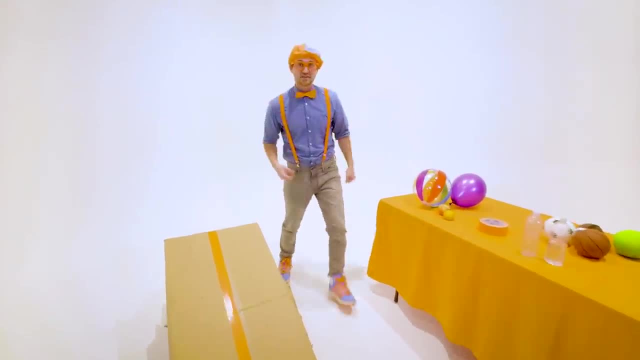 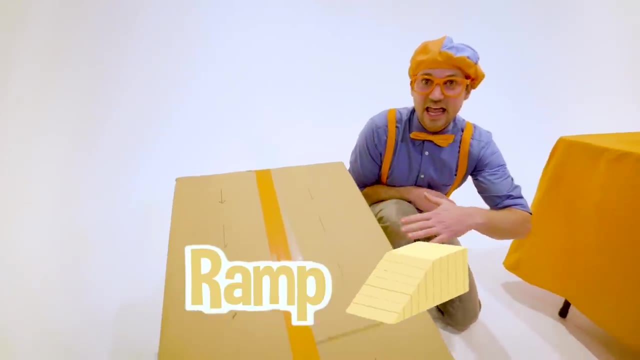 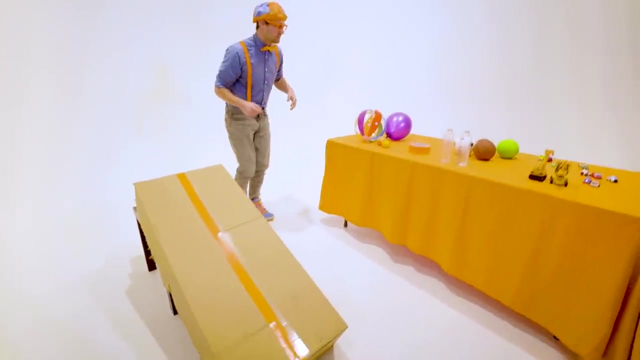 velocity race. yeah, that's where we put a lot of these items on this ramp and we're going to see how this ramp is at an angle. yeah, we're going to let them go at the same time and see what item reaches the bottom first. okay, so let's go with heat number. 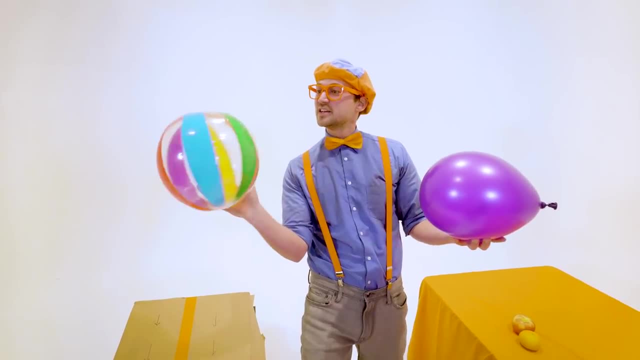 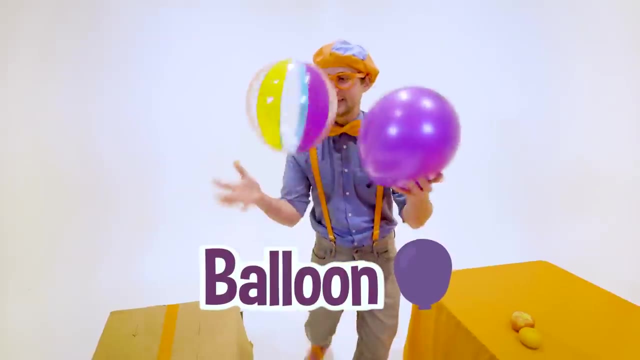 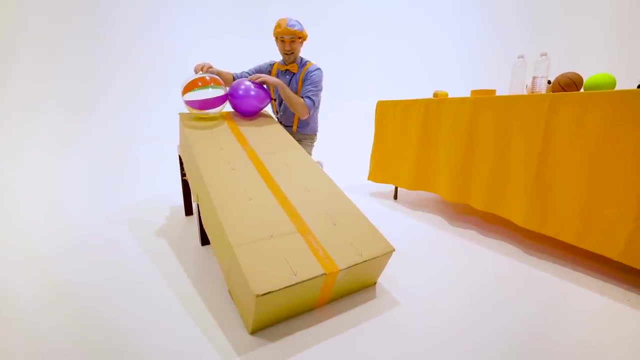 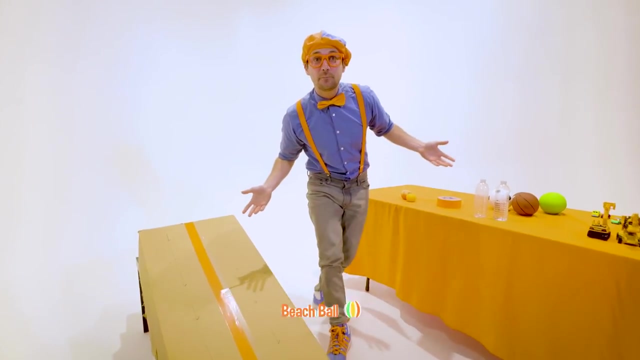 one, the slow pokes. we have this sweet colorful beach ball and then we have this really light balloon. okay, alright, what one do you think is going to reach the bottom first? I think I know Three, two, one, whoa. did you see that? yeah, the beach ball went to the bottom first. 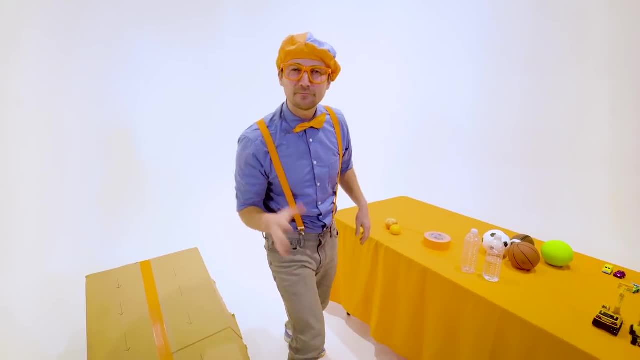 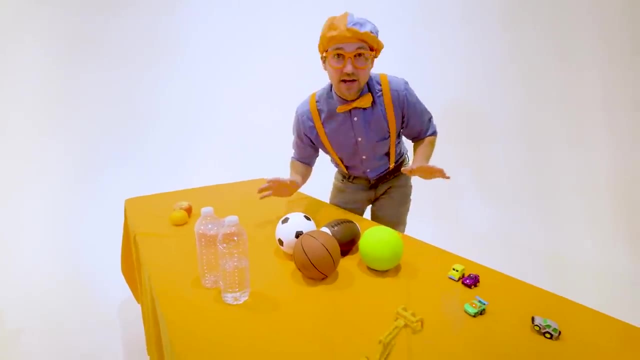 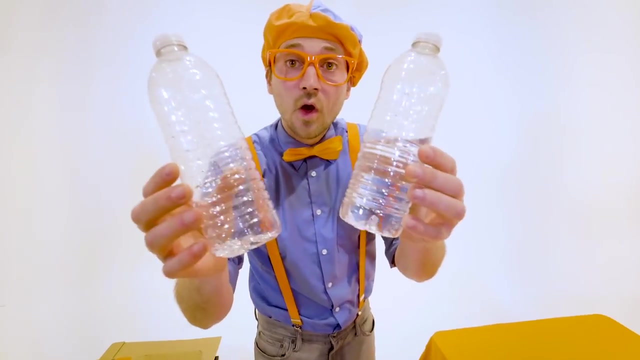 okay, let's let them just- you know- get warmed up for later, and then we'll use some more items. yeah, I'm sure all these items are going to be a lot faster. okay, here's another set of items. they're actually the same item: water bottles, yeah. 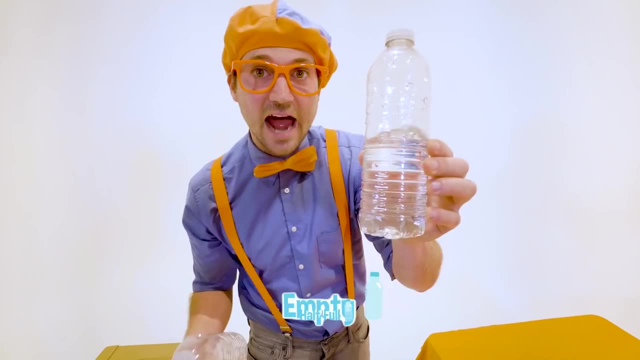 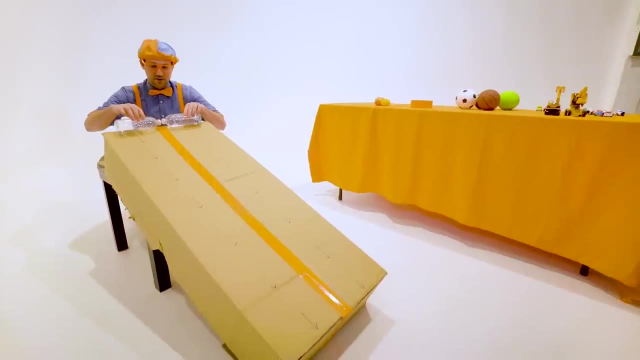 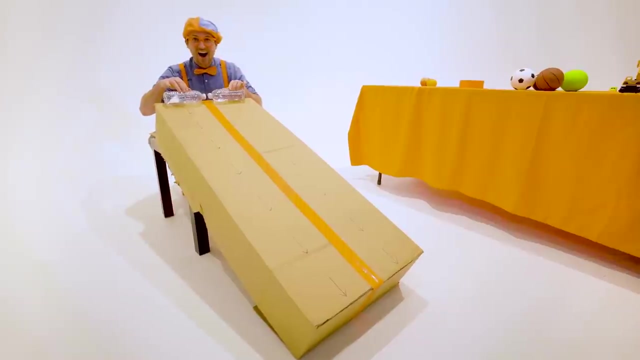 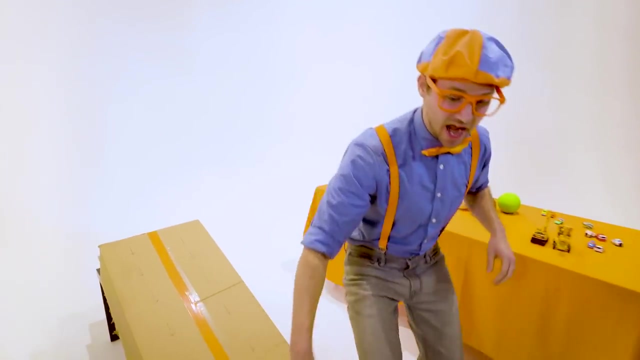 But this one is empty and this one is half full, haha, alright, let's put them on their side and then let's let them roll down. okay, are you ready? yeah, I'm ready. are you ready? oh, I'm ready. awesome, three, two, one, whoa, yeah, wow, the half full water bottle totally. 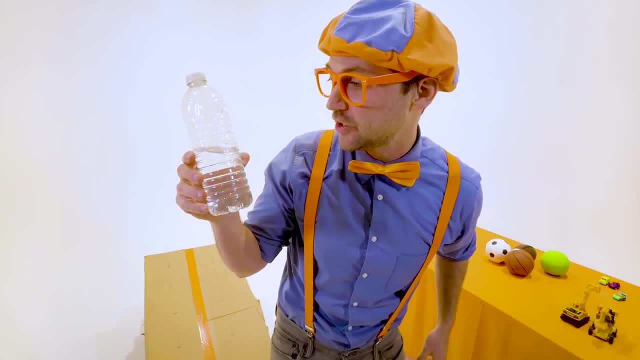 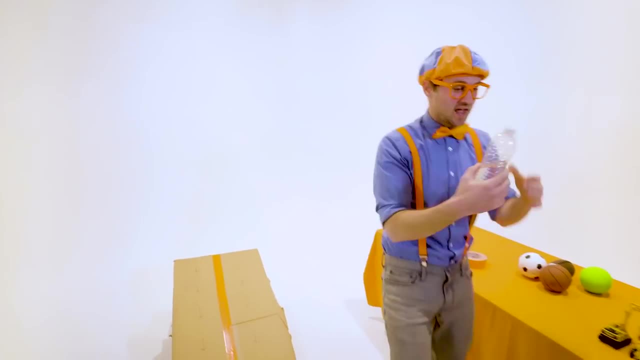 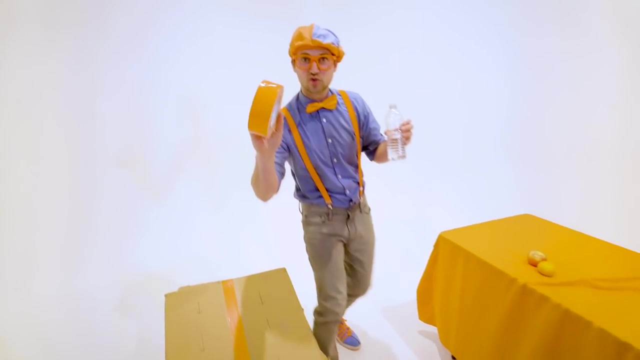 beat the empty water bottle. how do you feel after your race? half full water bottle- Oh Blippi, I feel amazing. I can't believe I've won. great well, it's going to move on to the next race. half full water bottle versus extremely bright orange duct tape. 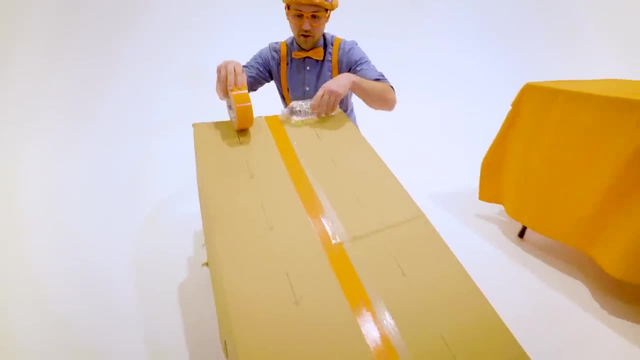 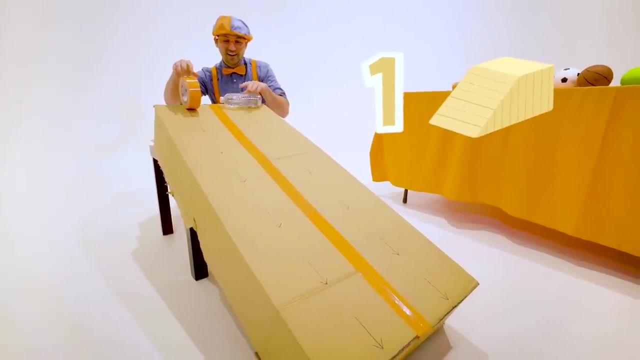 haha, alright, here we go. are you ready? ready to race? are you ready? you know, I'm ready. alright, Three, two, one, whoa, whoa. did you see that? yeah, the water bottle rolled down. 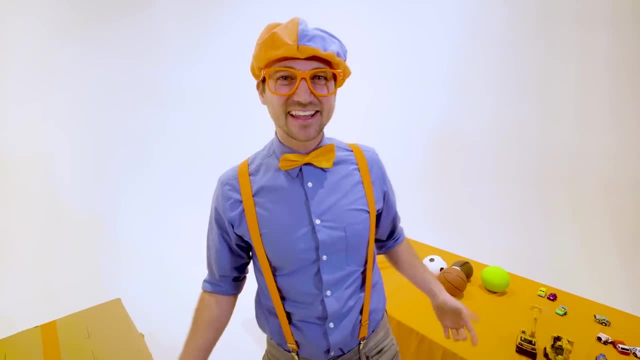 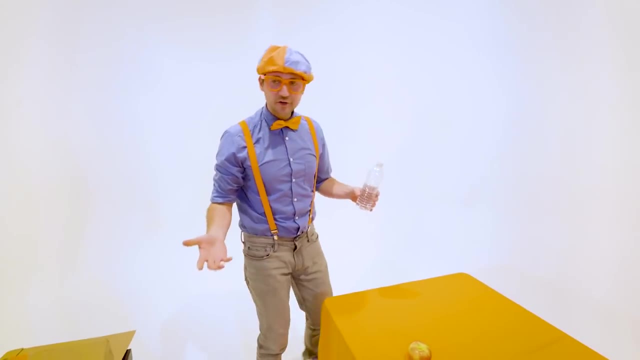 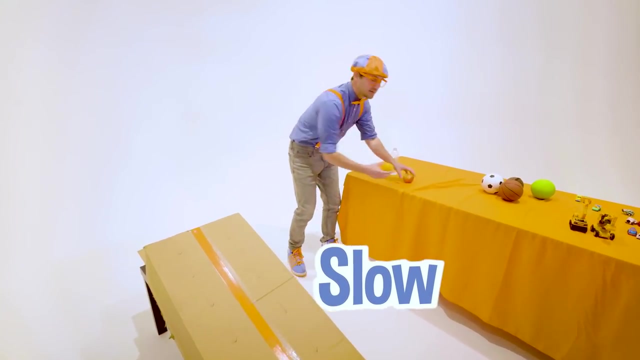 way to the bottom. way quick, way, faster than the duct tape. perfect, so now it can move on to the next round. have you ever wondered why these items some go fast and some go slow? yeah, it's because their velocity. yeah, velocity is basically, you know, the 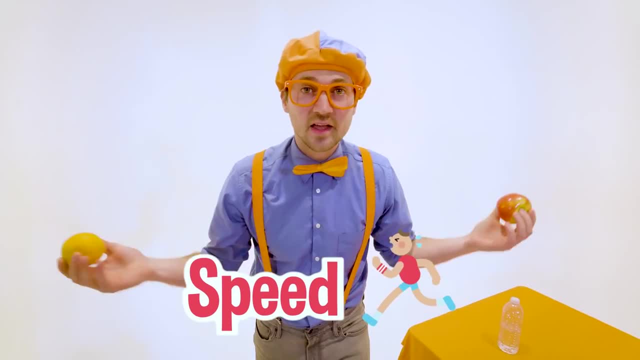 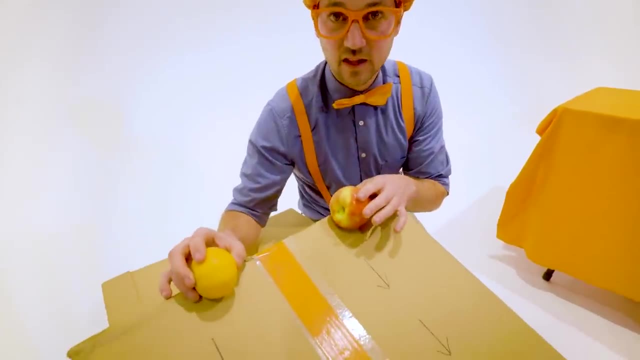 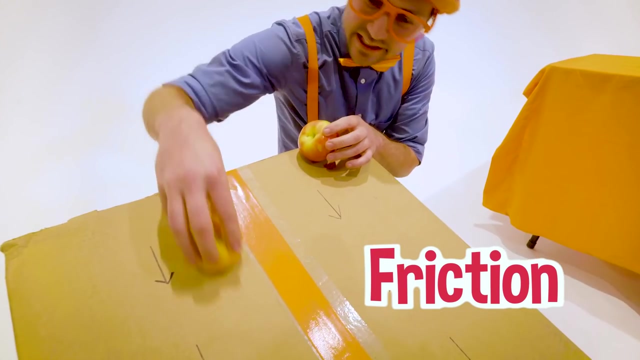 speed at which they're rolling down the speed and the direction. yeah, there's a lot of things that actually determine what the item's velocity is. I mean, like, think about it like this: there could be a lot of friction and it like can't slide, or maybe it rolls. 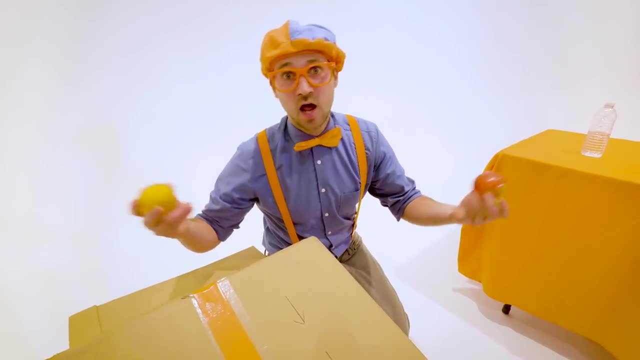 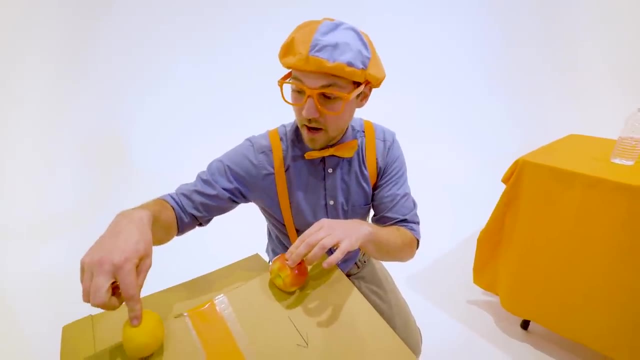 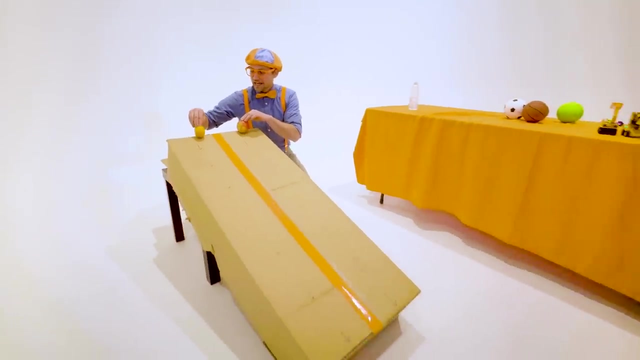 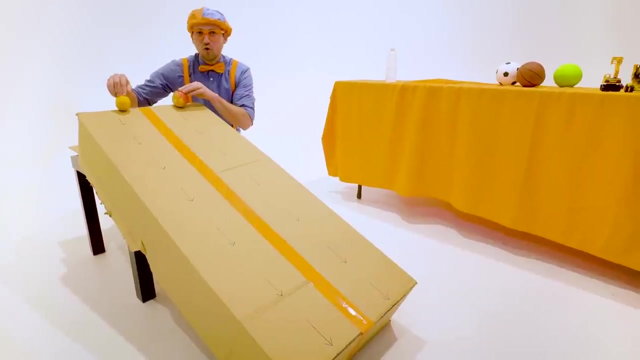 compared to you know, maybe there's sharp edges. there's just so many things that you know determine how fast, How much velocity these items have. so let's let these two items go. we have orange over here and apple over here and let's see who wins go. whoa, they were actually really. 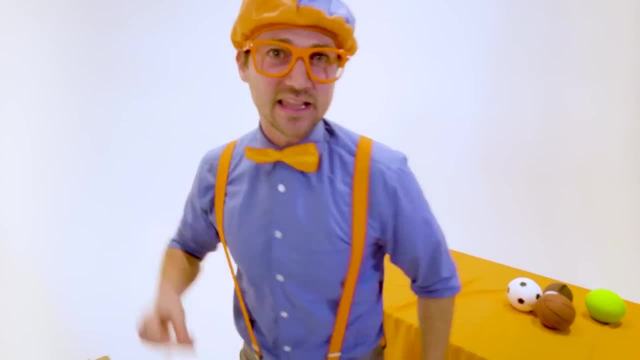 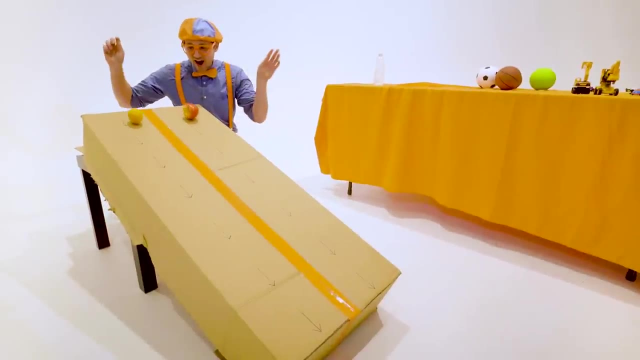 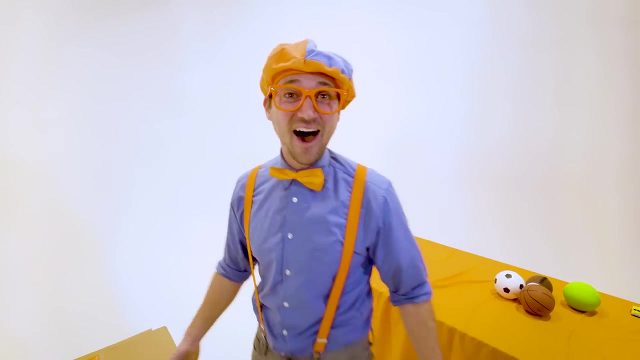 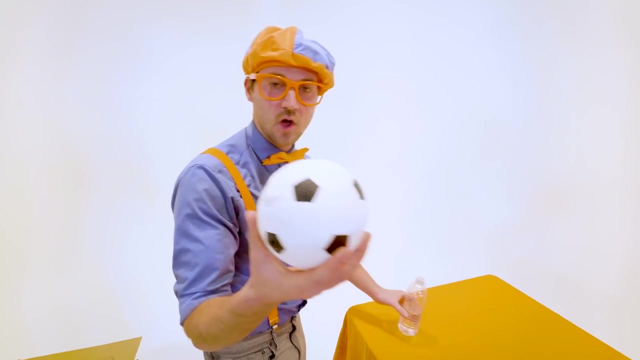 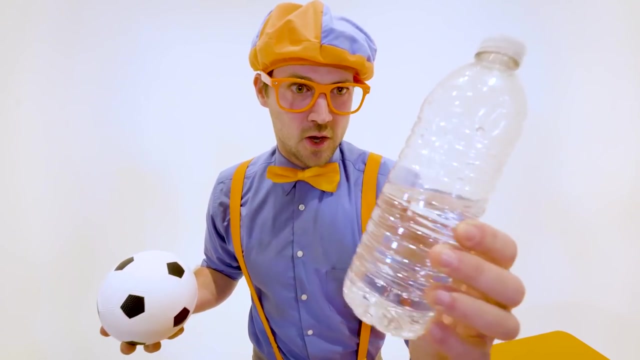 close to each other. I don't even know who won. let's see that instant replay. Whoa, that was awesome. All right, let's pick two more items. we have a soccer ball or a football, depends where you live- and the half full water bottle. the champion. 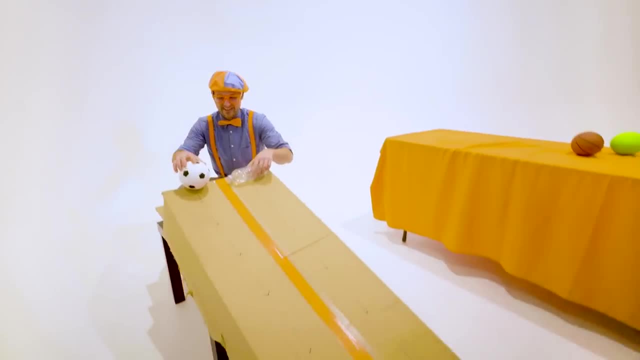 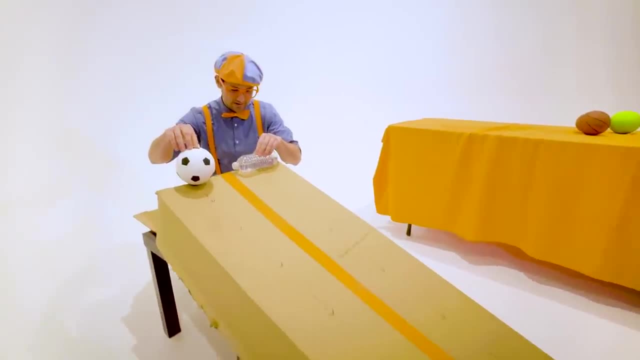 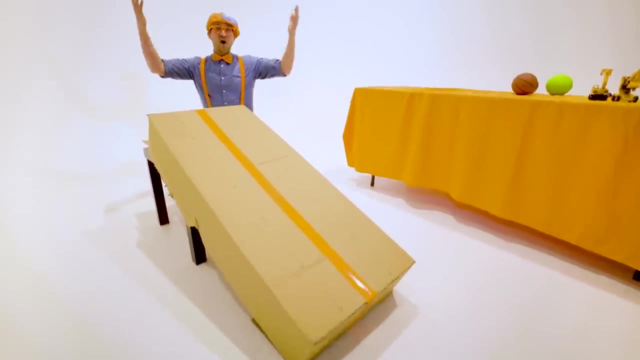 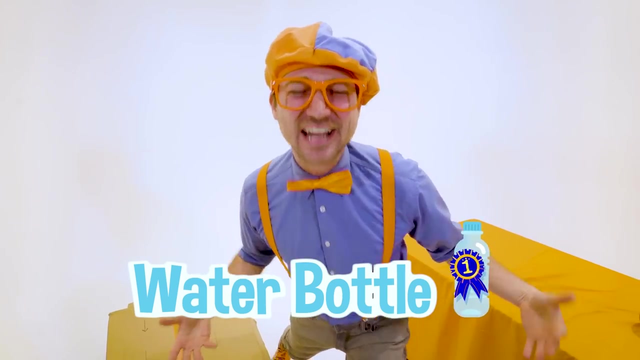 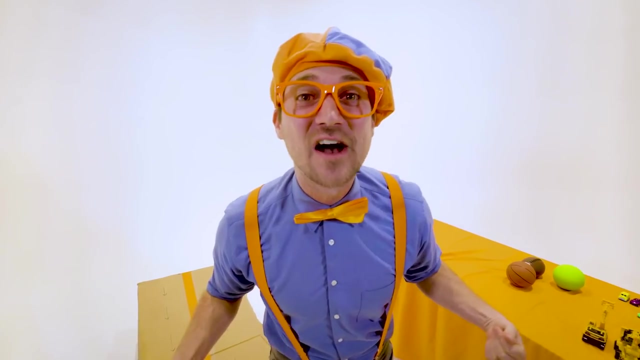 I'm good to go. Are you ready? I was born ready. All right and away we go. Whoa, I cannot believe it. the half full water bottle wins the velocity race. whoa, and the crowd goes wild. Wow, that was awesome learning about water. 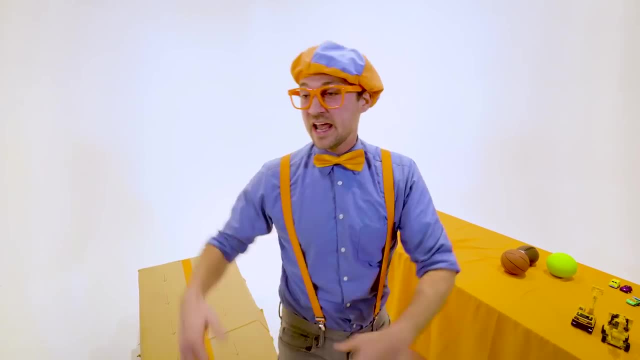 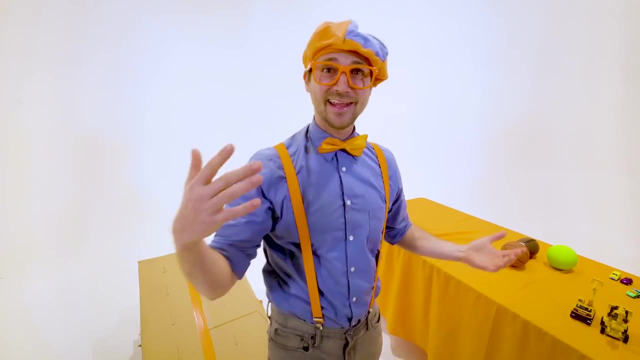 Wow, that was awesome learning about velocity and how fast that water bottle went and how the ramp is angled. but yeah, if the ramp was flat it definitely wouldn't go anywhere, right, Yeah, hey, can you think of a machine? that is actually really fast. 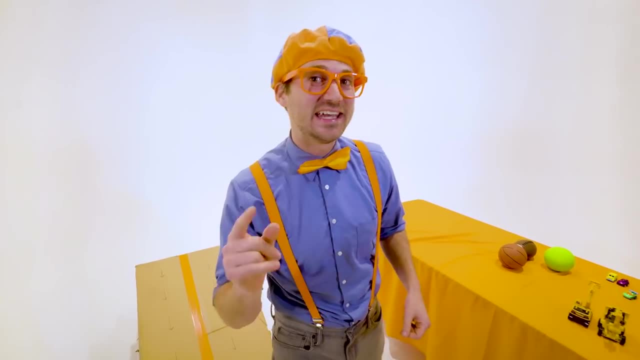 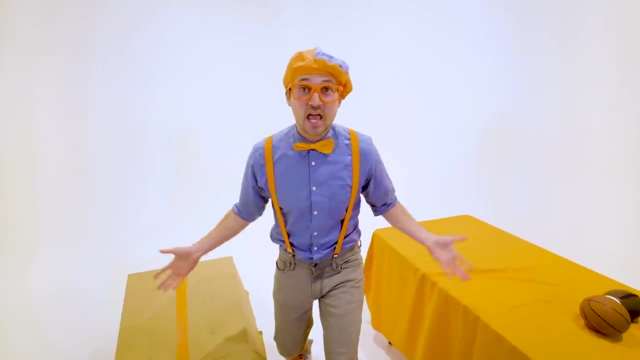 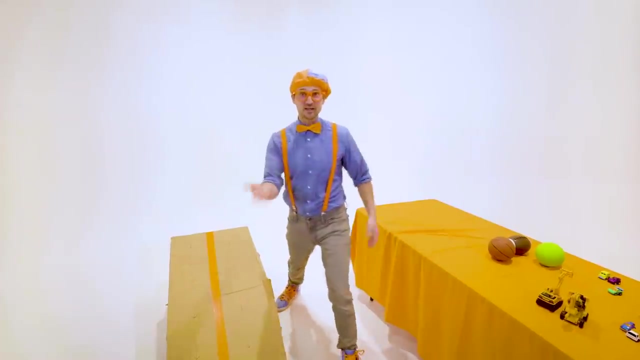 Yeah, there's a lot of them. Okay, let me give you a hint. okay, this machine does not go on the ground. well, it does, but then it goes in the air. Yeah, Whoa, I hear one. yeah, maybe you've got to fly in one before. 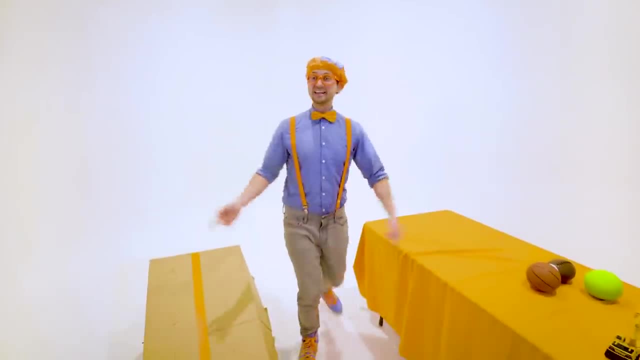 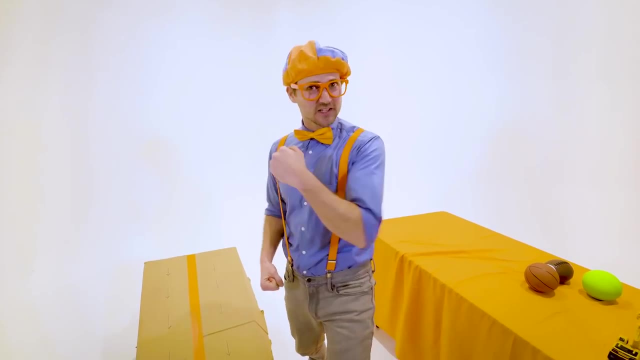 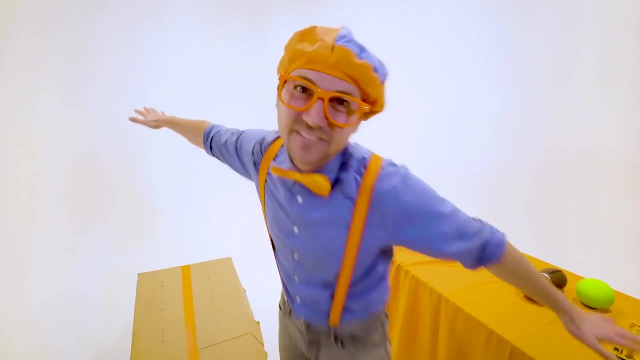 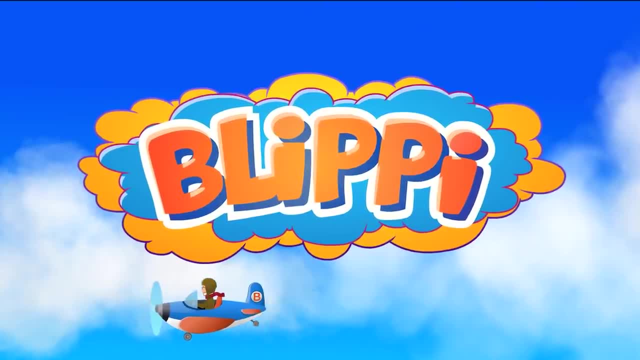 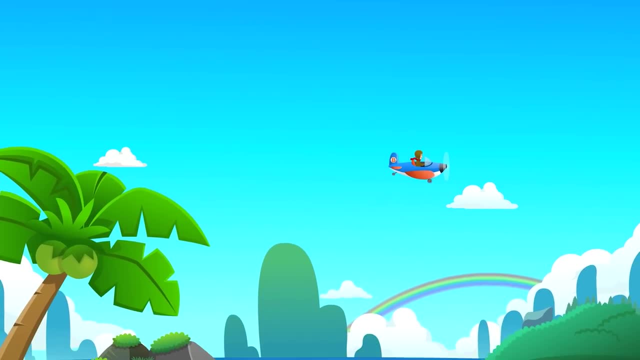 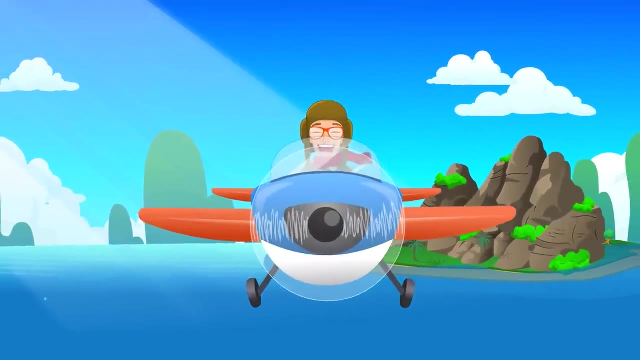 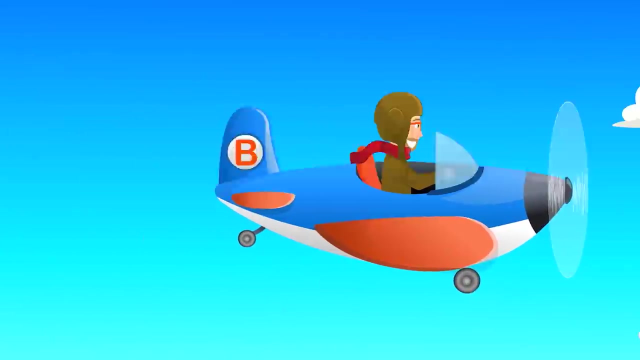 Woo, Woo, Woo, Woo Woo. Airplanes, airplanes flying all around the sky. Airplanes, airplanes flying way up high. Some airplanes are as big as a building, Some are a roof over it, And if you need a hand, then use a control center. 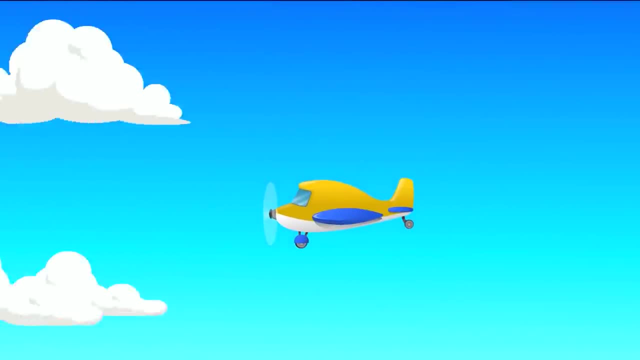 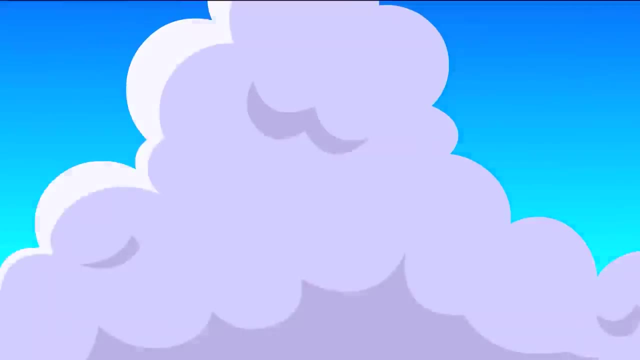 It is a great place to do that. It's good for quelque Kombat. Some are as small as a car. That's amazing. Some airplanes transport people. Some fly near to the stars- That's far. Some airplanes fly with propellers. Some airplanes fly with jet engines. 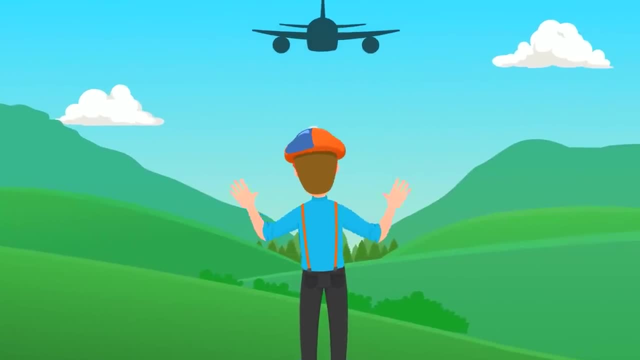 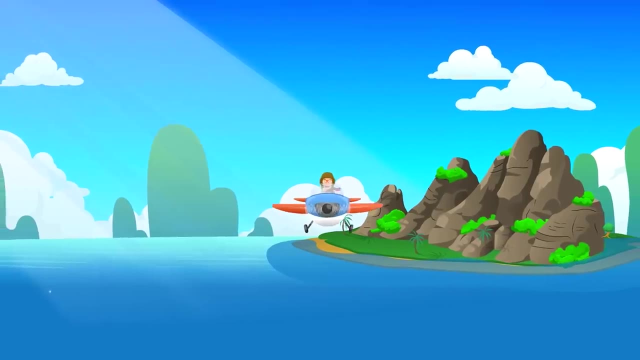 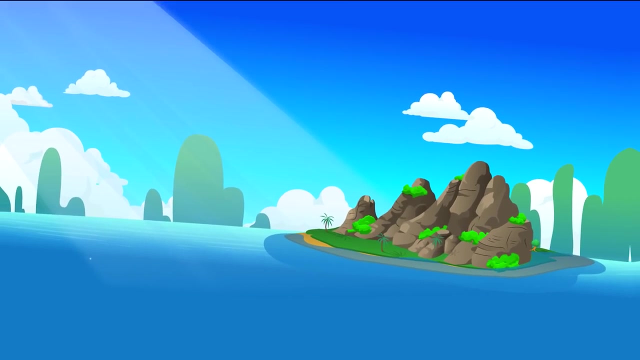 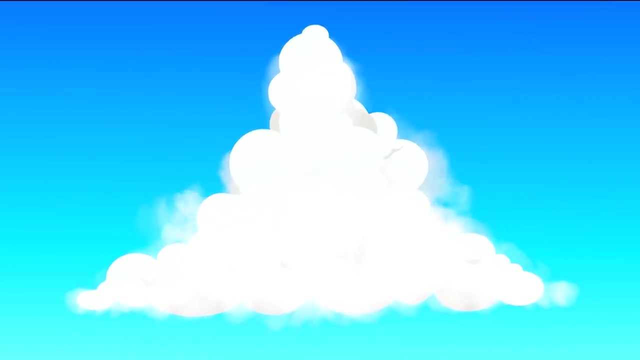 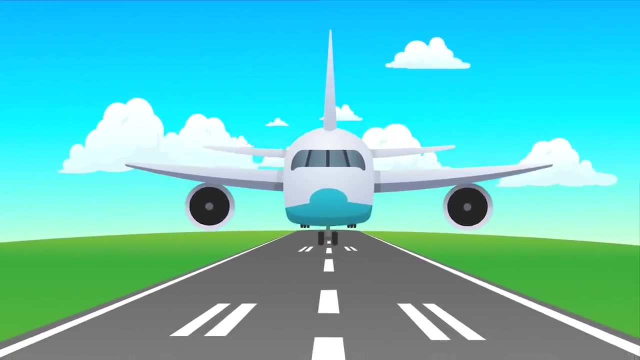 I love to look up and see their wings Waving down at me. Hey, airplane, Airplanes, airplanes Flying all around the sky. Airplanes, airplanes Flying way up high. Some airplanes can land on water, But most land on landing strips, So versatile Some airplanes fly just for fun. 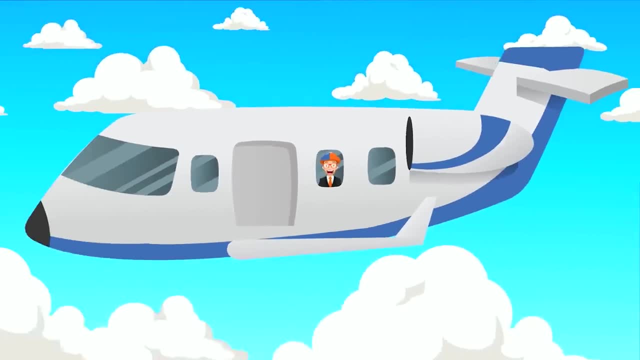 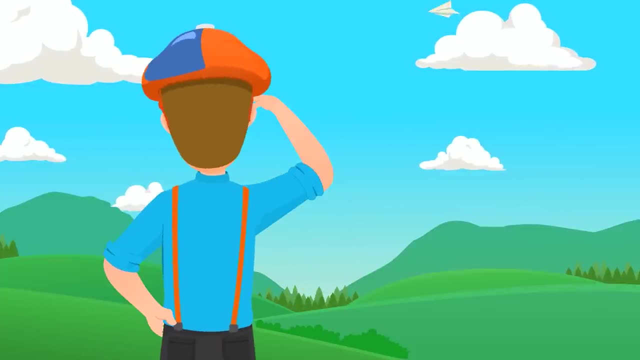 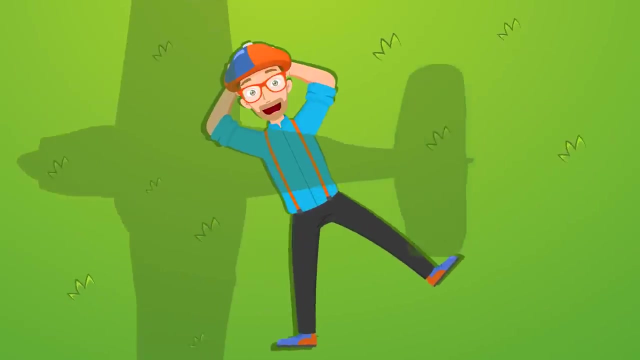 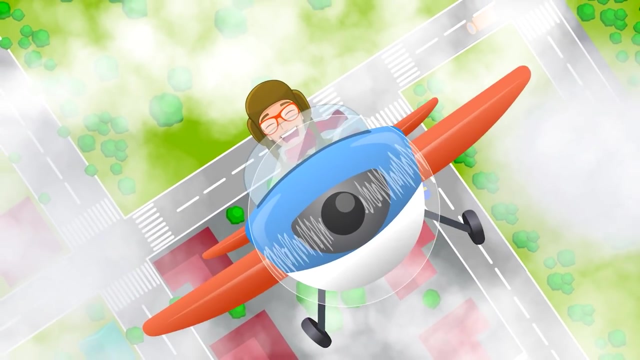 Some fly for business trips, Business or pleasure. You can make an airplane out of paper, Throw it in the air and watch it go. I love to look up and see its wings Waving down at me. Hey, airplane, Airplanes, airplanes Flying all around the sky. 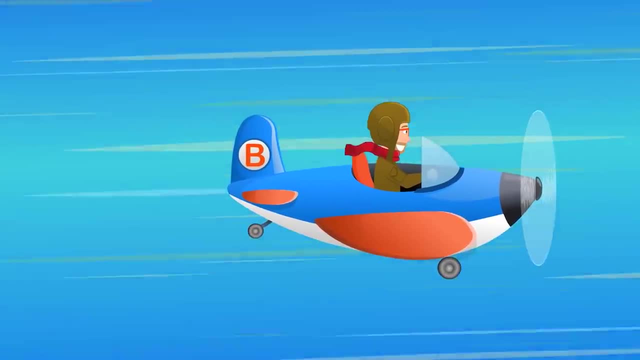 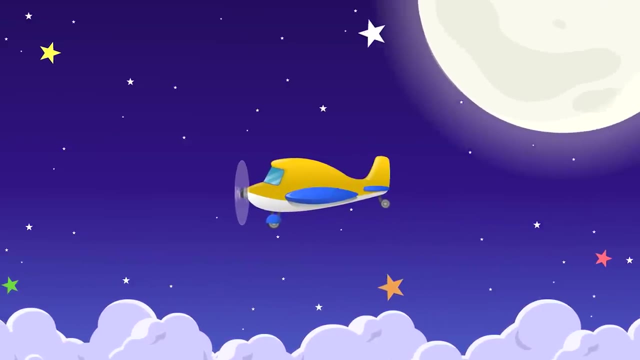 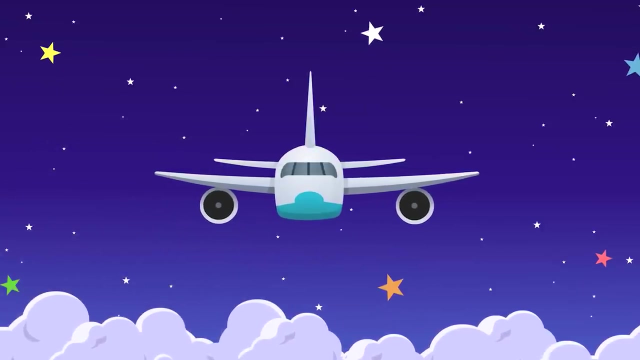 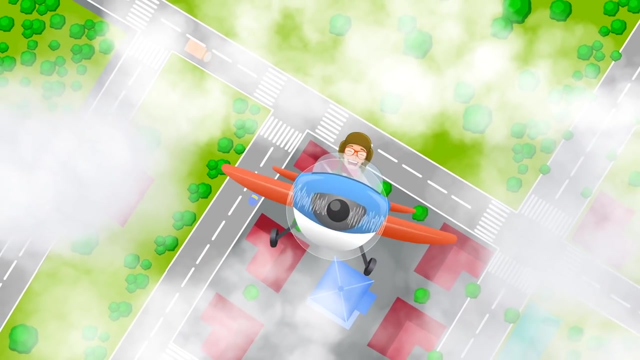 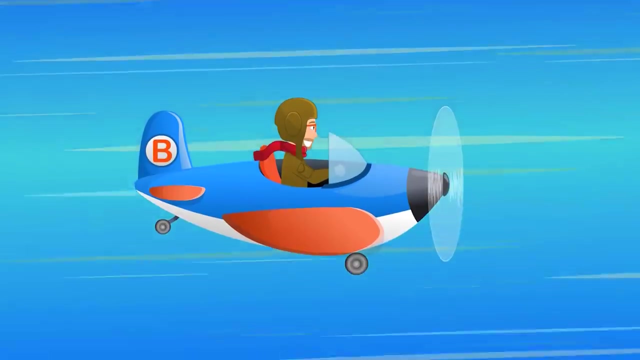 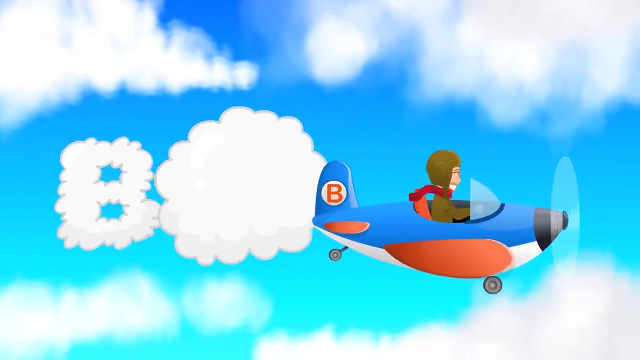 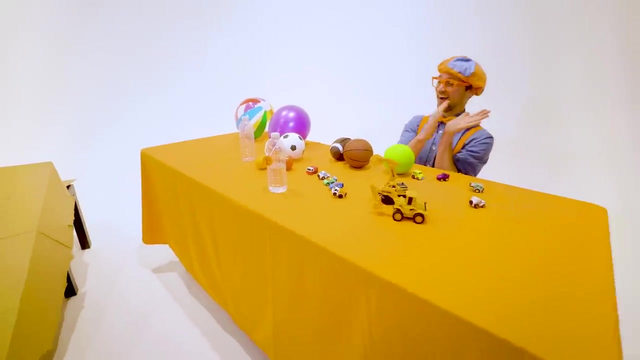 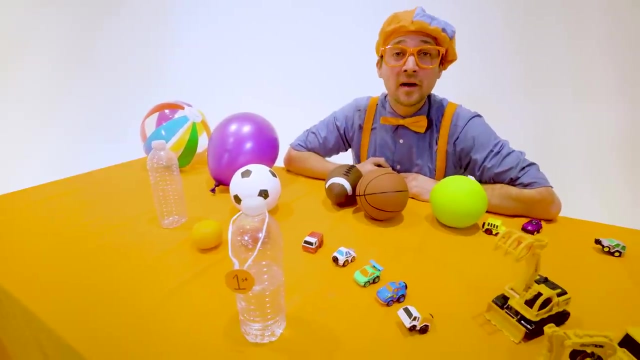 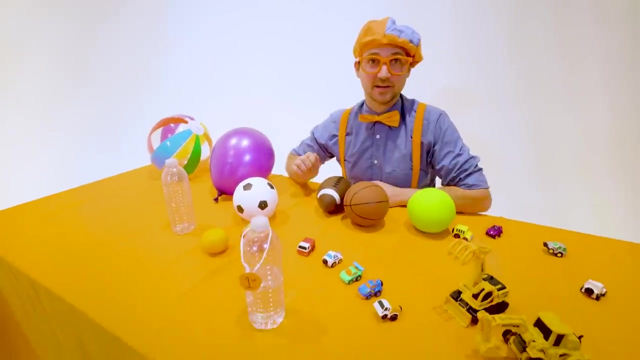 Airplanes- airplanes Flying way up high Airplanes- airplanes Flying all around the sky. Airplanes- airplanes- Ah, who's that? Wow, Wow, Good job. water bottle- Wow, That was so much fun learning about velocity with you And it was really fun seeing. 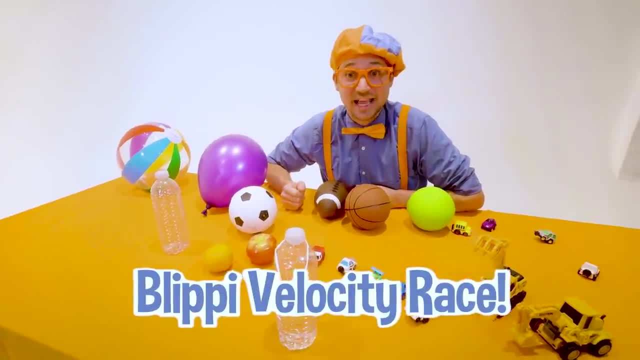 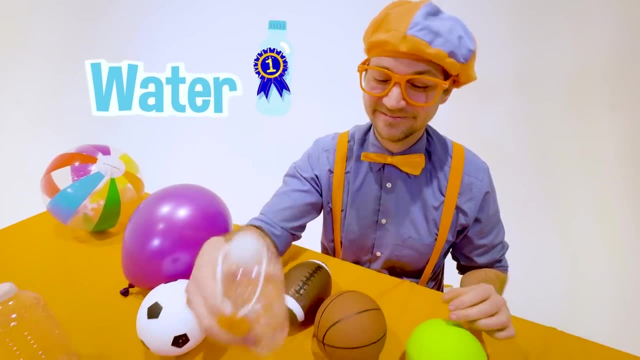 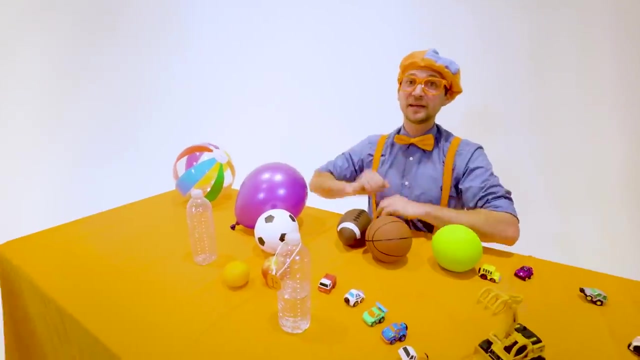 at the great Blippi Velocity Race, But there's only one champion, and today that was water, Wow. Well, this is the end of this video, But if you want to watch more of my videos, all you have to do is search for my name. 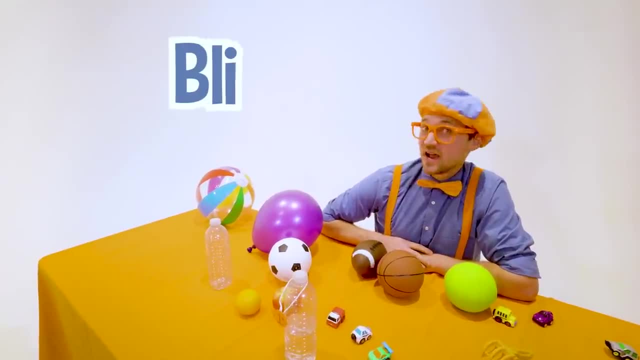 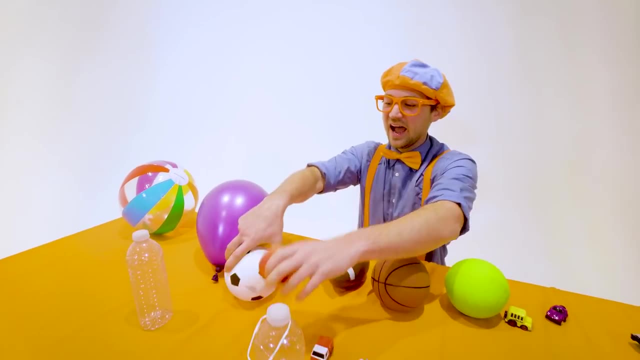 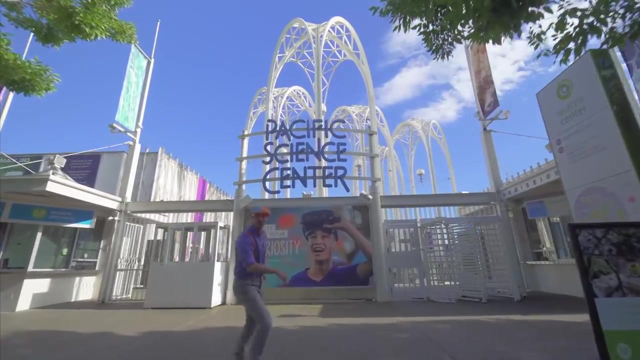 Will you spell my name with me: B-L-I-P-P-I. Blippi, Good job, All right, see you again. Buh-bye, Hey, it's me Blippi, And today we're at the Pacific Science Center. 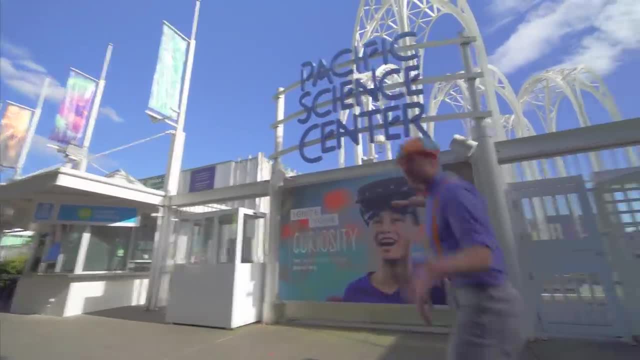 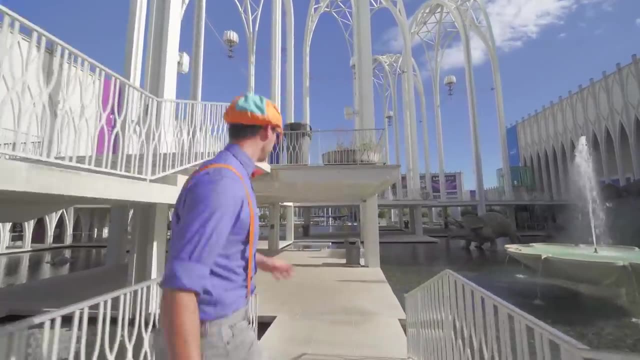 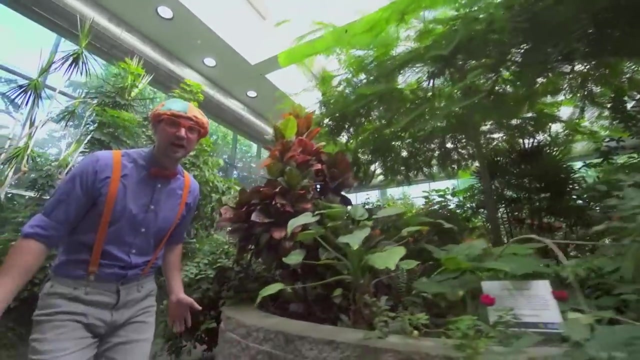 in Seattle Washington. This is going to be so much fun. Come on, Whoa, Look at this place. This place is awesome. Ooh, Now we're in the butterfly room. Have you ever seen a butterfly before? Yeah, 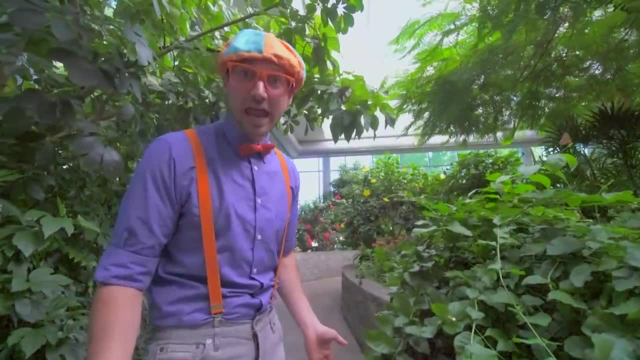 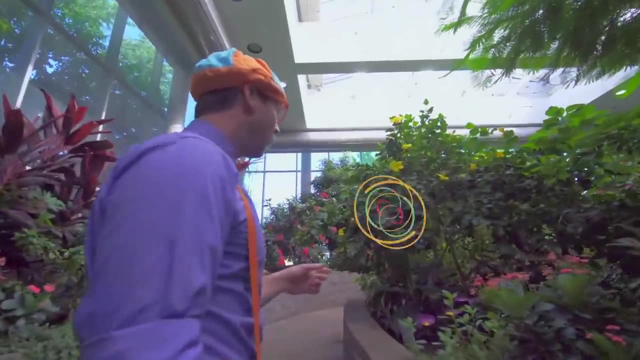 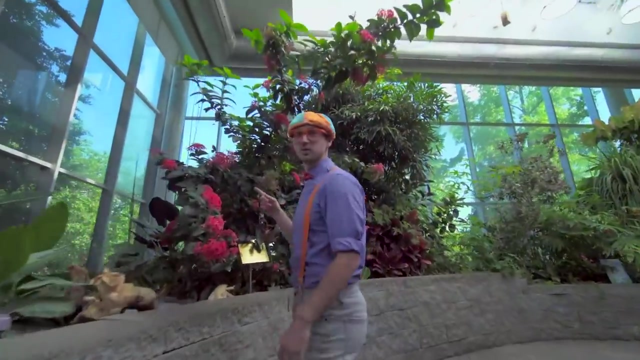 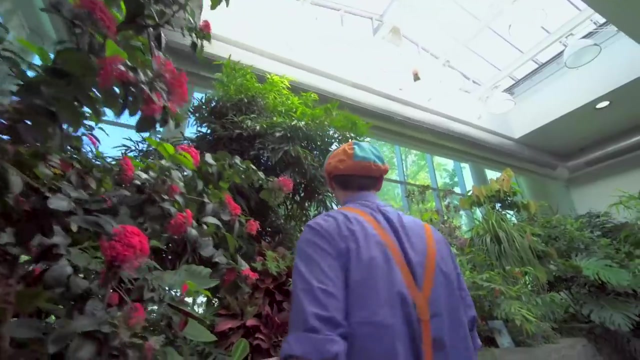 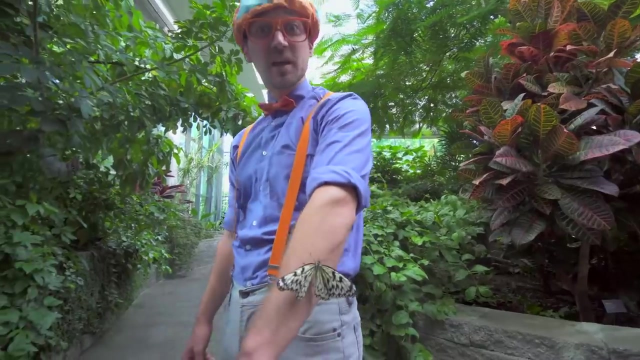 I love butterflies. They're so beautiful and light. Will you act like a butterfly with me? Whoa, Look at him, go, Whoa, There's one right there. Hey, butterfly, Whoa, Whoa. Ah, Oh, there is a butterfly. 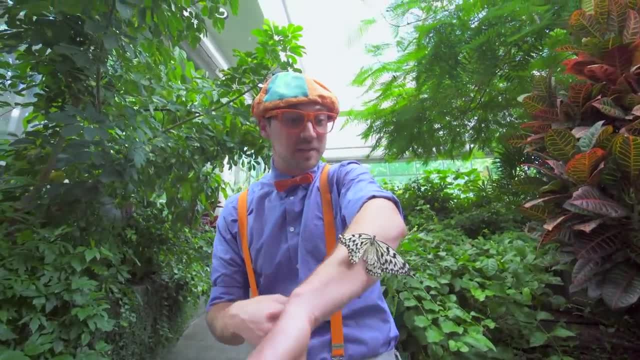 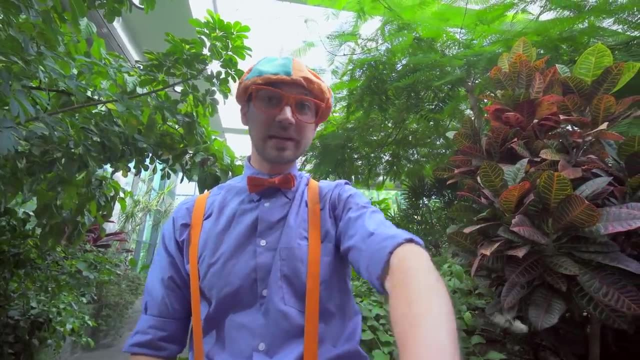 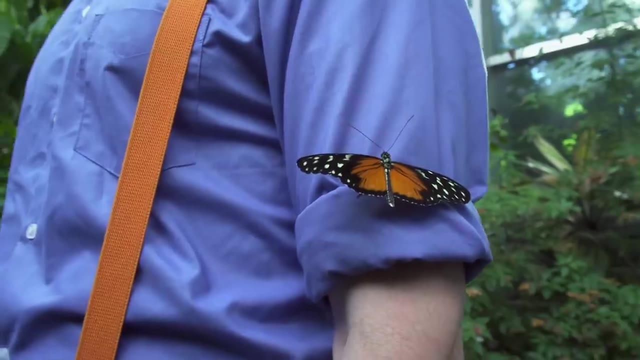 Check it out. A butterfly just landed on me. So anytime they land on you, you don't want to touch them and they're actually just being really nice, So you can be nice back to them, See, Ha-ha. 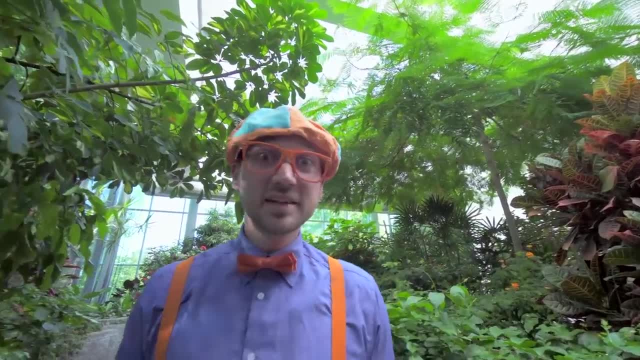 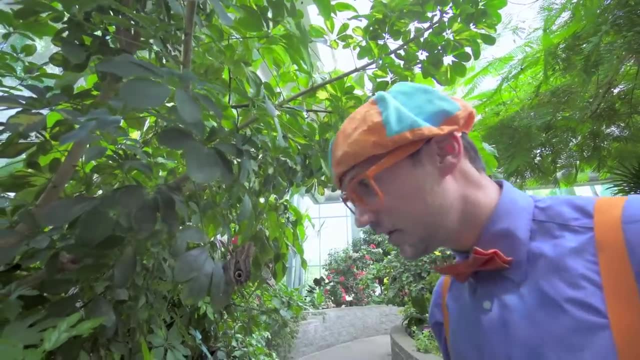 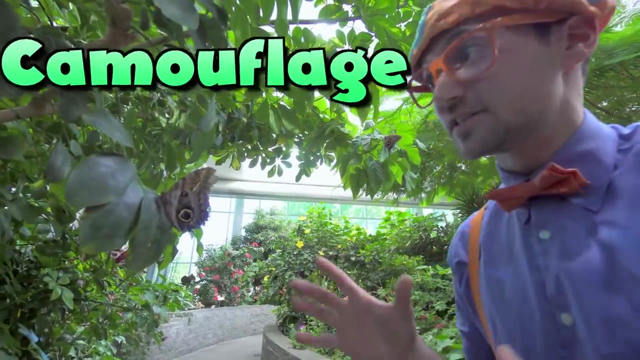 I love butterflies because they're so bright And some are camouflaged. though, Look, can you find one? Whoa, look, This butterfly uses camouflage for its defense mechanism, just in case, if there's any predators, then the predators can't see it. 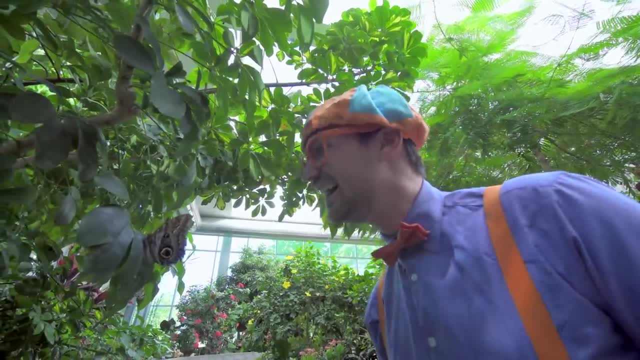 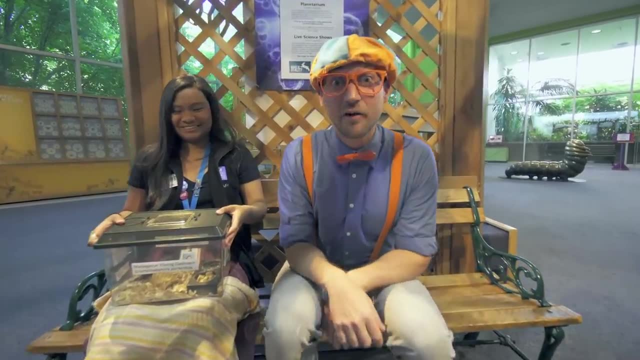 See, Hi All. right now I'm with Lorraine, and what are you gonna show us? So this here is a Madagascar hissing cockroach. I can take it out for you. What am I gonna do with it? You can hold it if you'd like. 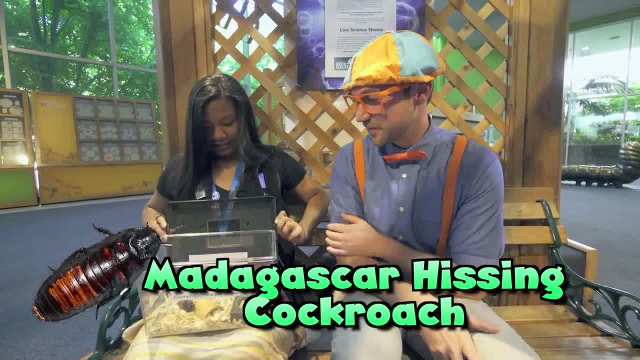 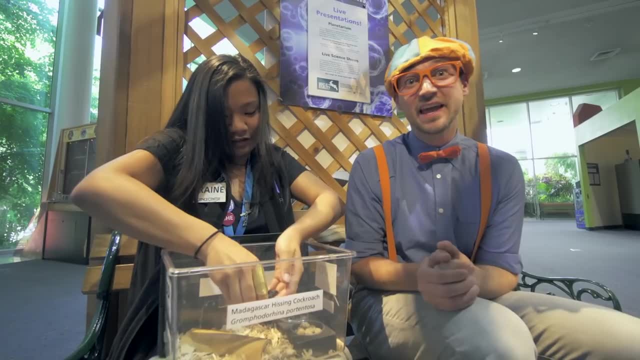 Sure, let's try it. I'm about to hold a Madagascar hissing cockroach. All right, hold your hand out. really, still There you go. Oh, that's a good one, I'm gonna hold it. I'm gonna hold it. 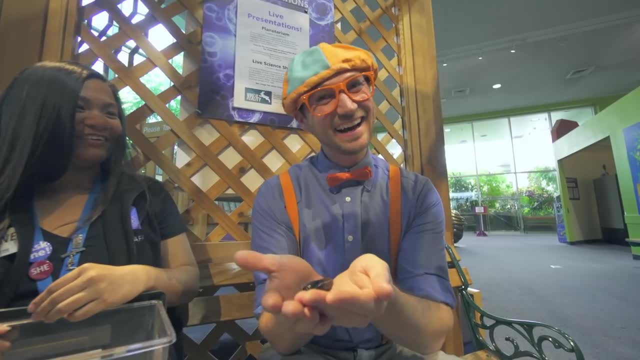 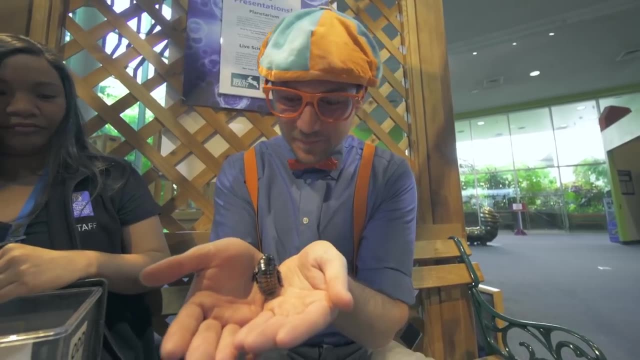 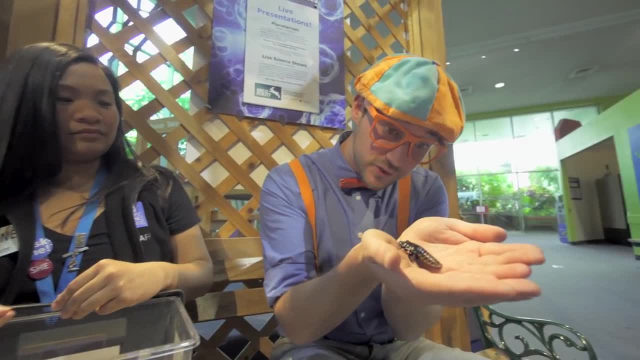 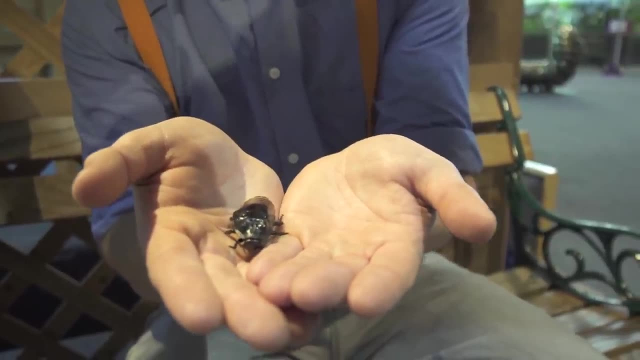 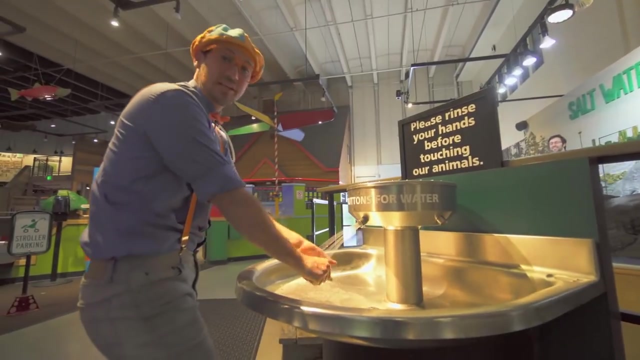 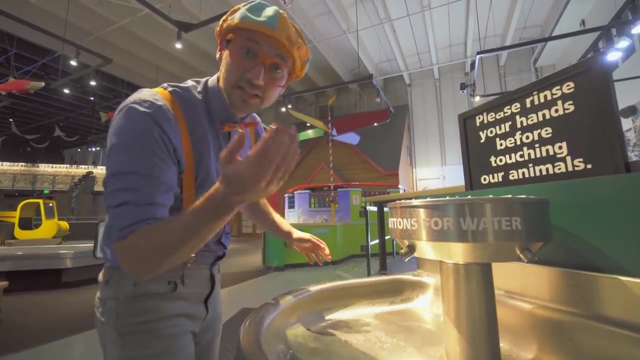 Hey, How are you? What did you do today? Did you enjoy your food? Yeah, Ooh, now we get to touch some animals, But first we need to wash our hands, so then our hands are nice and clean. Okay, I think that's good. 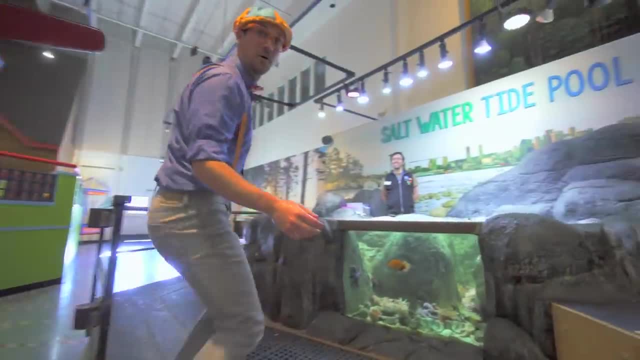 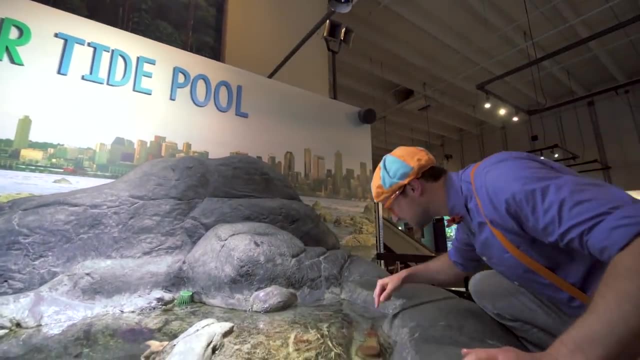 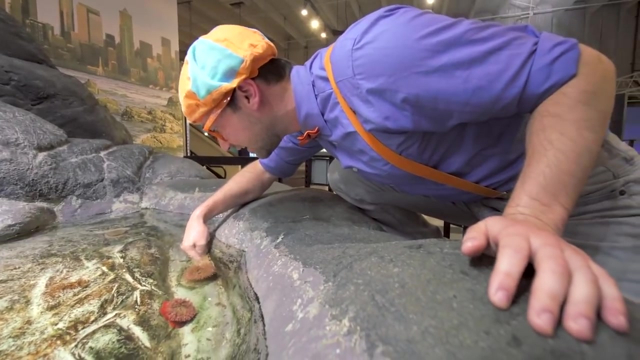 Let's go. Come on. Ooh, look at this. Wow, Okay, what do we have here? Well, over there we have some anemones. They're really friendly and kind of squishy. You're doing a really good job petting it. 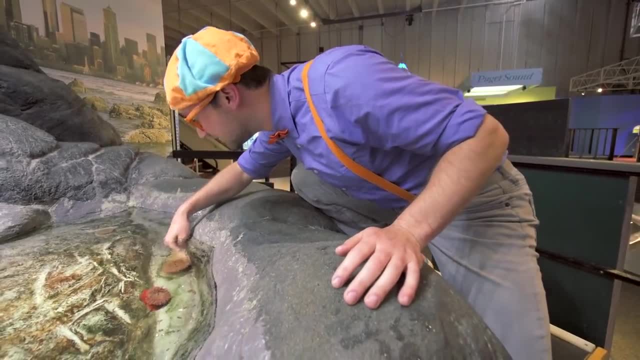 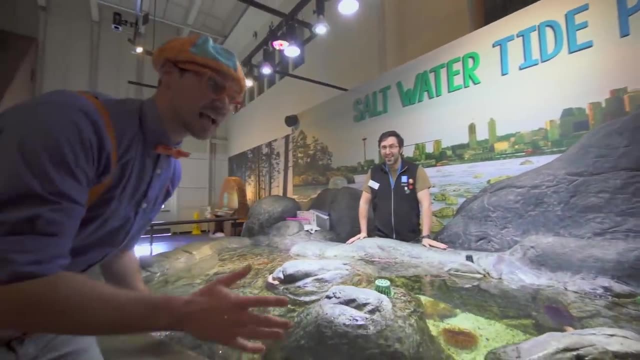 with one or two fingers And then on the side. we don't really want to poke it right in the middle, because that's its mouth. Oh, cool, Ooh, look at this one. So the last one's really soft. 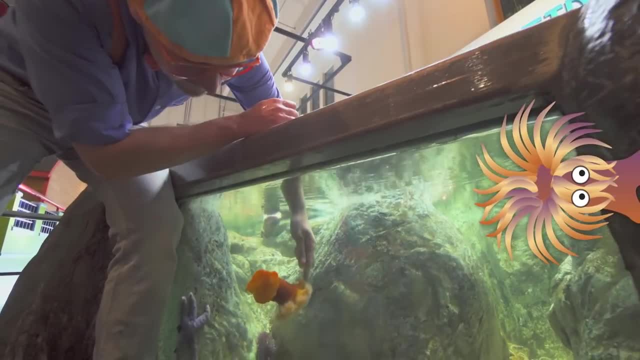 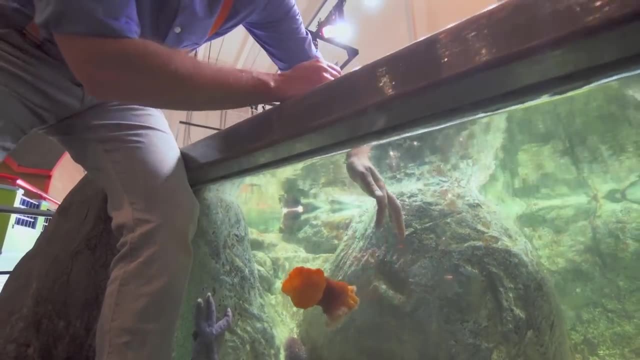 I wonder what this is gonna feel like. Whoa, it looks like it's closing itself up a little bit Blippi. it might think you're food. Ooh, that's funny. Oh, look at this one. What's this? 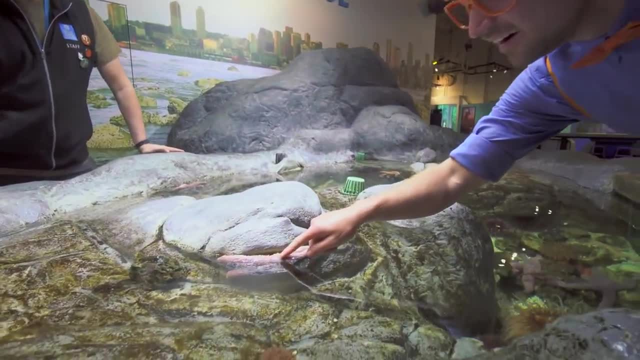 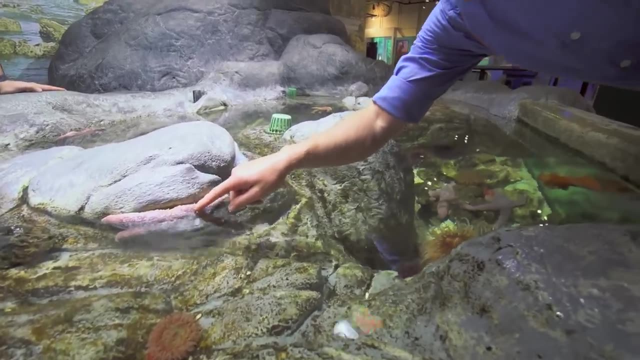 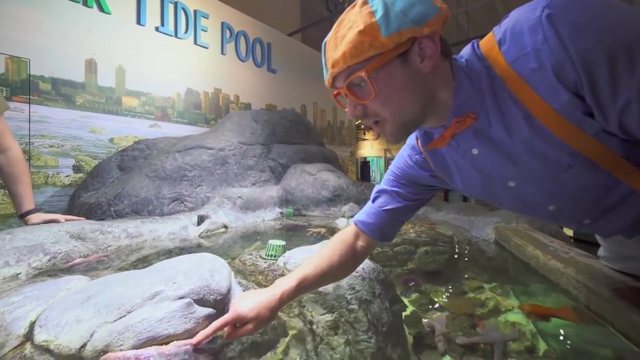 That over there is a sea star. How does it feel? Whoa Kind of bumpy maybe. Yeah, bumpy, and kind of small spikes. The last couple were really soft, but this one is hard. Those little dots are made out of the same stuff. 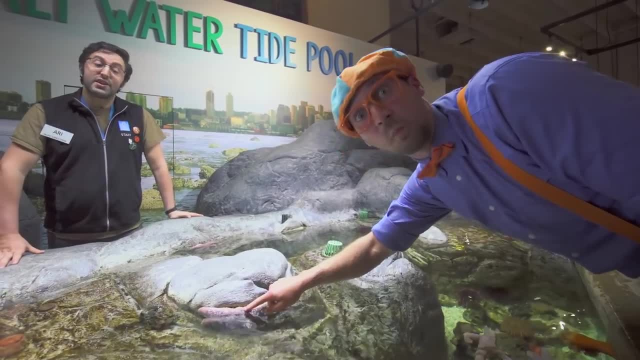 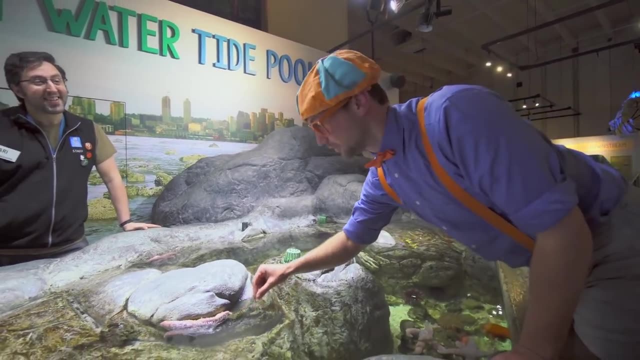 that seashells are made out of. So, even though a sea star doesn't have its own seashell, it's kind of like it has little bits of a seashell. Wow, that's pretty cool. Well, thank you so much. 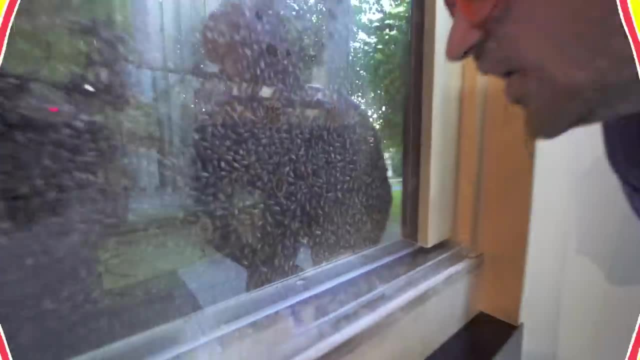 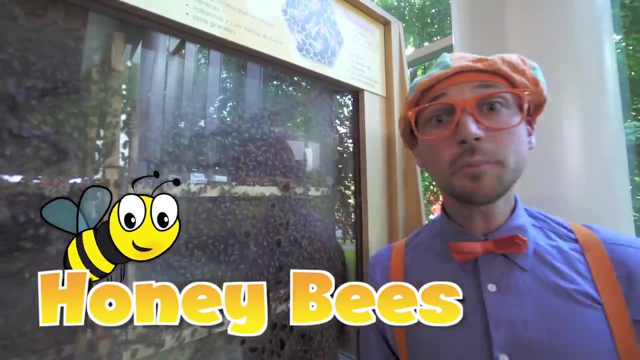 My pleasure, Bye-bye, Bye. Oh, I found the queen. Wow, there's so many honeybees in here. Hey, don't be scared of honeybees. All they're trying to do is make some honey. Yeah. 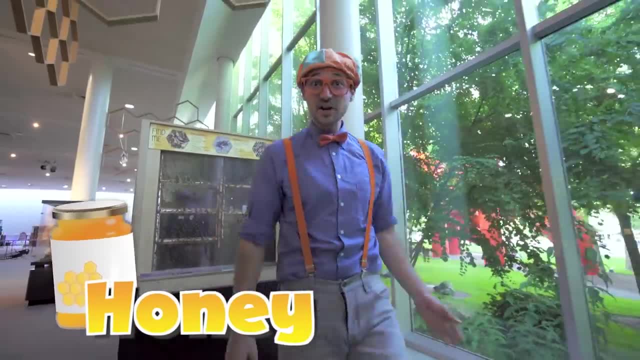 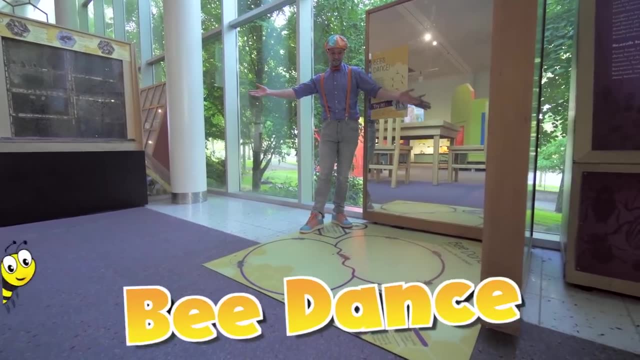 Have you ever had honey before? Yeah, it's so tasty. Look at what it is. This is the spot where you can eat honey. This is the spot where you can do the bee dance. Are you ready to learn the bee dance? 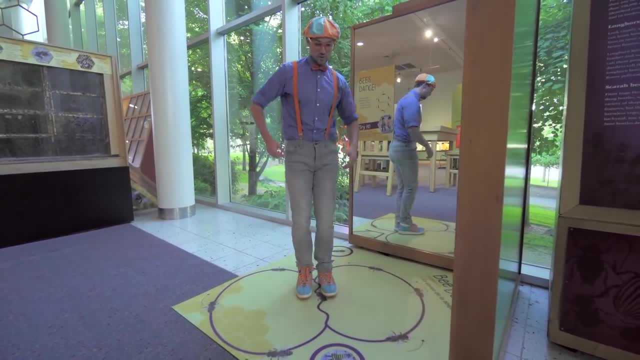 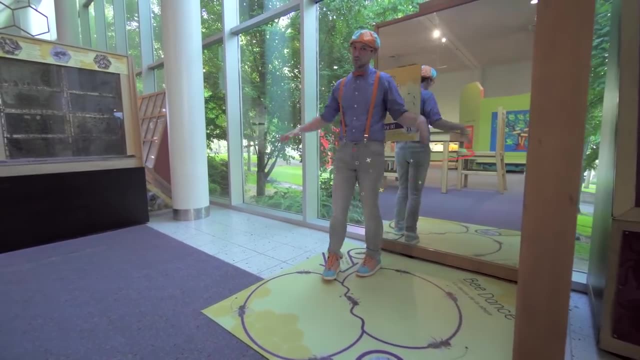 I'll teach you. Okay, in the middle, here you go and do a little wiggle. Then you go this way, flap your wings- Yep, because we want to make some honey. Middle wiggle, wiggle, wiggle. 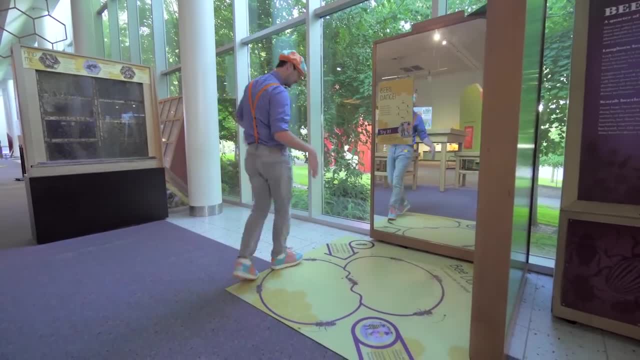 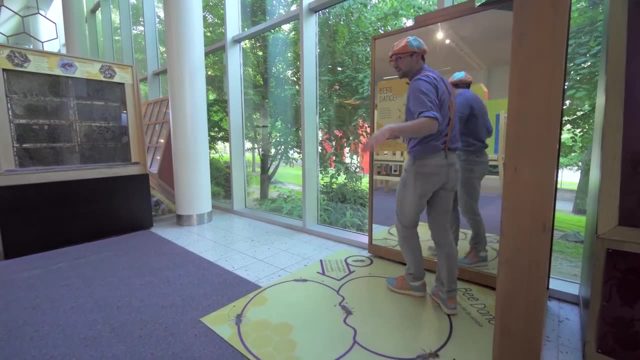 Then go this way, flap your wings And then, since you're back in the middle, you wiggle, wiggle, wiggle and go this way, And then you keep doing it until you're really tired. All right, ready. 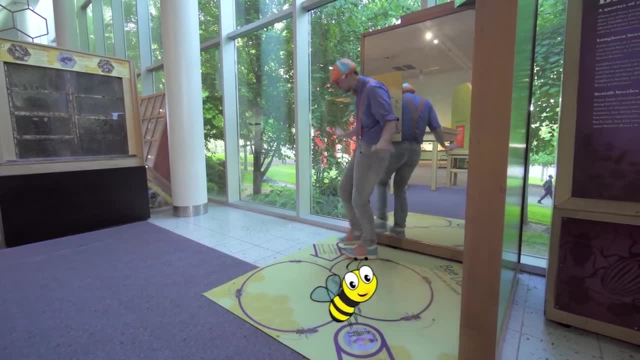 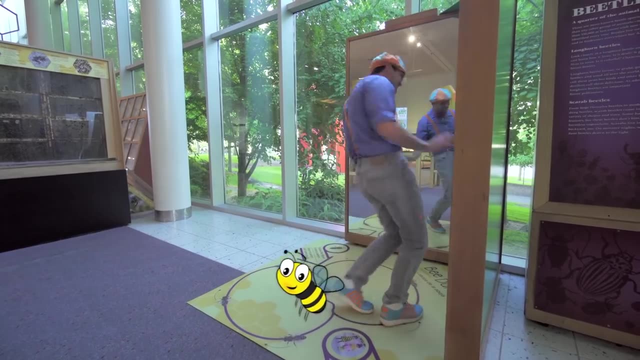 Wiggle, wiggle, wiggle, Flap your wings, Wiggle, wiggle, wiggle, Flap your wings, Wiggle, wiggle, wiggle, Flap your wings, Wiggle, wiggle, wiggle. 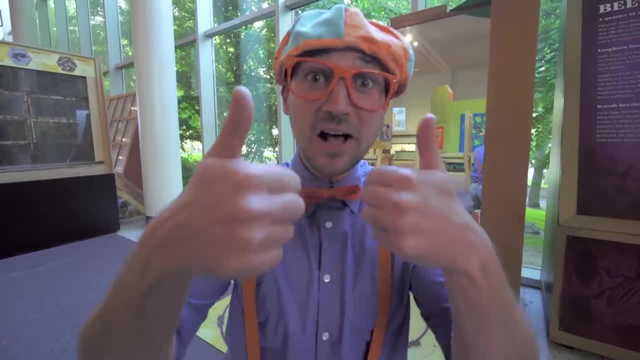 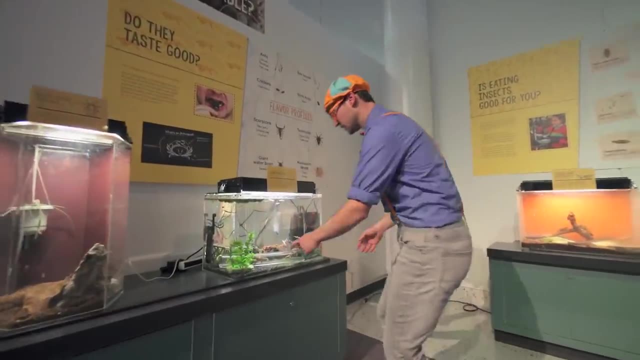 Oh, I'm tired. Oh, that was awesome, Good job, Good job. Oh, now we're in the Living Things exhibit. Oh look, Hey, look at what it is. It's a crayfish. Do you see it right there? 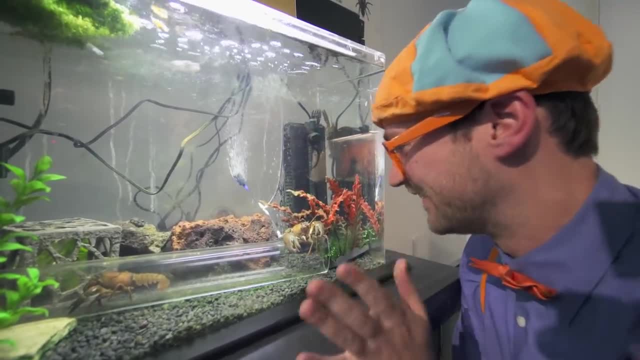 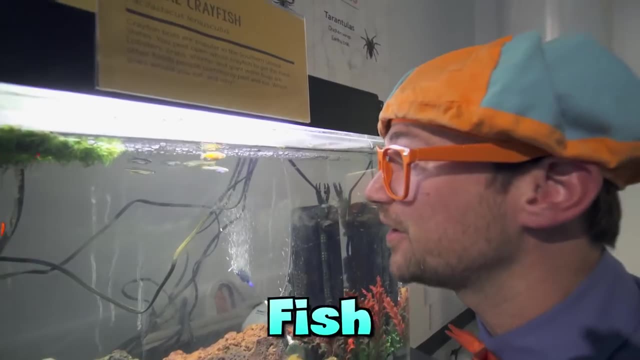 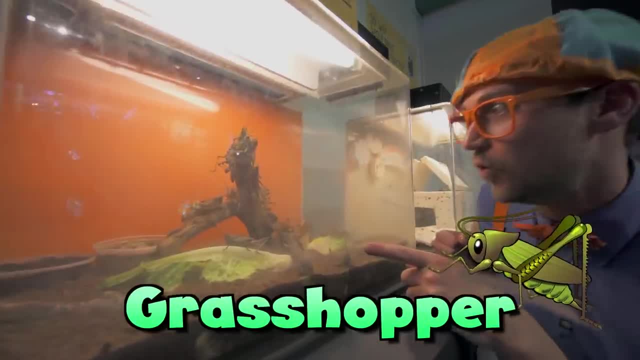 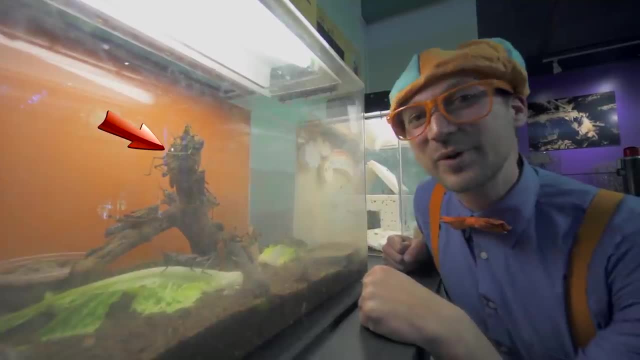 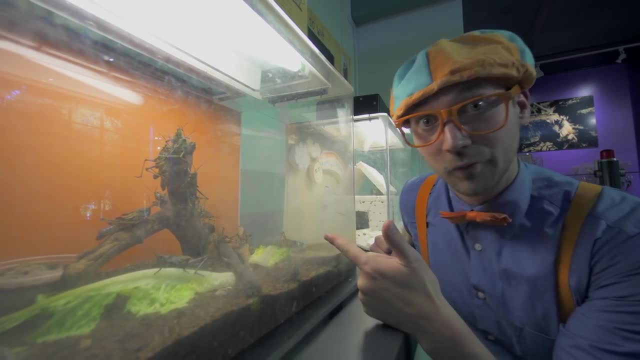 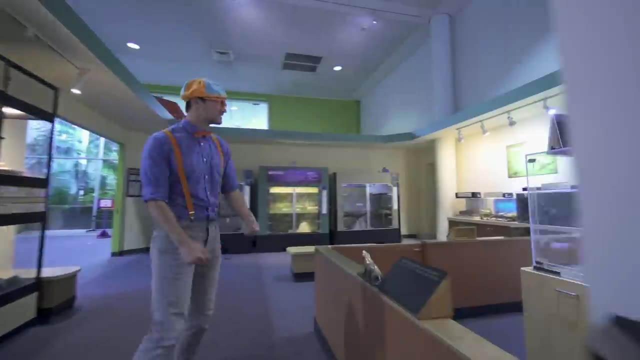 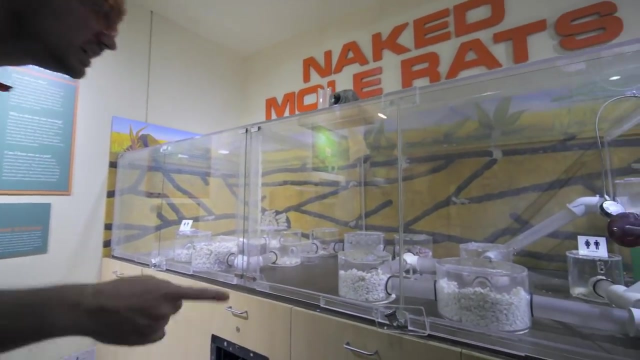 Lot of times they live in the grass and they hop really high. Let's go see what else there is. Whoa, look at this room, Another part of the Living Things exhibit. Whoa, Whoa, yeah, do you see these? 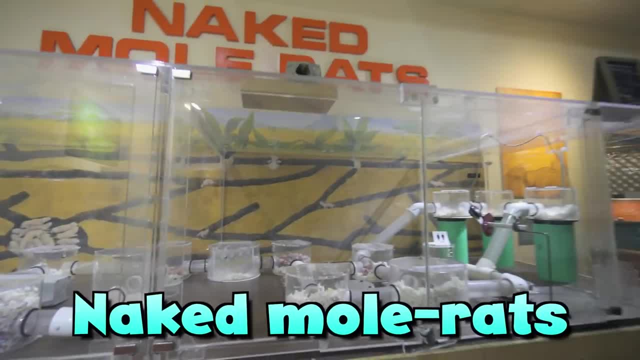 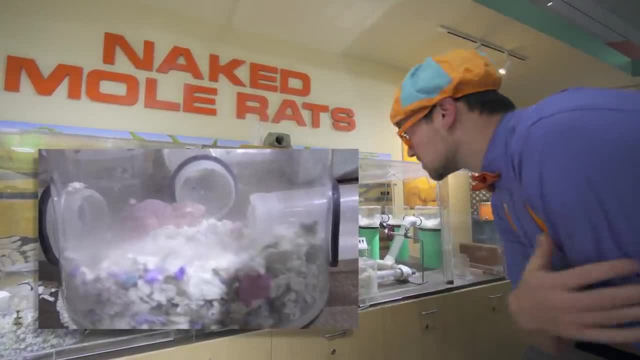 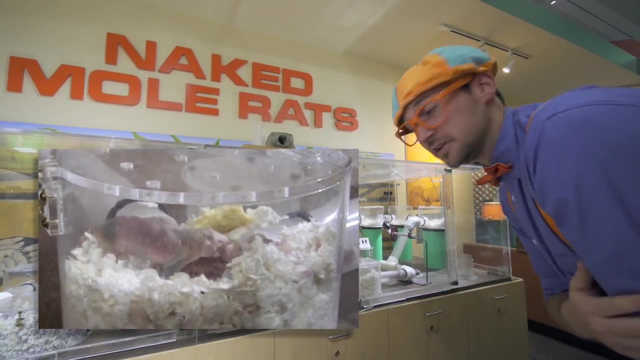 Whoa interesting. These are naked mole rats. Wow, They're like rats, but they have no fur or hair or scales or anything like that. That's why they're called naked mole rats. Oh, and an axolotl. 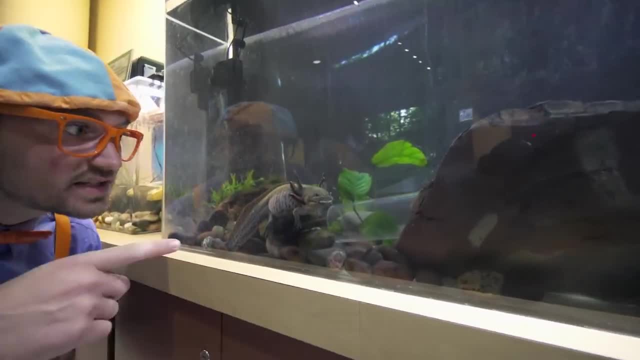 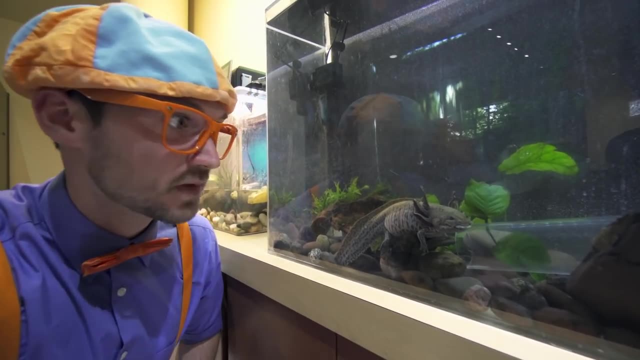 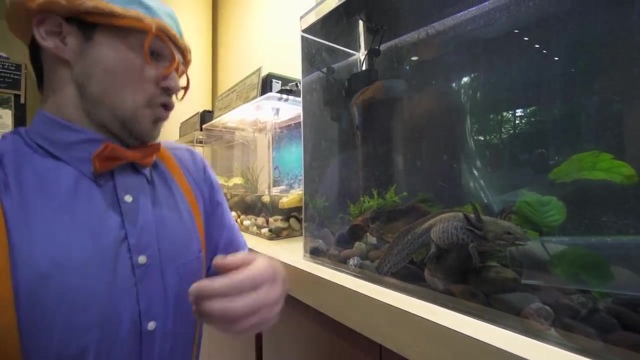 Check this out. Whoa, See that That's an axolotl. Whoa so interesting. Kind of looks like a salamander mixed with a fish. But the cool thing about axolotls are if they lose a limb like their arm. 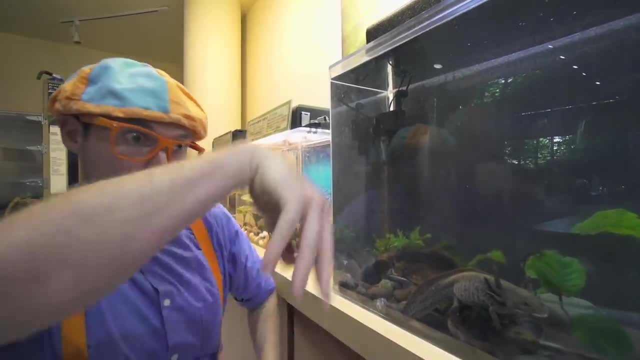 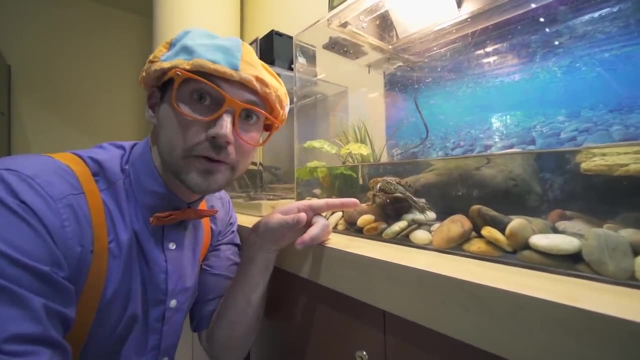 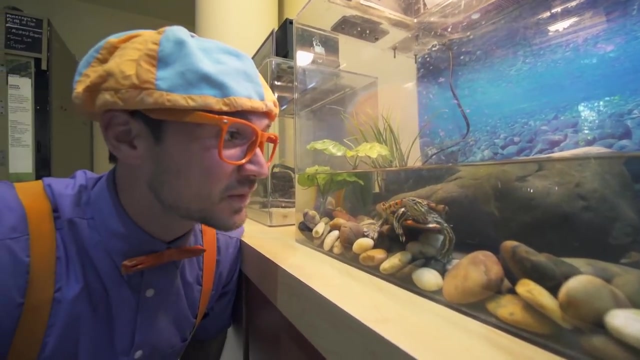 then from there they can regrow it back. Whoa, Whoa, Whoa. Check out this little person, or guy or girl, or I don't even know, but this is a turtle. Wow, Hey, how are you turtle? 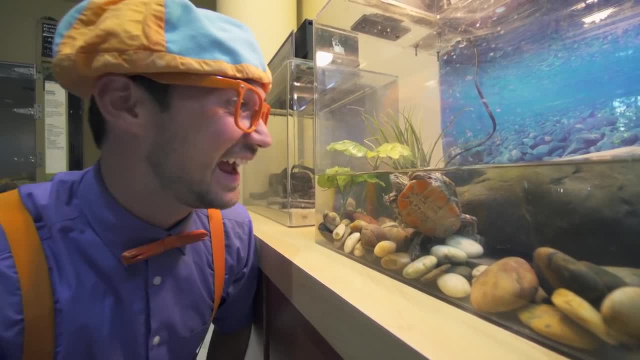 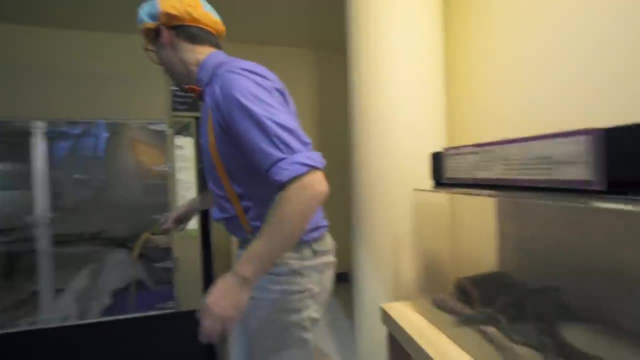 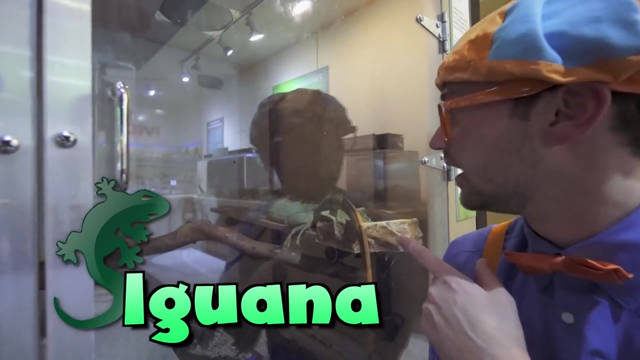 Are you having a good day? Are you having fun? Yeah, You sure do. look like you're having fun. See you later. Whoa, It's kind of dark in here, but that's okay. This is a green iguana. 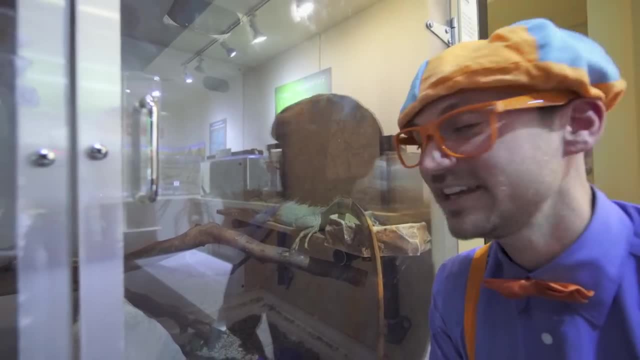 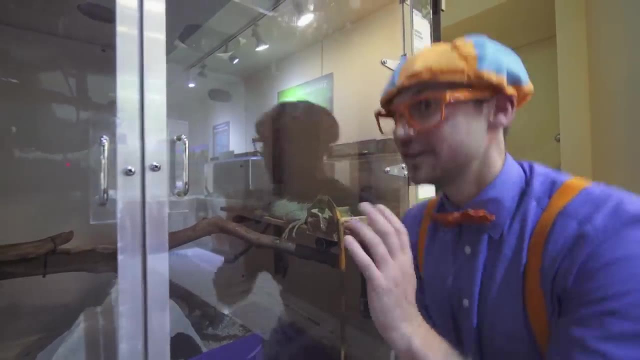 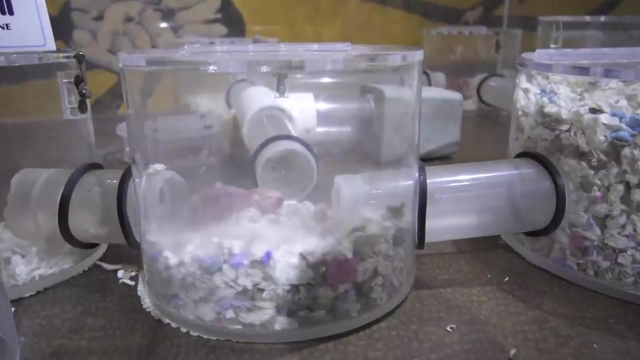 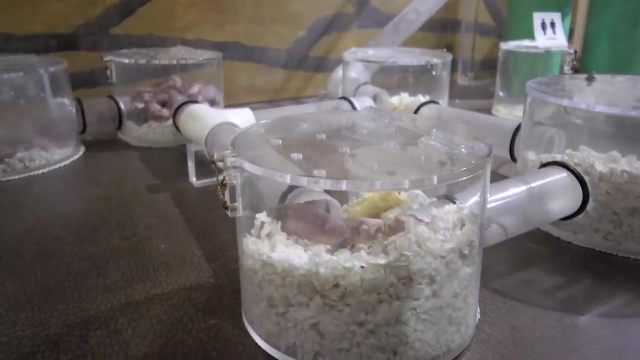 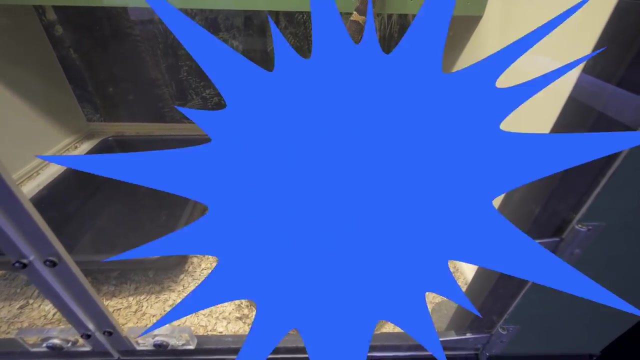 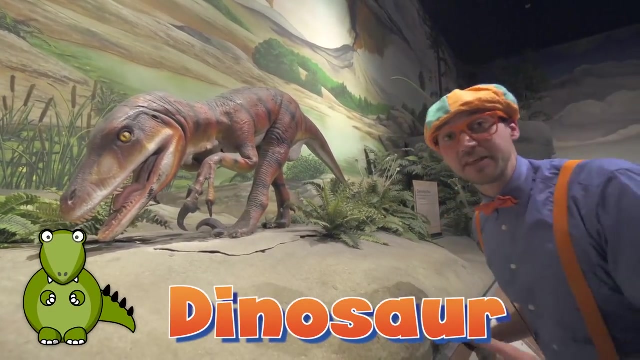 Can you see it, Whoa? It's just relaxing, Having a good time. All right, See you, iguana. Whoa, Check that out. That right there is a dinosaur. That right there is a dinosaur. They don't live on our planet anymore. 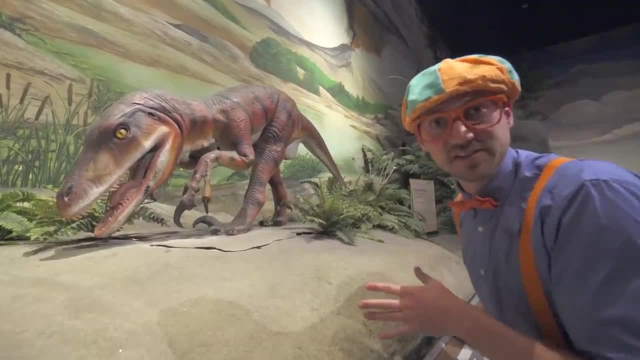 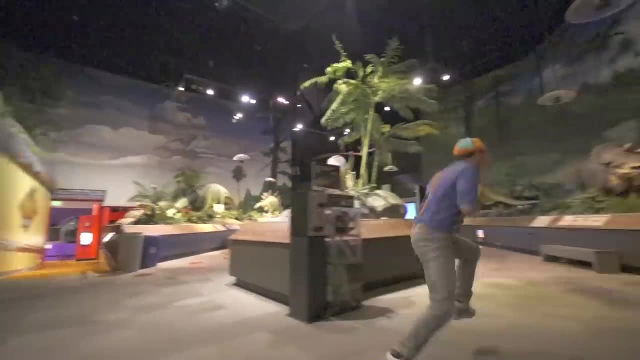 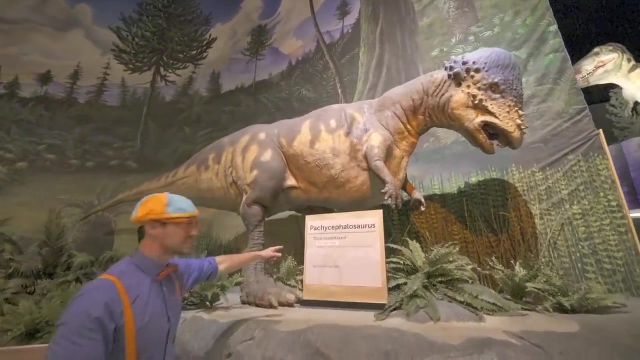 but they used to Look at it. It kind of looks like a velociraptor. Will you act like a velociraptor with me? Whoa, Another dinosaur. Whoa, This dinosaur- that's its name- right there, It's really big. 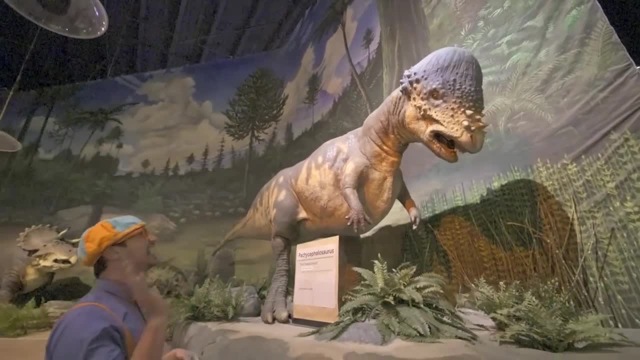 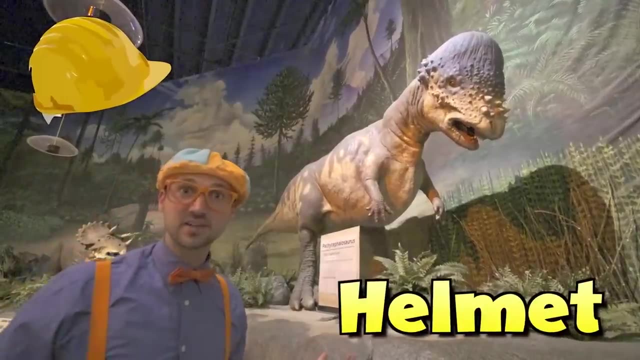 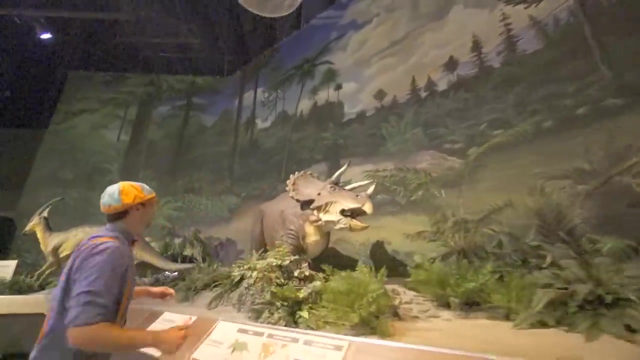 Hey, look at its head. Hey, Hey See. it kind of looks like it's wearing a helmet, Just like when you and I ride bicycles, we wear helmets, Cool. Oh, here's some more dinosaurs. Whoa, look at that one. 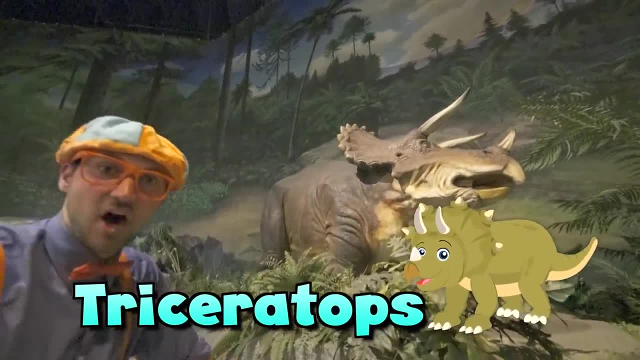 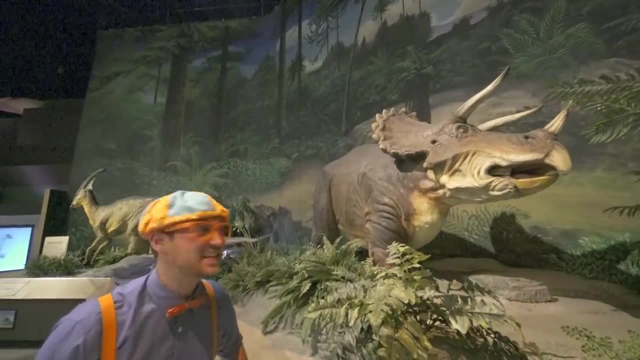 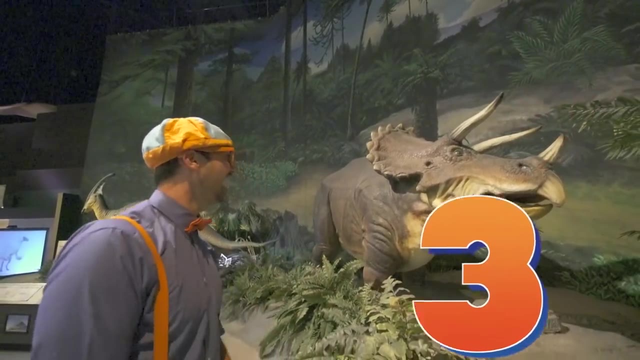 That is a triceratops. Do you know why they call it a triceratops? Yep, because it has three horns on its face and head. Let's count them One, two, three. All right, See you later, triceratops. 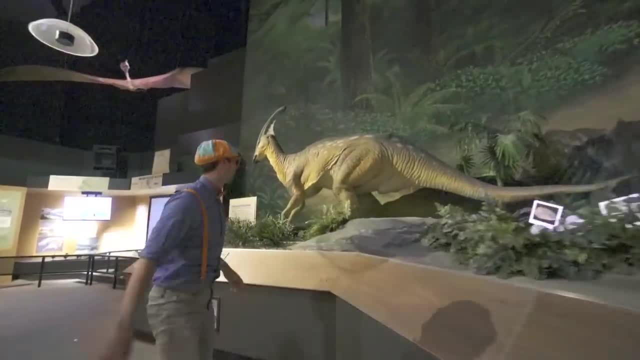 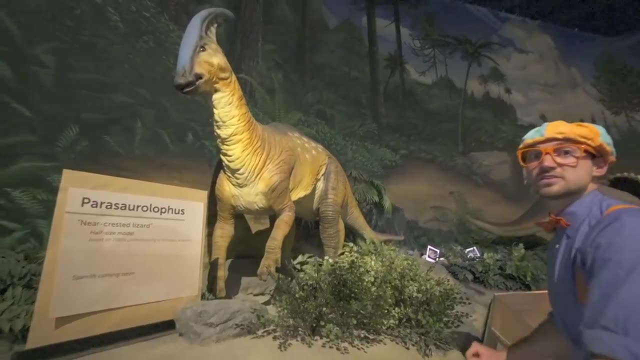 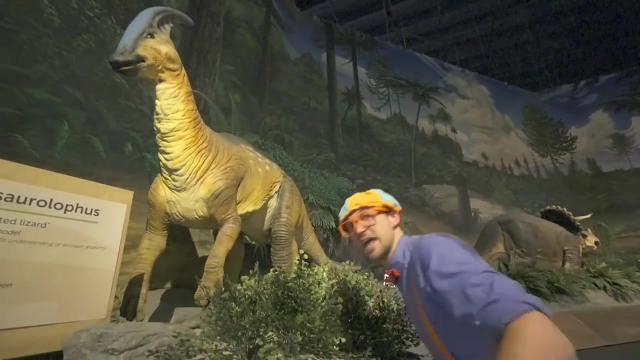 Whoa, Hey, another dinosaur, Wow, Hey, dinosaur. Oh, this dinosaur right here was a herbivore. See these plants. That means it eats plants And plants, only It doesn't eat meat. It doesn't eat meat And plants, only It doesn't eat meat. 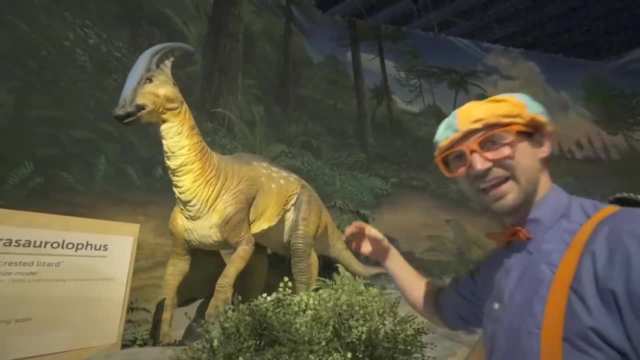 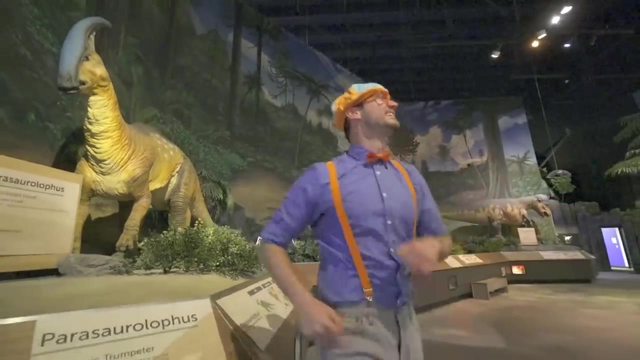 It doesn't eat meat And plants. only It doesn't eat meat And plants, only It doesn't eat meat. And look at what's on its head. It kind of looks like a shark fin. So silly Whoa, check this out. 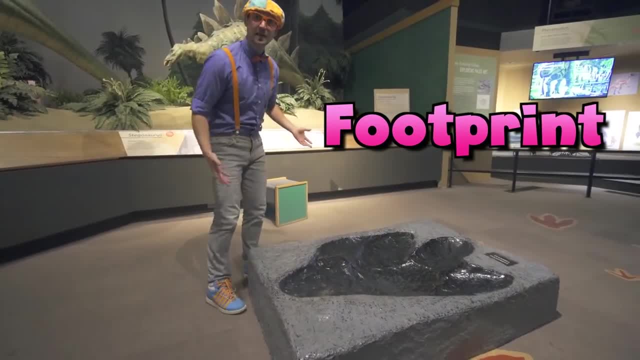 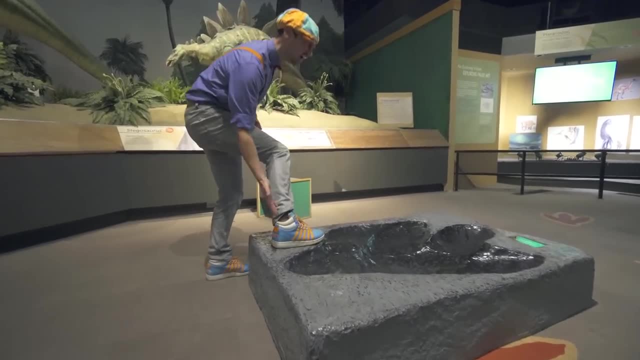 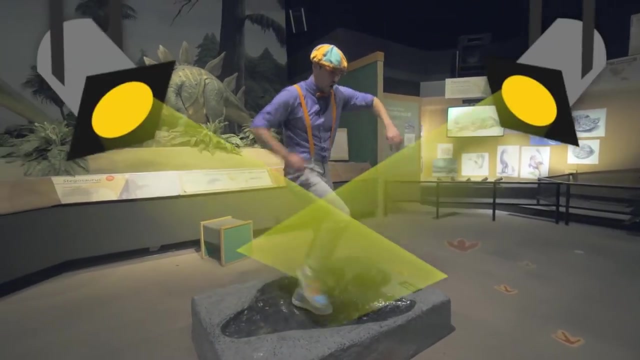 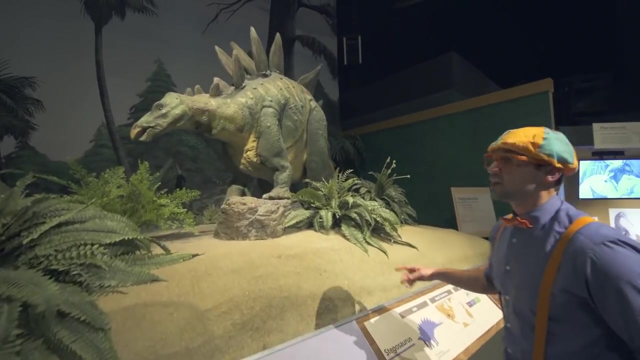 Whoa, this is a massive footprint. Okay, let's compare my foot to this dinosaur's foot Ready. Its foot is way bigger than mine. It's even way bigger than two of my feet. Whoa, another dino. Check it out. 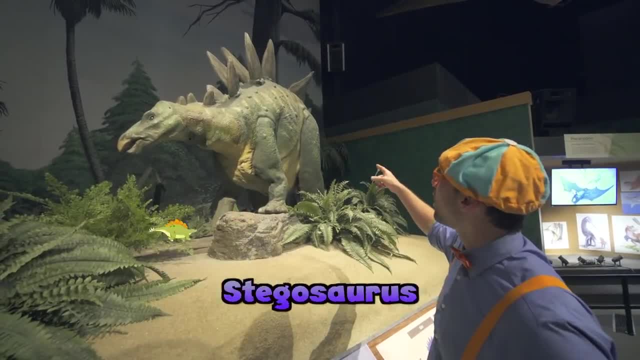 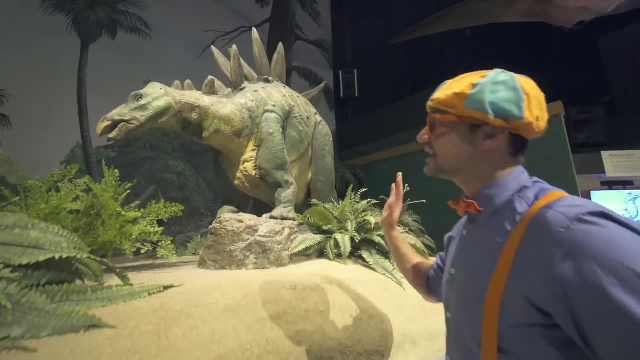 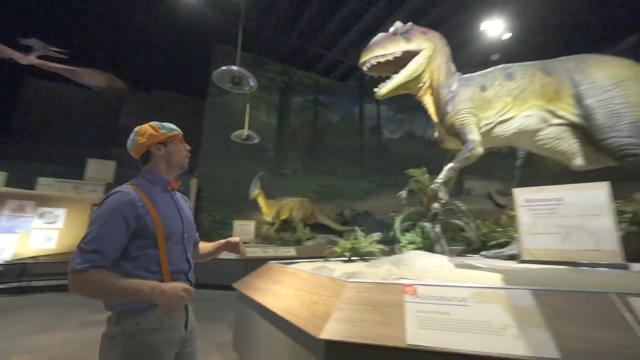 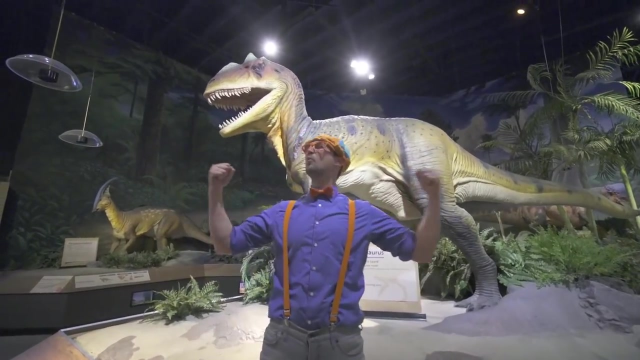 This is a stegosaurus. Whoa, Do you see those plates on its back? That's for its defense mechanism. Wow, Hey, stegosaurus. So many cool dinosaurs in here. Whoa, this dinosaur is so scary. it's the king and queen of the dino land. I'm gonna act. 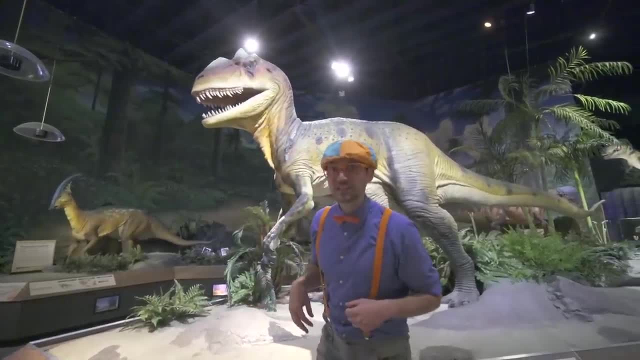 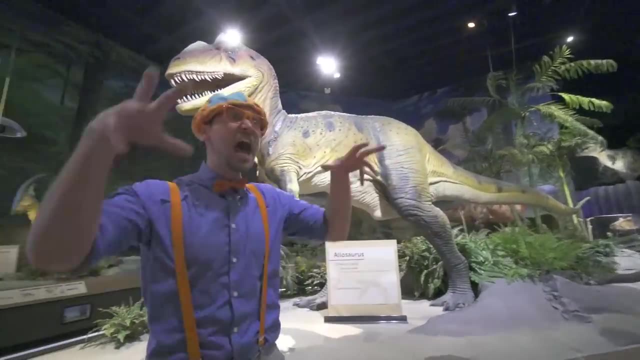 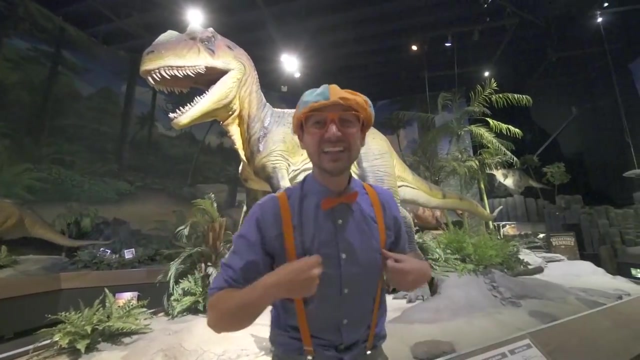 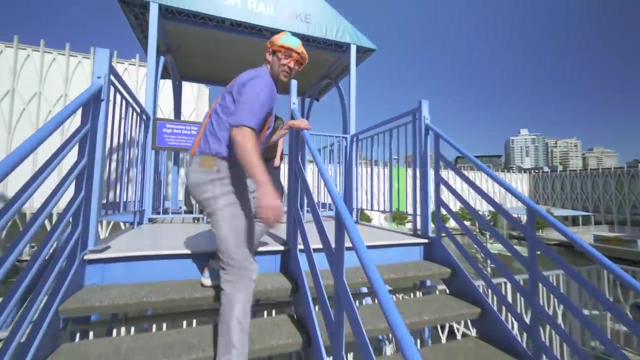 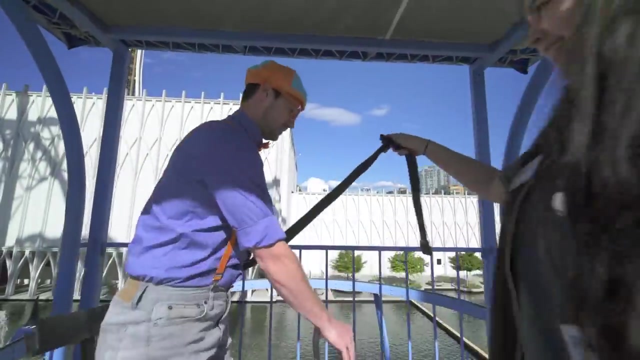 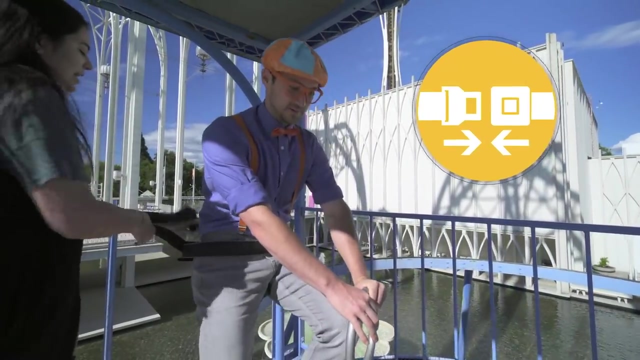 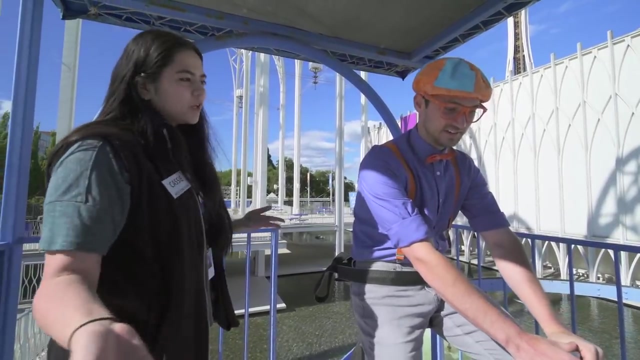 like this dinosaur. okay, will you do the same? ready, I love acting like a dinosaur. now we're gonna do the high-rise fight. all right, gotta buckle up, whoa. before you go, okay, just make sure you're going at like a walking pace. you're always going forward and just keep cuddling the whole time, okay, hands. 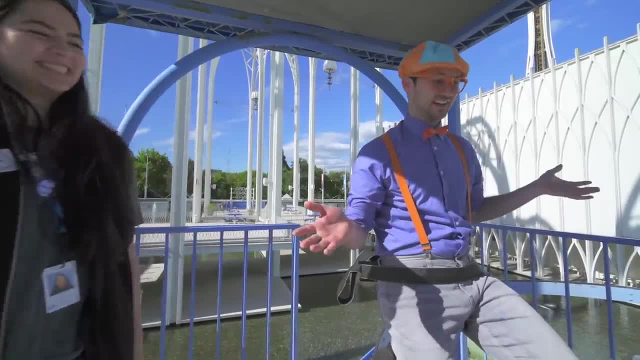 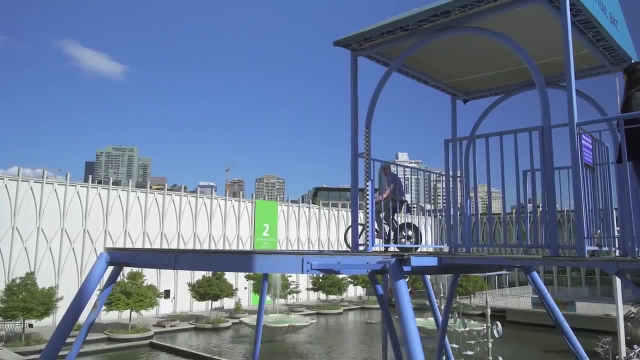 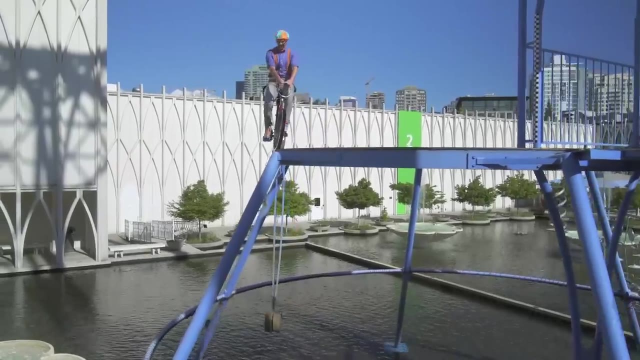 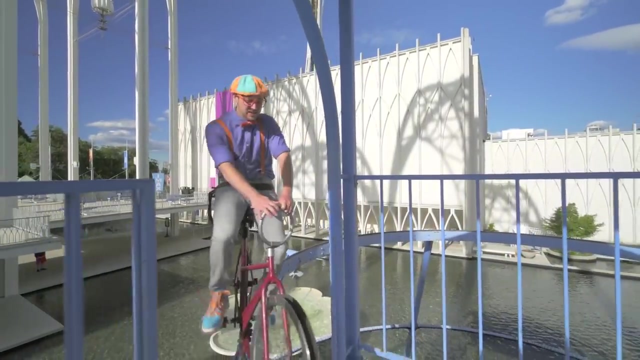 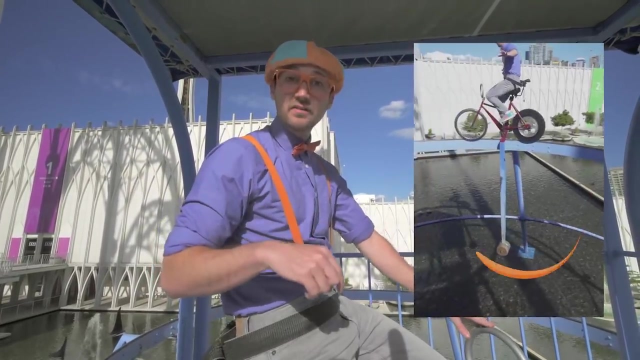 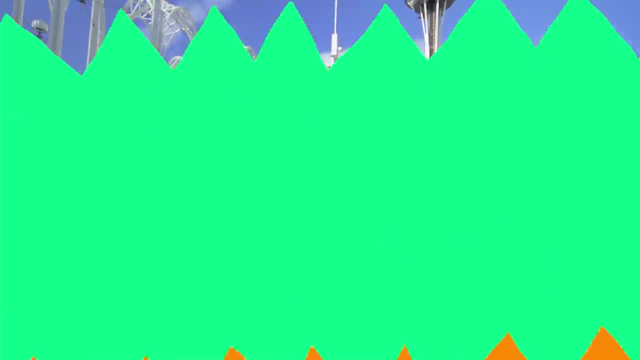 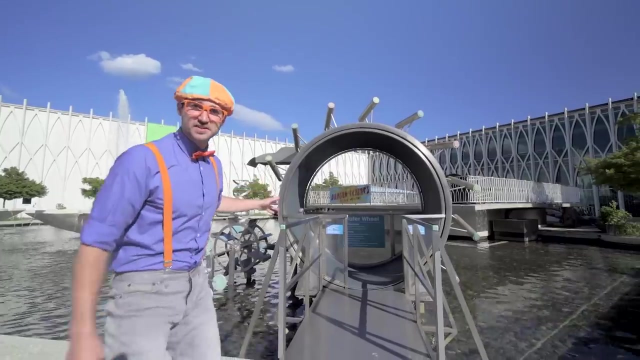 are optional. whoa, hands are optional. here I go. did you see that? you would think I would fall off because it's a really thin rail? but I didn't, because the weight is really heavy and it's really far away from me. here I go. Oh, whoa, look at this interesting. this looks like a giant circle and this is. 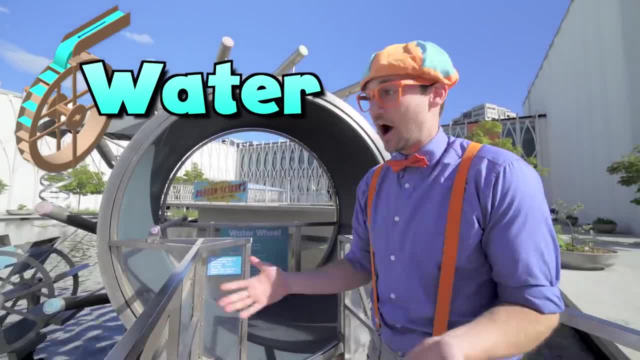 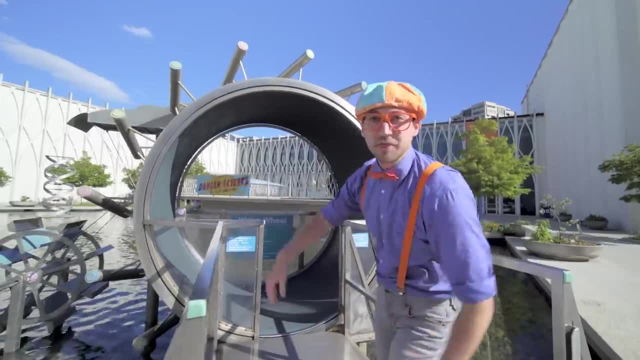 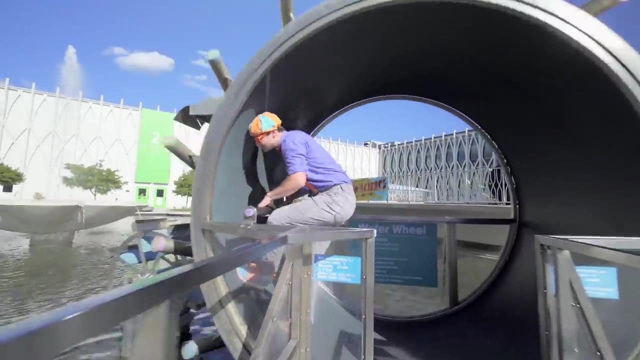 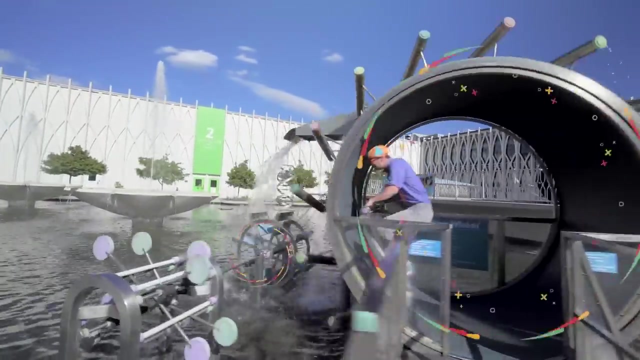 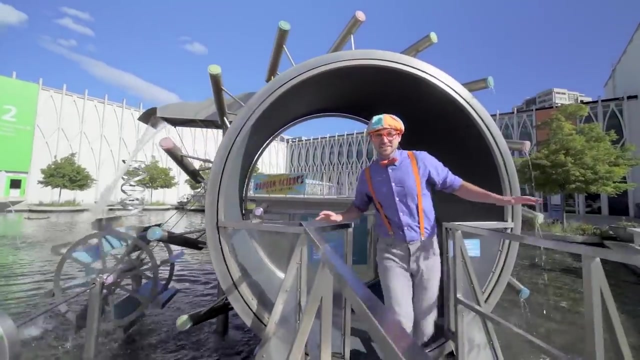 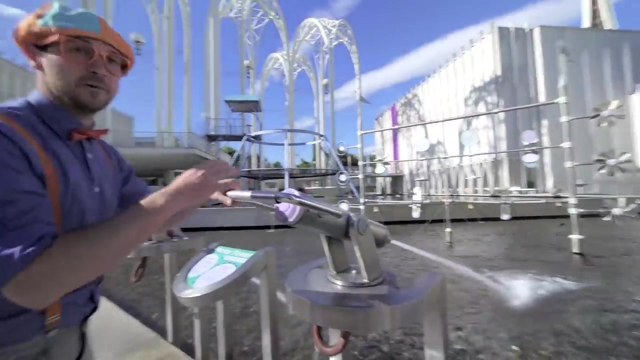 actually called the water wheel. it's kind of just like how a hamster runs in their wheel. I'm gonna do the same, but it's gonna grab water from the bottom and throw it up over the top. ready, here I go. whoa, did you see that? that was awesome? whoa, what's this? 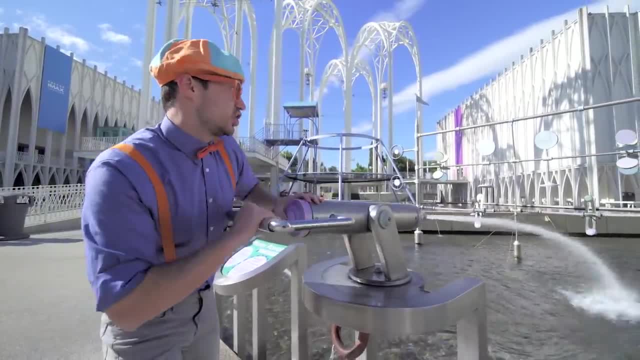 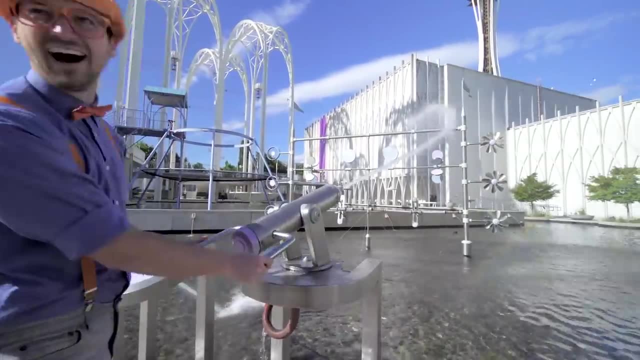 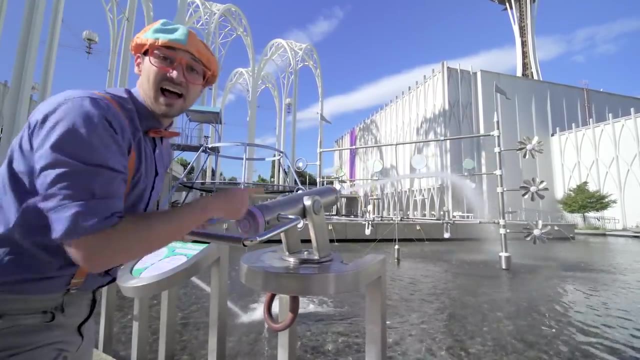 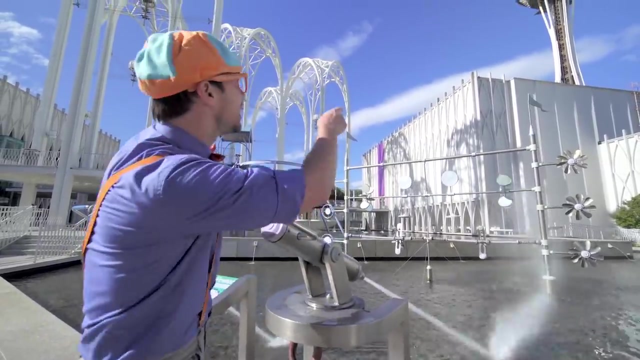 whoa. this is the water power station. water is getting shot out on the front of this little water gun. whoa, okay, whoa. wow Watch, I'll make that spin. Yeah, we're doing it. Whoa, Okay, whoa. what's that way up there? 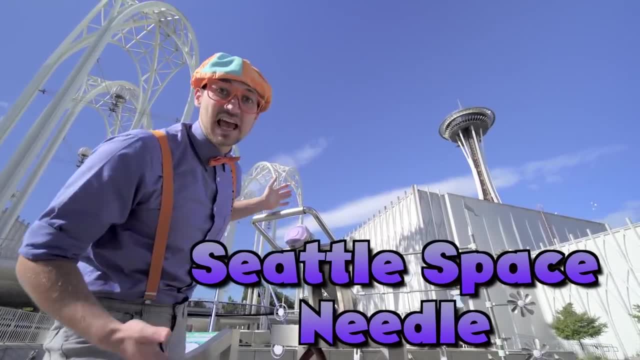 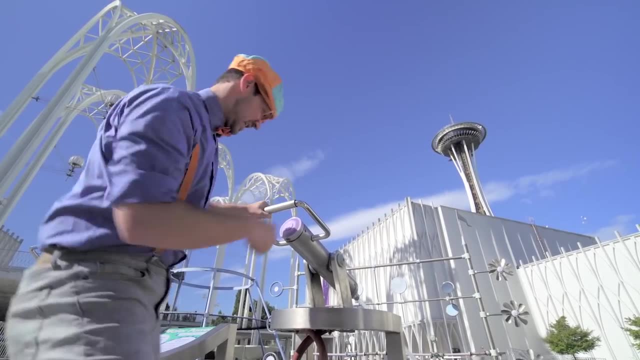 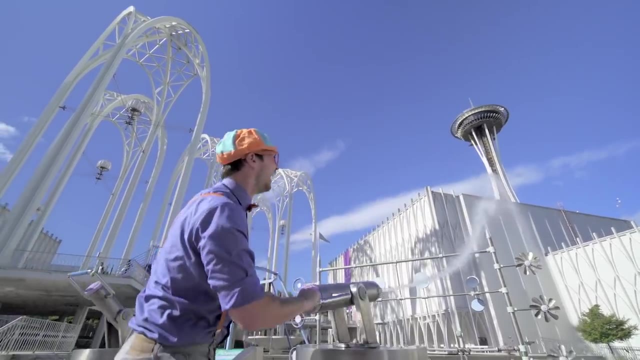 Do you see that? Yeah, that's the Seattle Space Needle. I think we should take the water power gun and try and shoot way up there. Here we go. Whoa, it's such a nice day, I wanted to give them a cool break of water. 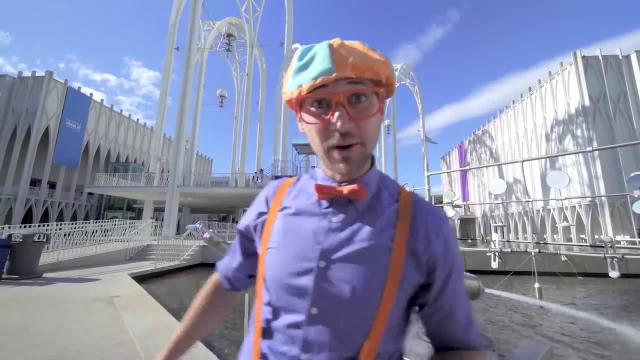 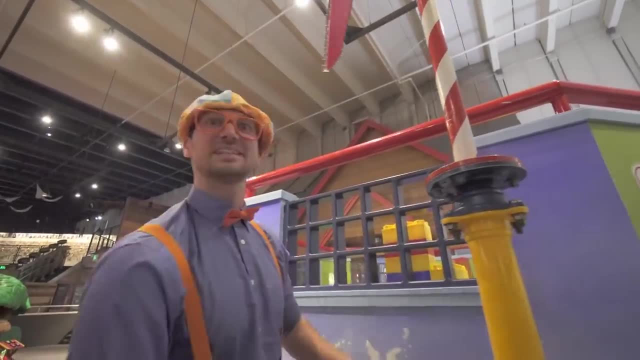 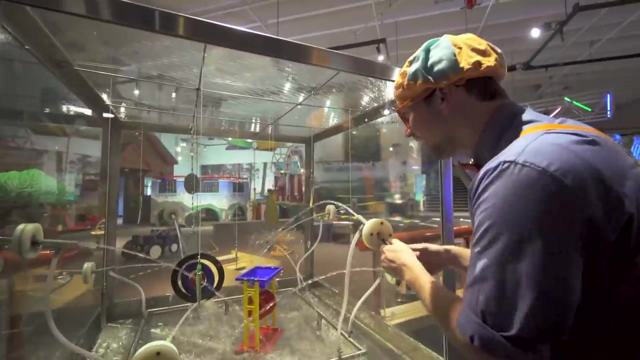 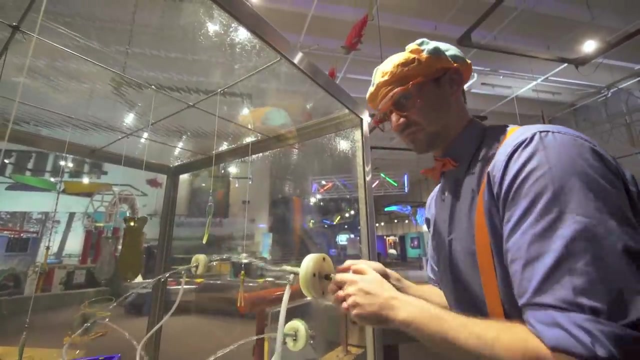 but it's too high up there. Let's go see what else there is around here. Whoa, that's pretty fun. Whoa, look at this area. You can use these water squirters to squirt inside there. Isn't this a clear cube? 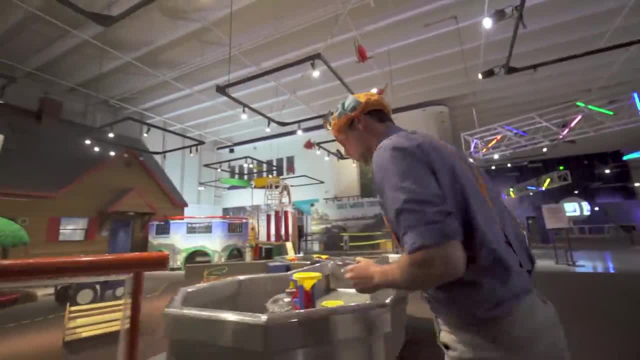 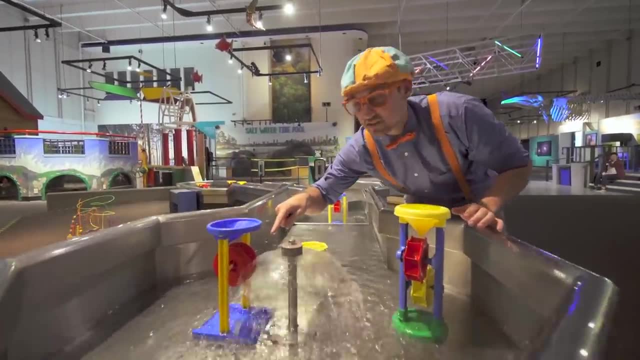 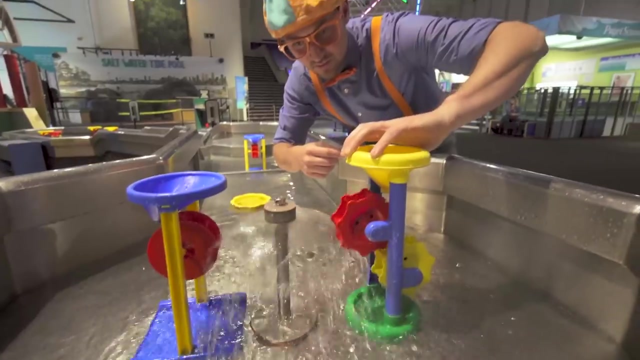 All right, let's see what else there is. Whoa, look at this. All right, I wonder if I put this right here. Yeah, see, The water is pushing this gear around. Okay, let's try this one. Whoa, look. 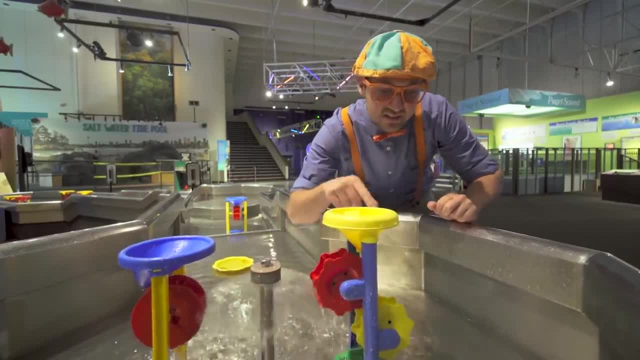 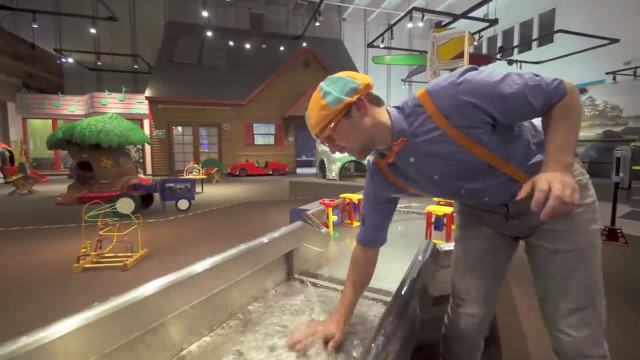 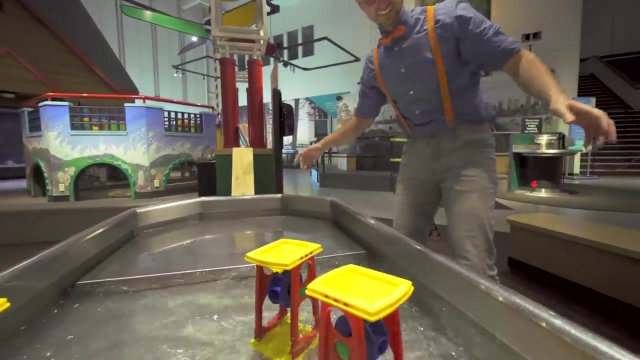 Both of these are going in circle, The red one and the yellow one. Come on, Come on. I love playing with water. Whee, Okay, Whoa, Wow, Okay, look in there, Let's go. Whoo. 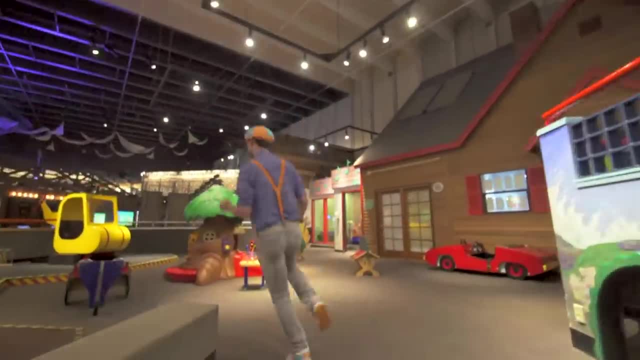 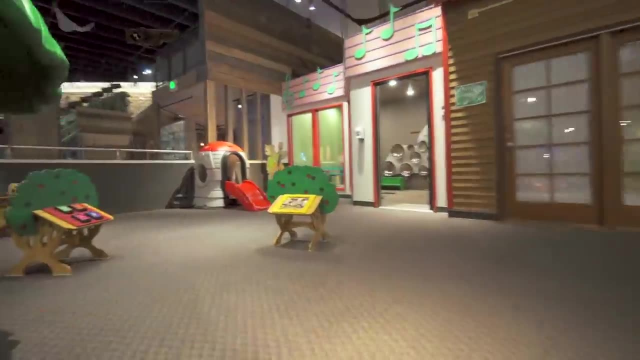 Welcome, Come on in. Hey look, It's a little tree house, Here I go. Hey look, It's a little tree house, Here I go. Hey look, It's a little tree house, Here I go. 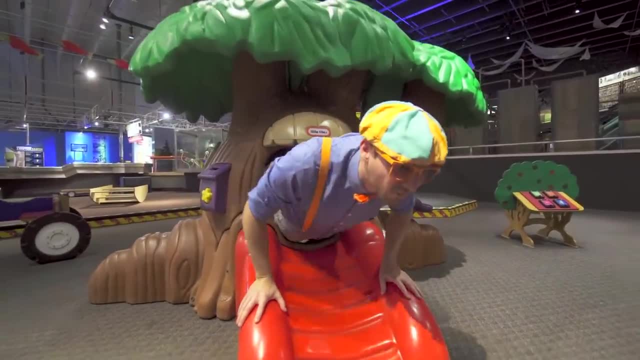 Here I go. Whoa, Whoa, Whoa. look at this, It's a bunch of spirals, ups, downs, lefts and rights. Here we go. Whee, Whoa, Whoo, Whoa. 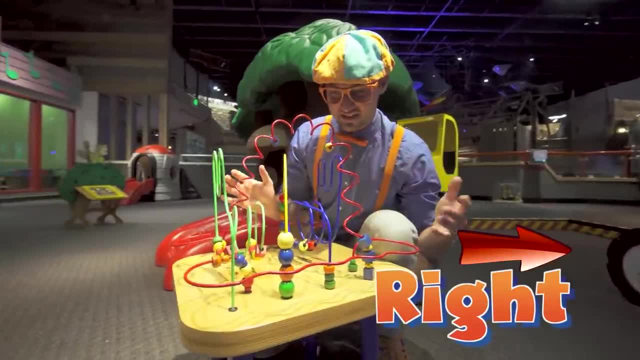 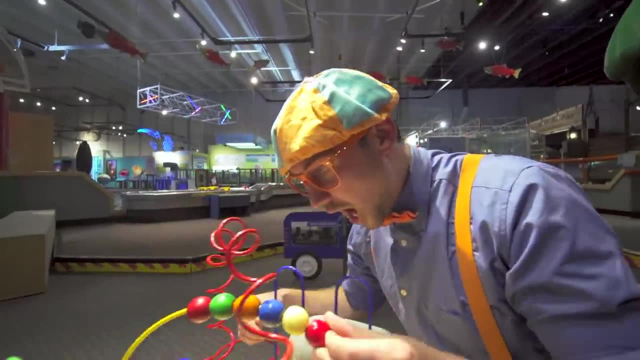 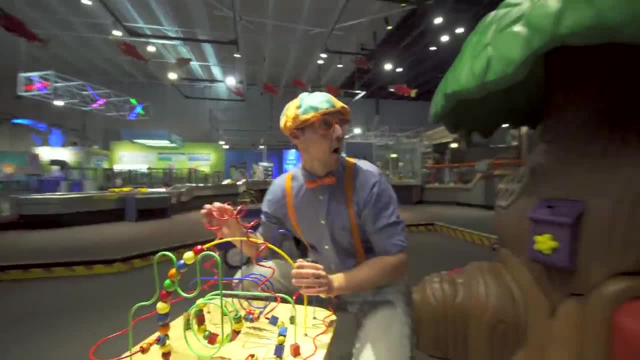 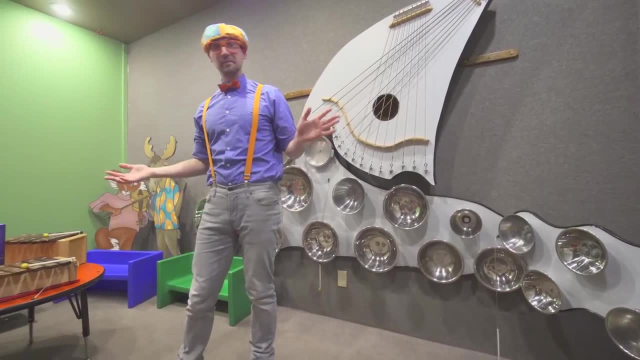 Whoa, Whoa, Whoa, Whoa, Whoa. The noise room. Come on, Whoa. This room is a room that you can make as much noise as you want. First thing I'm going to do is yell. 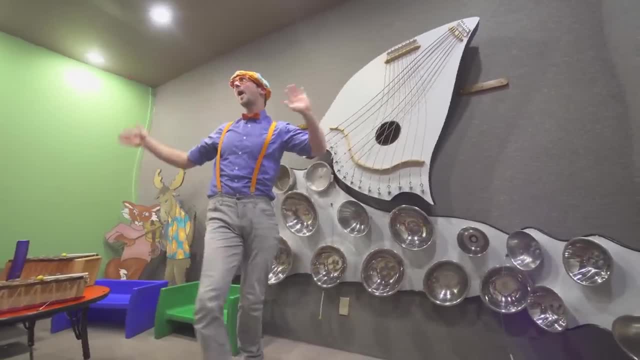 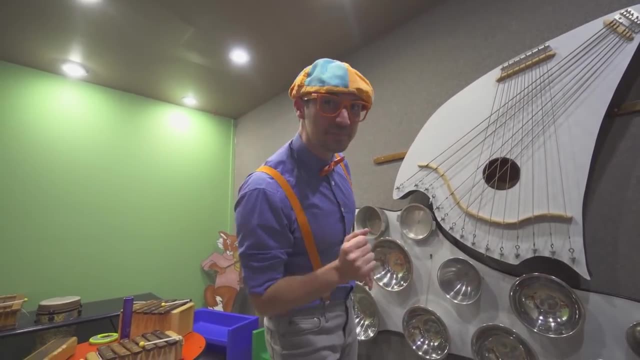 Whoa, Whoa, Whoa, Whoa, Whoa. Now let's use the things around us to make some noise and, if we're lucky, maybe it will sound like music. Whoa, Whoa, Whoa. 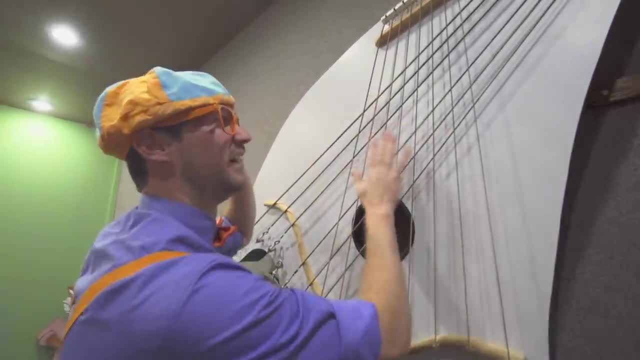 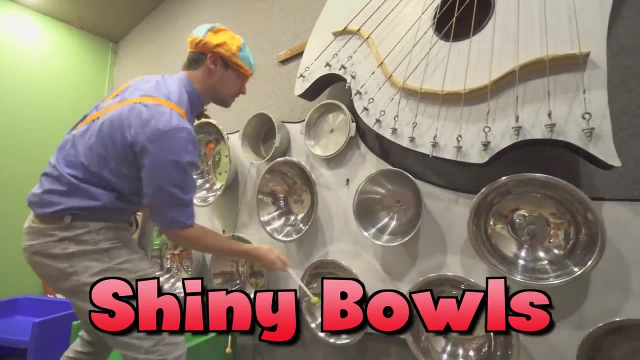 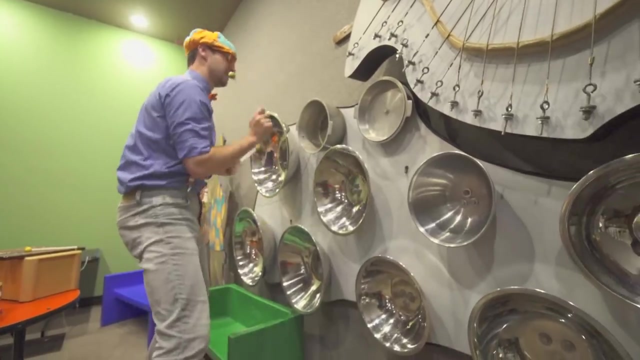 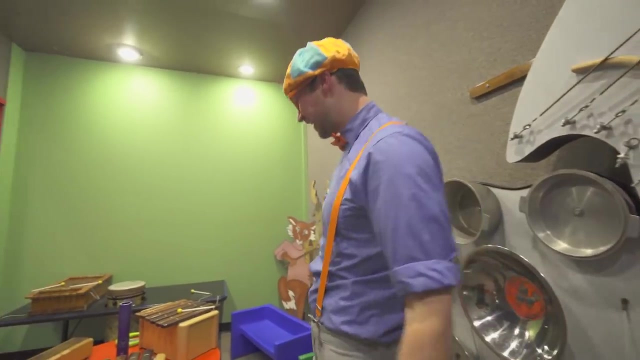 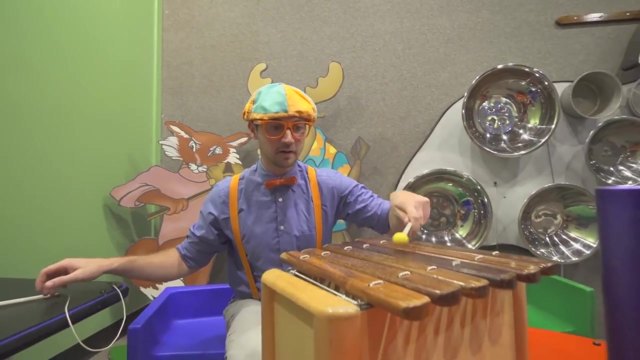 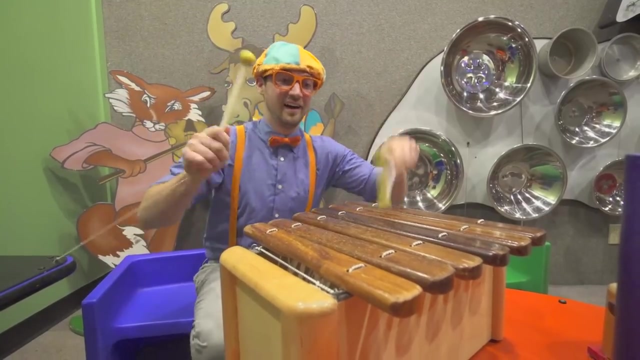 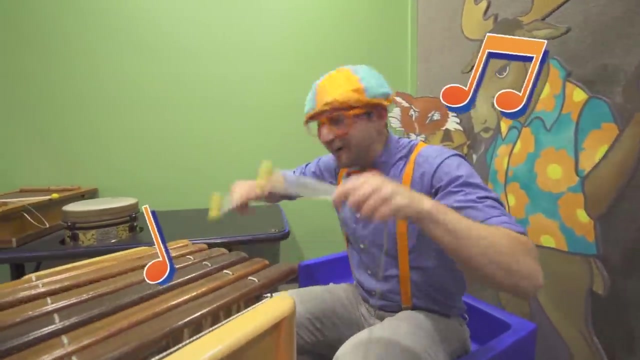 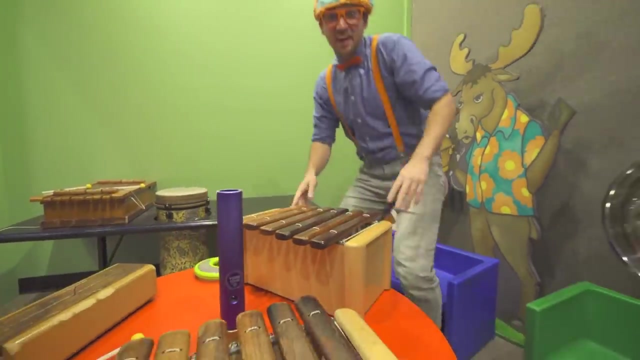 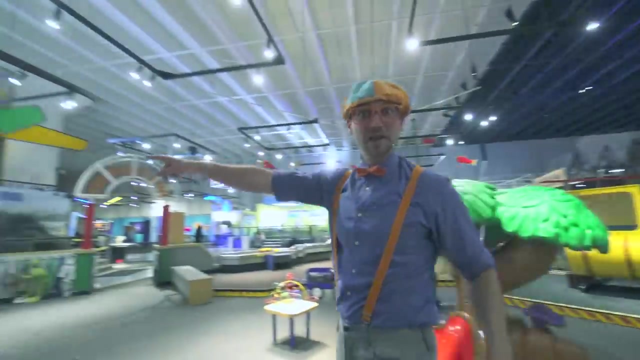 Whoa, Whoa. Oh, look some shiny bowls. Oh, I'm pretty good, huh? Oh yeah, Check it out, Listen. Okay, enough music for now. Let's go back outside here. Ooh, let's go to the top, right up here. 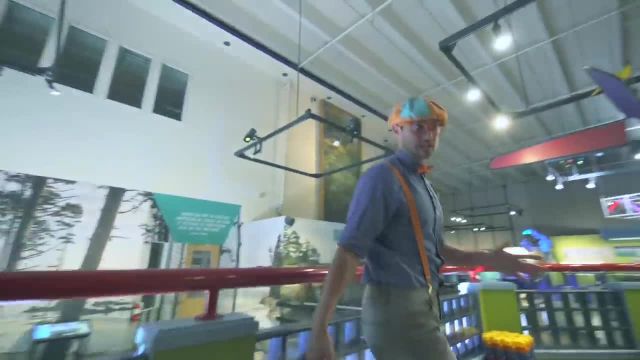 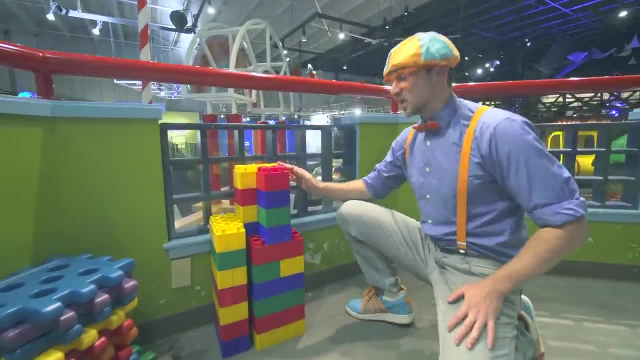 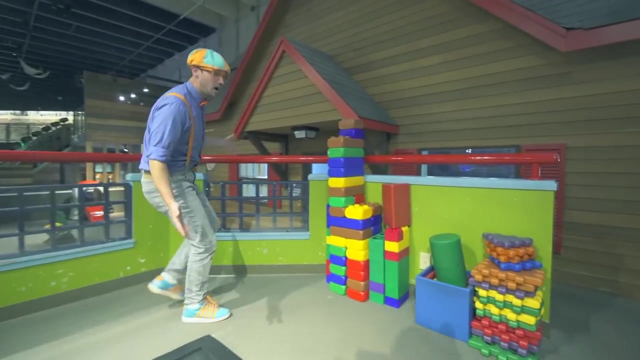 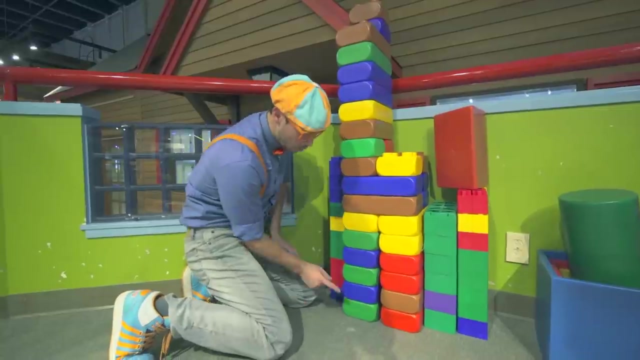 Whoa, this area has a lot of colorful bricks. Yeah, see Right over here. All right, Timber. Whoa, a taller one, Let's count how many there are. This is a lot of stories of bricks. One, two, three, four, five, six, seven, eight, nine. 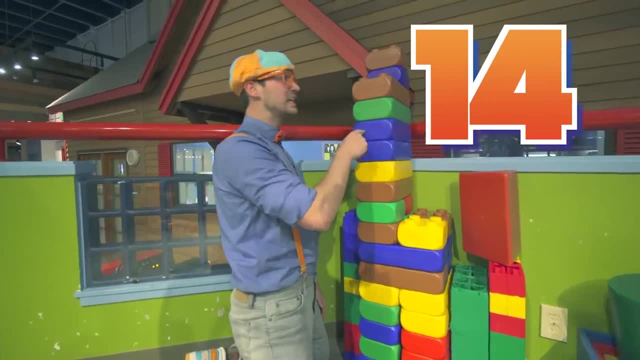 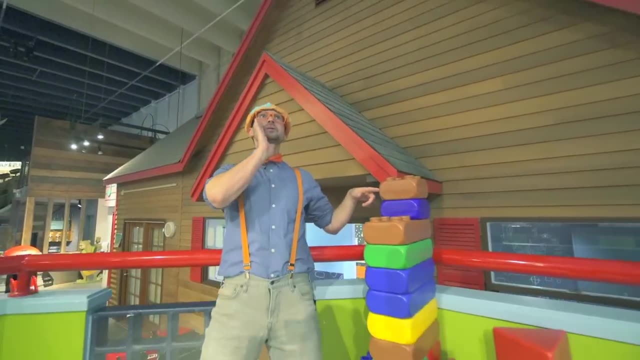 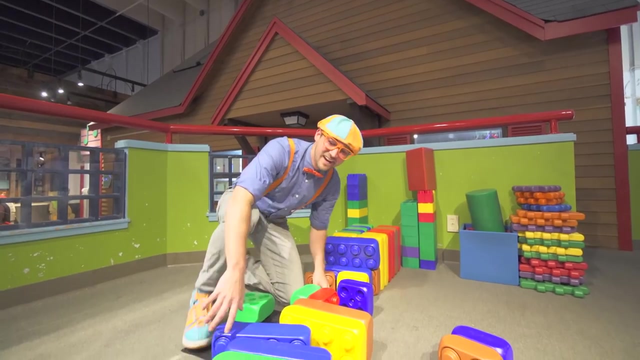 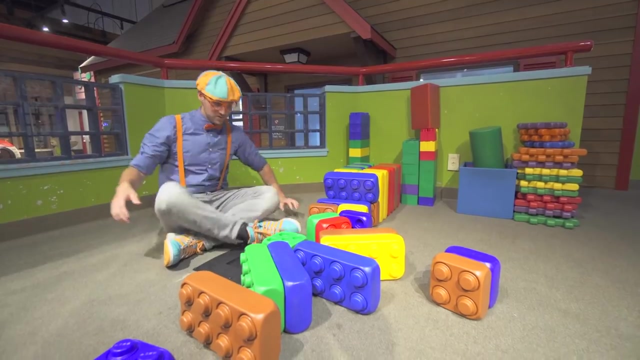 ten: 11,, 12,, 13,, 14,, 15,, 16,, 17, 18.. 18 bricks coming down, Whoa, Whoa. Oh, that was awesome. Okay, let's organize these bricks in their different colors, okay. 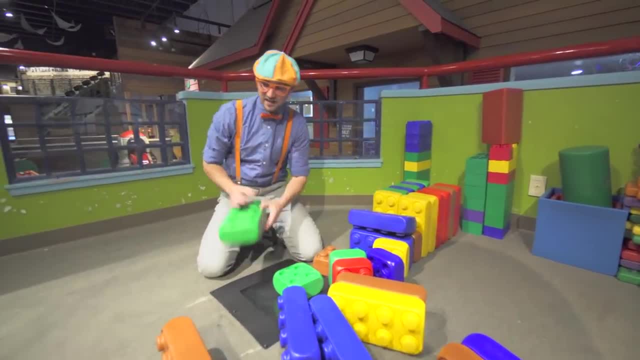 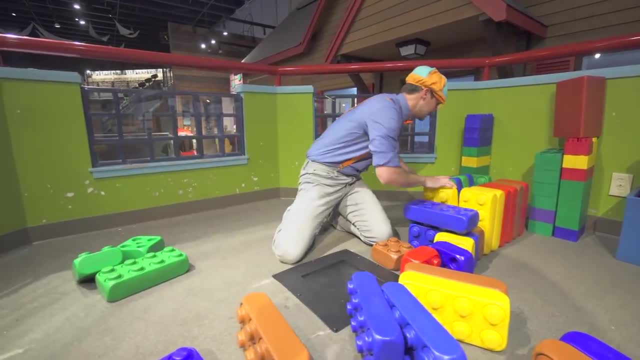 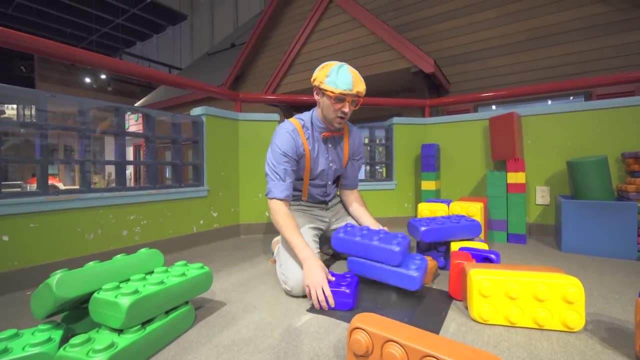 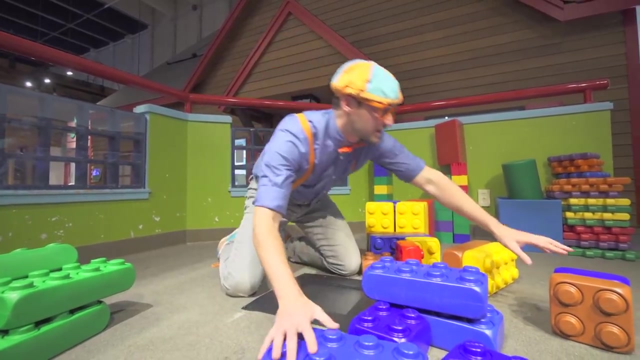 We need to put them over here, Okay. Okay, there's the green bricks, And let's now take the blue bricks and put them right there. And let's now take the blue bricks and put them right there, Okay, Awesome, Perfect. 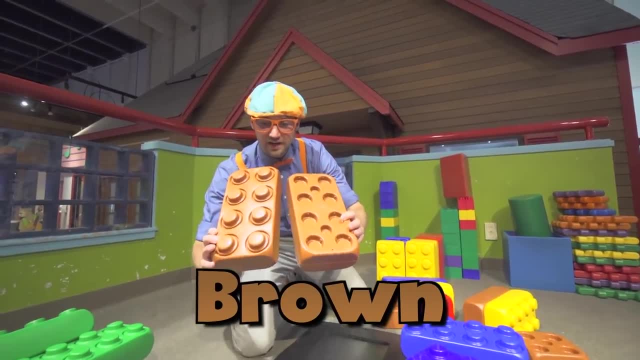 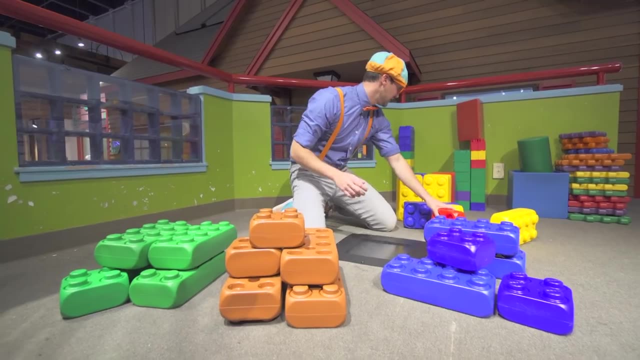 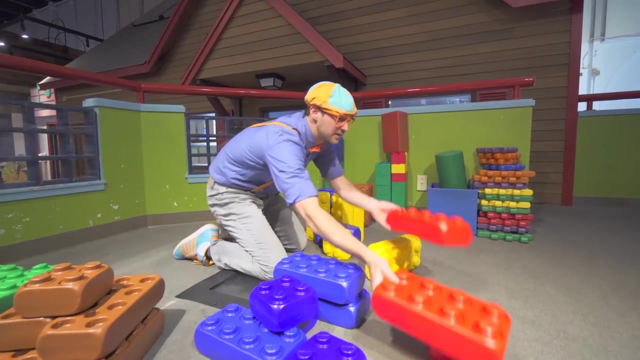 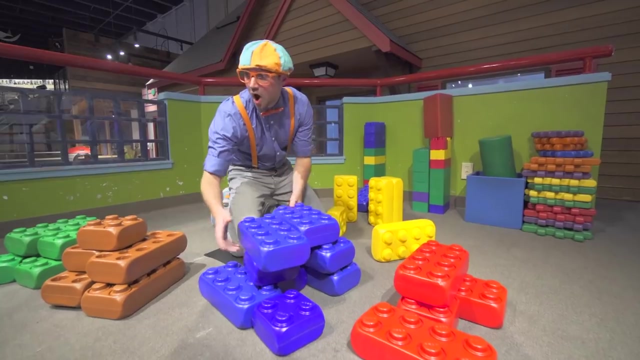 Oh, hey, Look, Here's some brown bricks, Let's put them right here. Okay, awesome, Friendly house. Here's a red brick, let's put it right there. here's some more blue bricks. look at this one. what color is that? 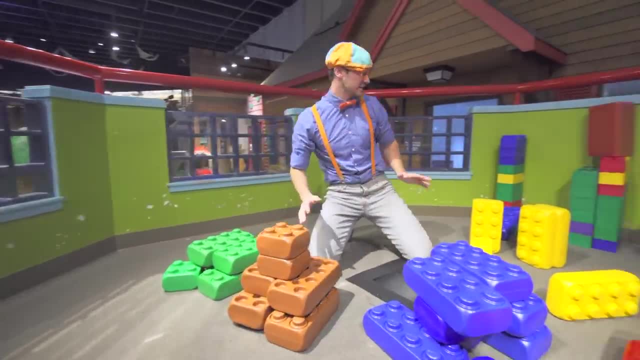 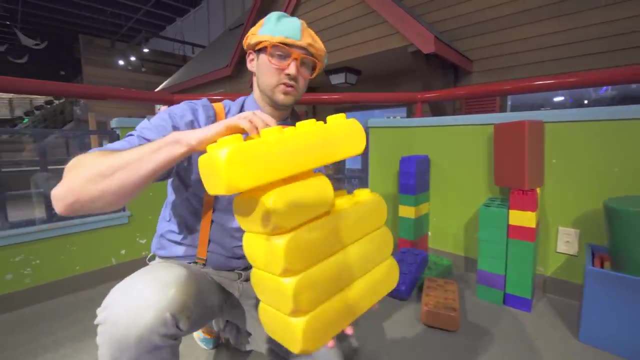 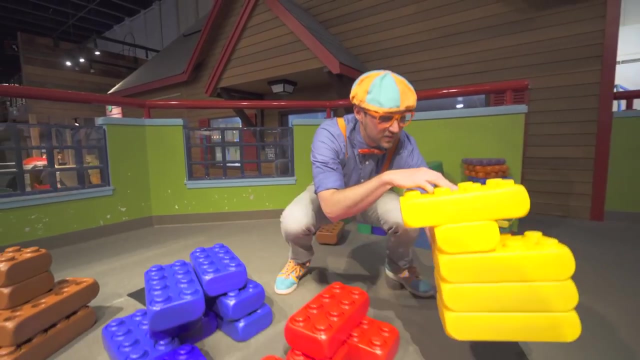 Yeah, this is brown. let's stack it right there. hey, look at all these. what color is this? Do you know what color this is? Yeah, it's the color yellow. let's put these right over here, okay, so when those 18 bricks? 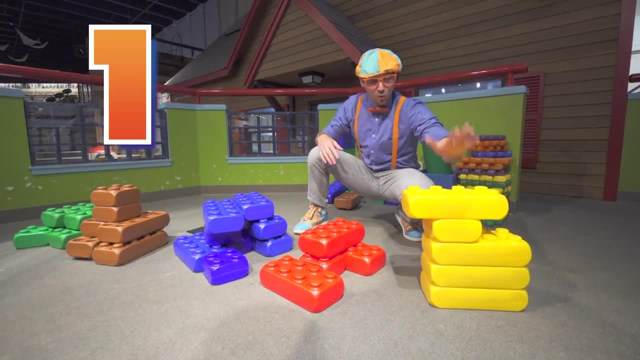 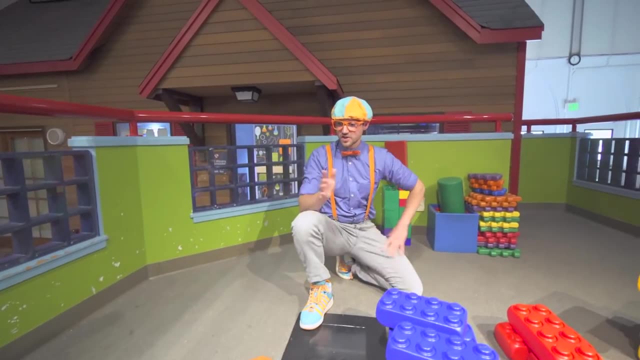 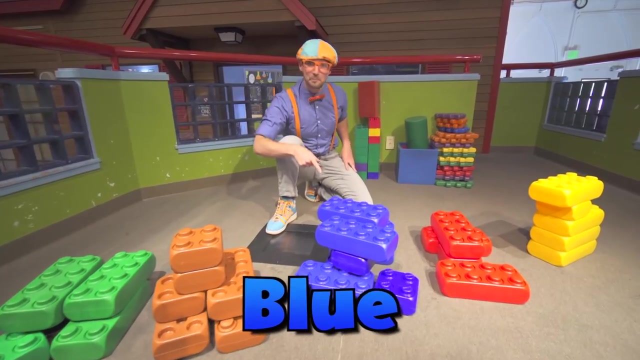 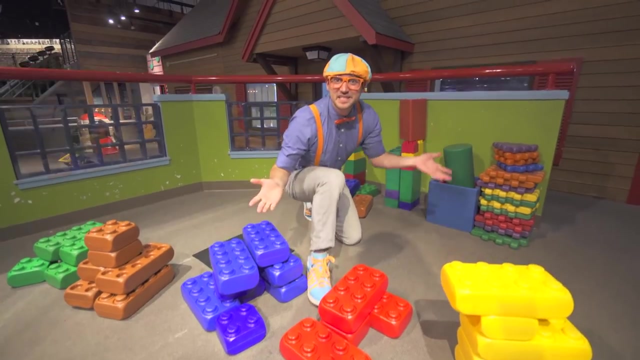 fell down. they were comprised of these one, two, three, four, five colors, and those colors are green, brown, blue and red, Blue, red and yellow. good job, let's see what other fun things they have at the Pacific. 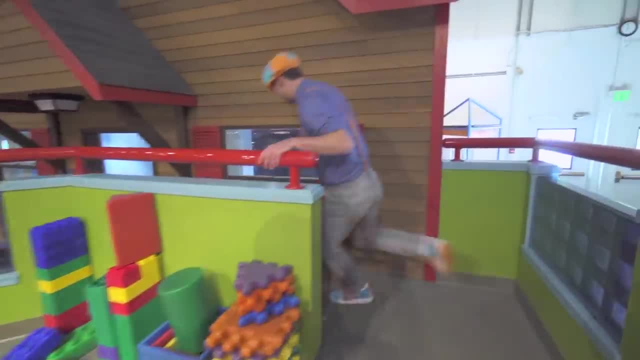 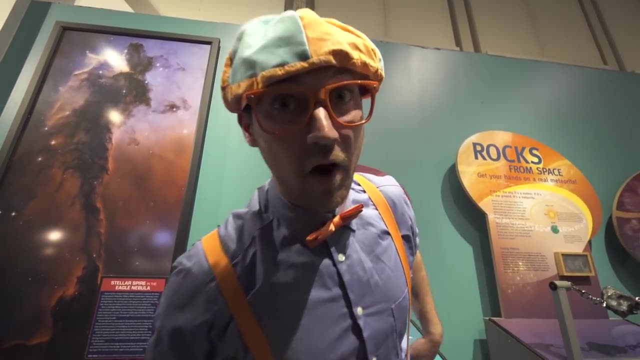 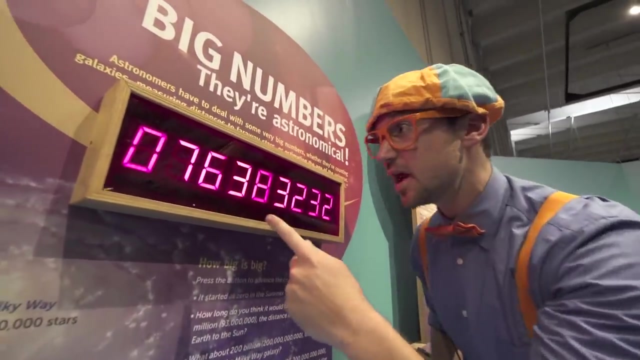 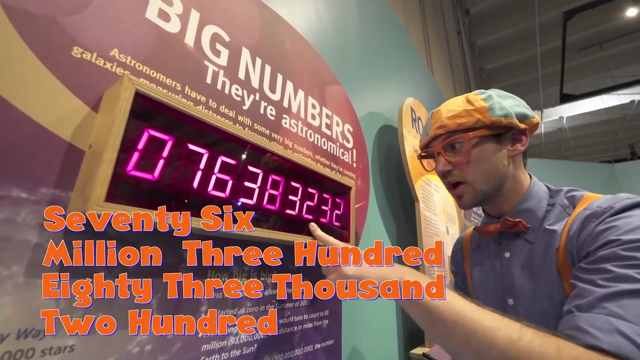 Science Center. let's go. Do you like numbers? Yeah, I do too. what about big numbers? yeah, check this out. this is a big number: seventy six million three hundred and eighty three thousand two hundred thirty two. whoa, that's. 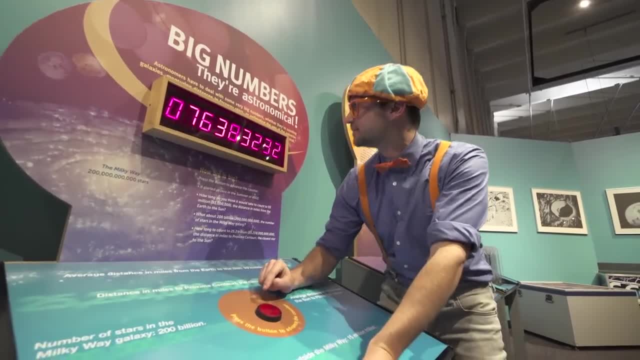 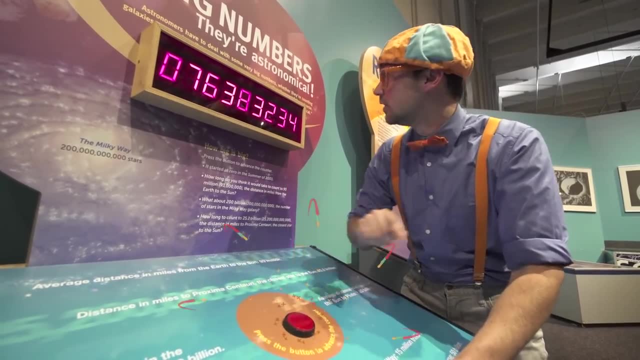 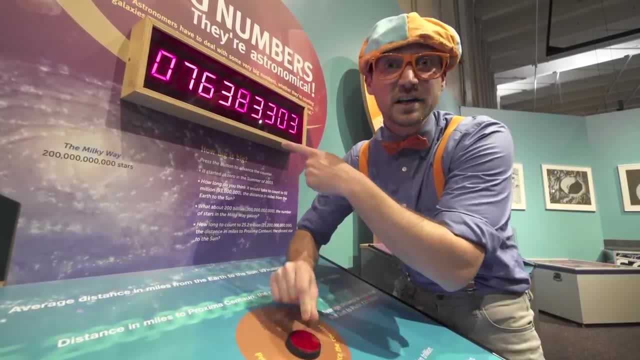 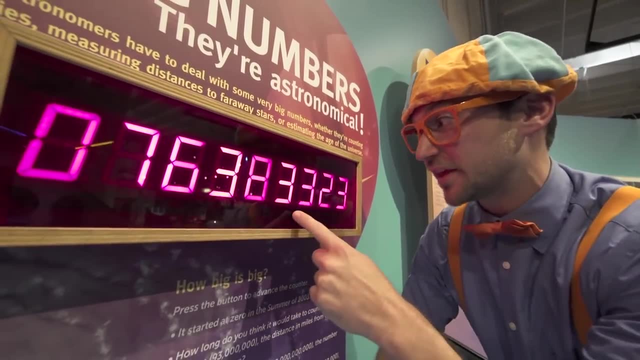 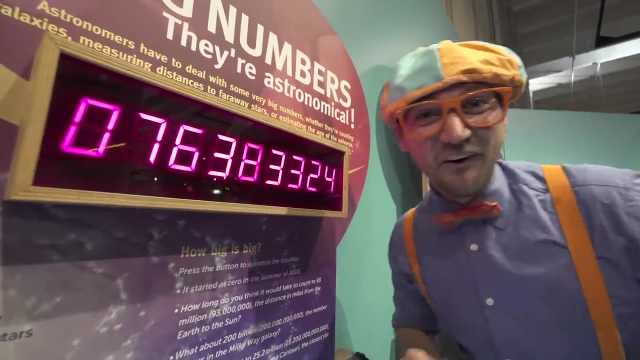 have a lot of fun. So if you ever come to the Pacific Science Center, you can see what number it's at, because I am going to leave it at seventy six million three hundred and eighty three thousand three hundred and twenty three- wait, no, three hundred and twenty four, ha ha. 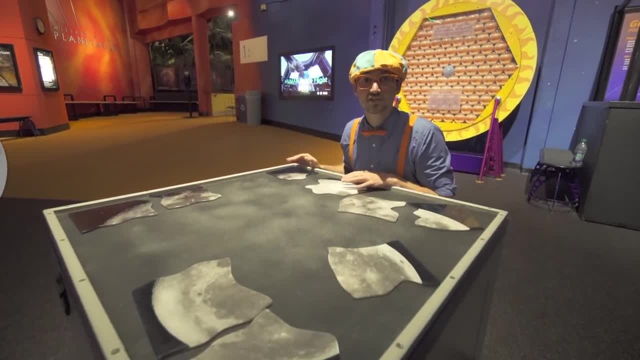 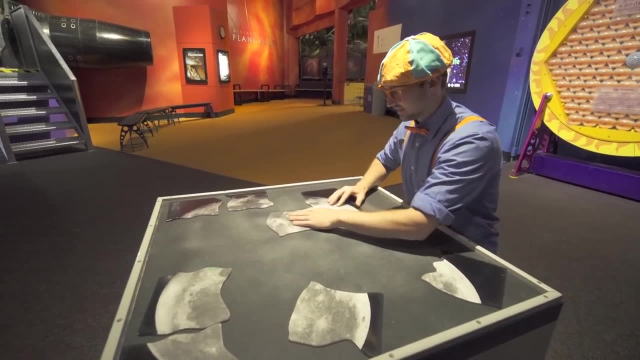 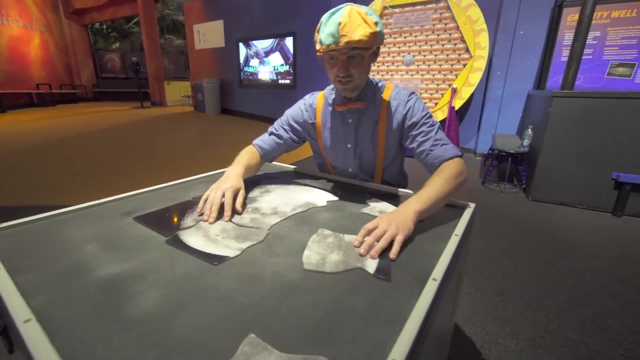 Hmm, hey, I'm just doing this puzzle of the moon. okay, there's one, let's see. hey, there's another. um, yeah, that looks about right. perfect, we're almost done. look, yeah, this. 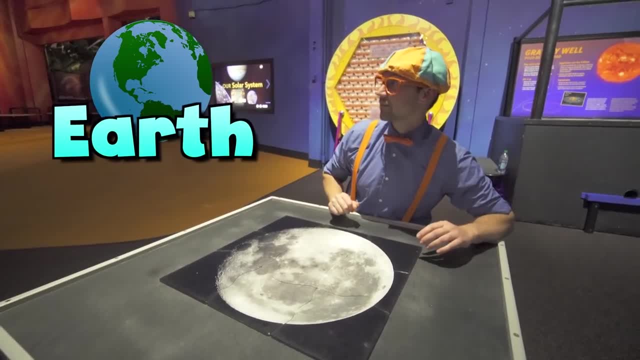 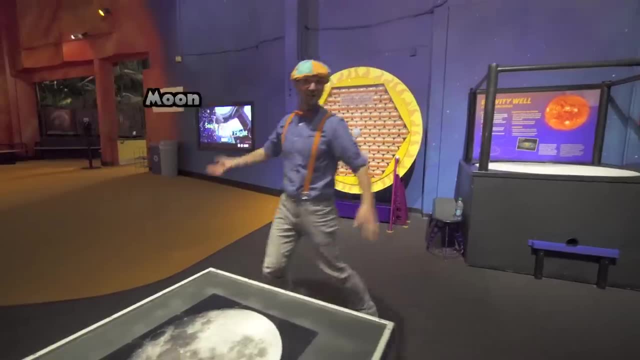 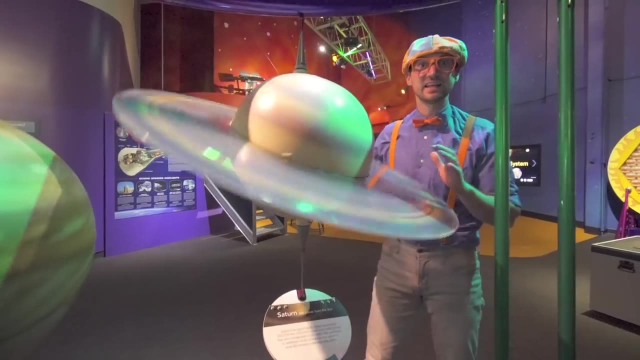 is our moon. we live on planet Earth and we have one moon and we call it moon. ha ha, wow, how clever of us. hey, look at what it is. this is a planet, just like how we live on planet Earth. 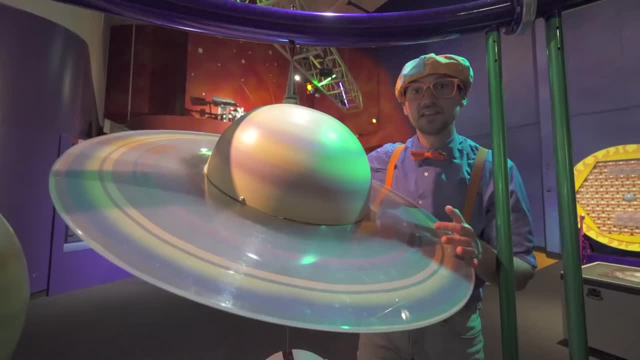 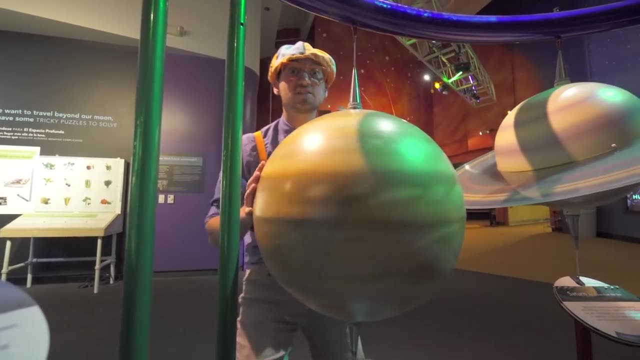 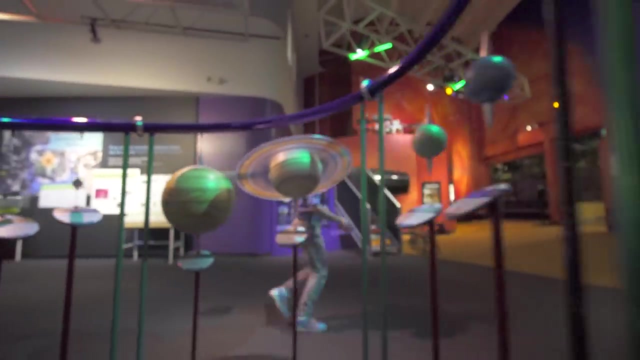 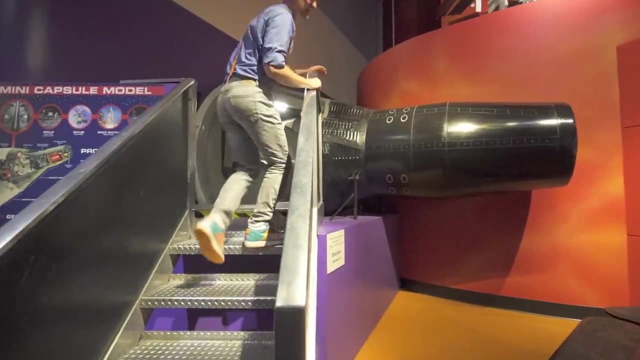 This is a planet in our solar system and this is Saturn. oh, and the biggest planet in our solar system is Jupiter. whoa, it is really big. look at that. come here, this is a space capsule. watch your step, see. this capsule is where astronauts can see the 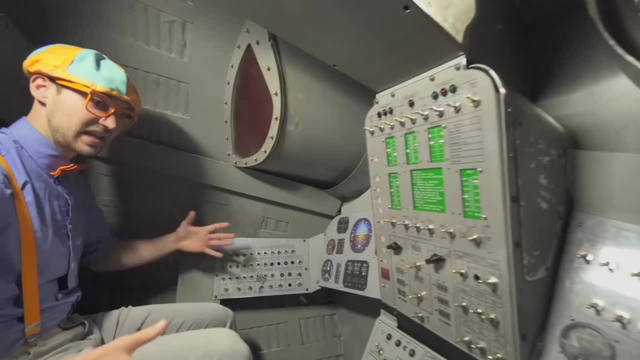 Earth around them and Sophia has a great personalatamente pair. your Friends the Earth and very happy in our Mars virtual space capsule And then they can sit in and go into outer space, so then they can feel the effects of gravity and they can push all these cool knobs ready. 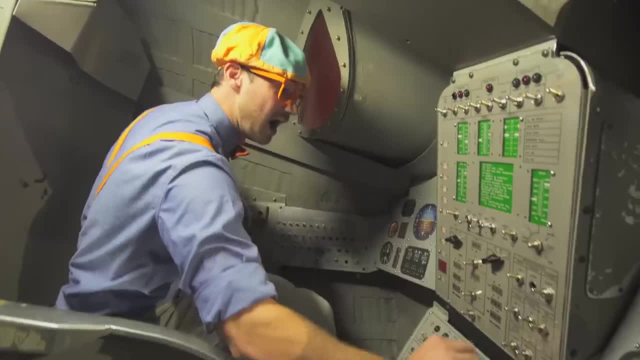 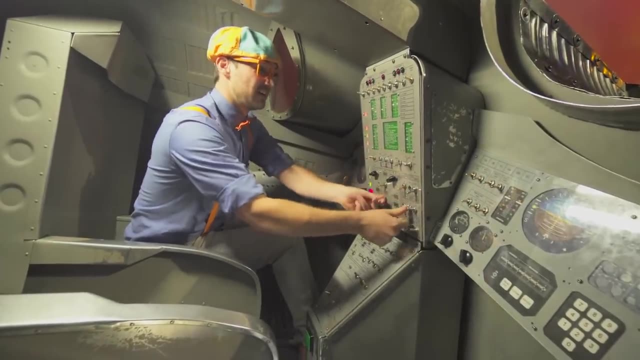 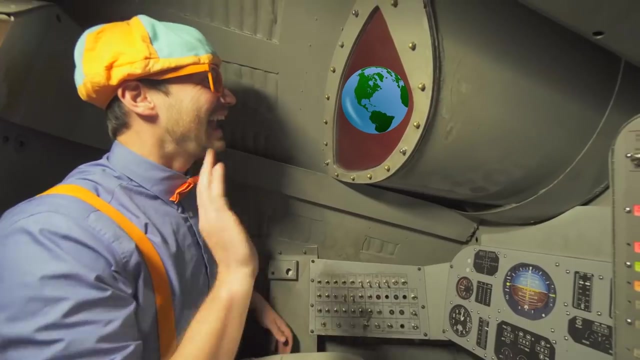 Whoa, Yeah, look, I just made all those things light up. Whoa, this is fun. whoa, it's like I can see planet Earth all the way from out here. Whoa, hey, mom Woo Woo. 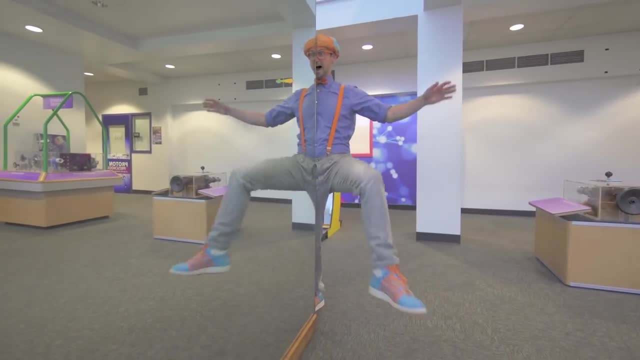 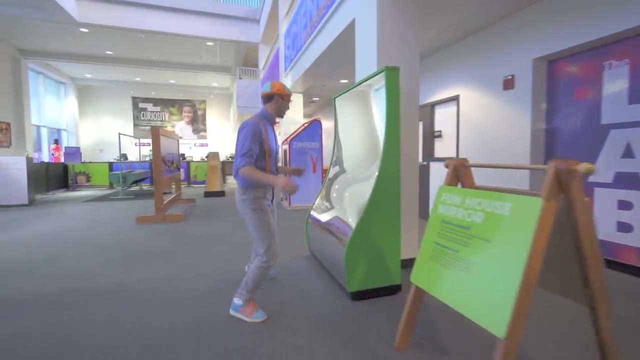 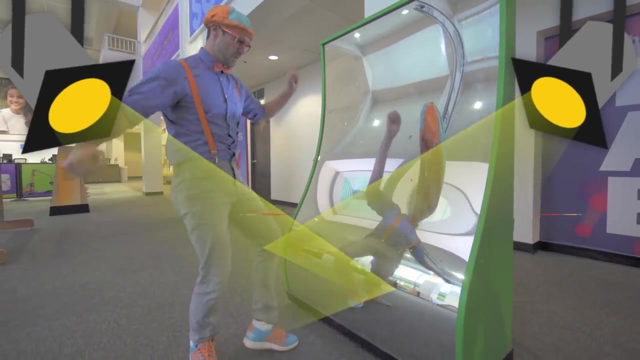 Whoa, Whoa, Just kidding, it was just a mirror. Come over here, I'll show you some more fun that we can have with mirrors. Ooh, look at this. Whoa, I call this the mirror dance. I look silly. 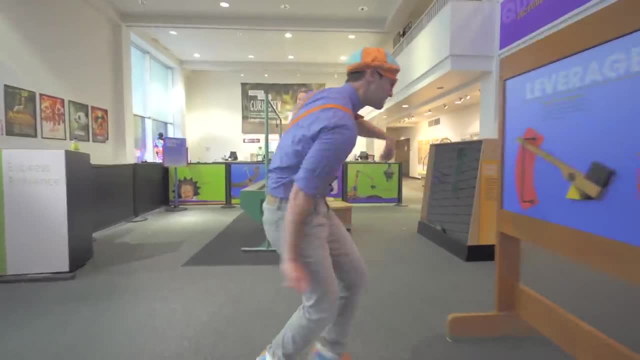 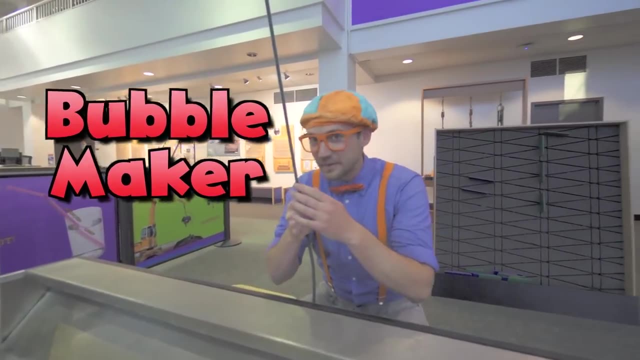 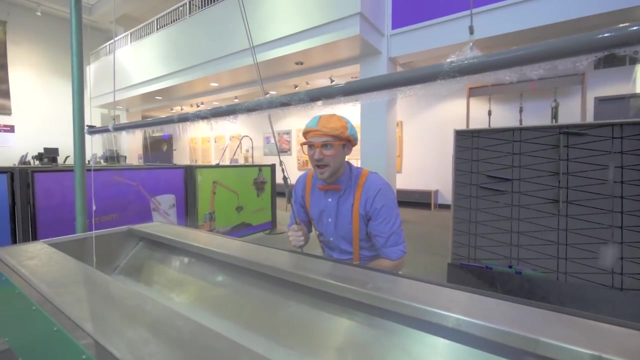 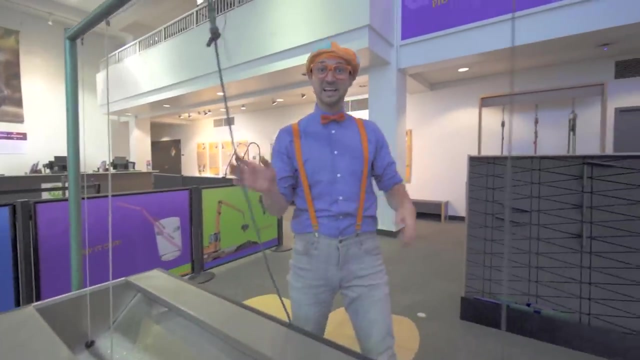 Come on, Come on, Ooh, This is a bubble maker. All right, I'm gonna lift this up Nice and slow And I'm gonna blow now. Yeah, I did it. Did you see that? That was awesome. 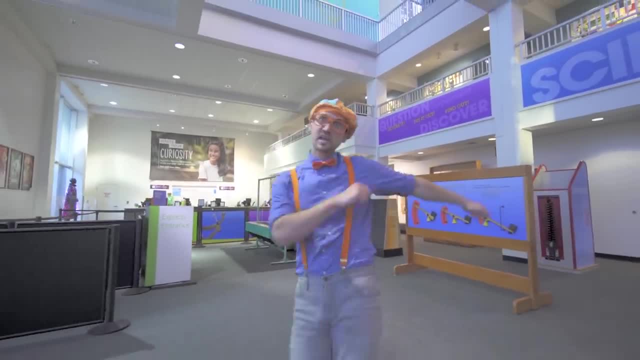 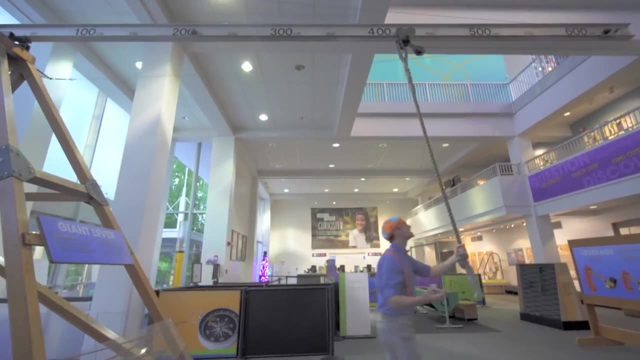 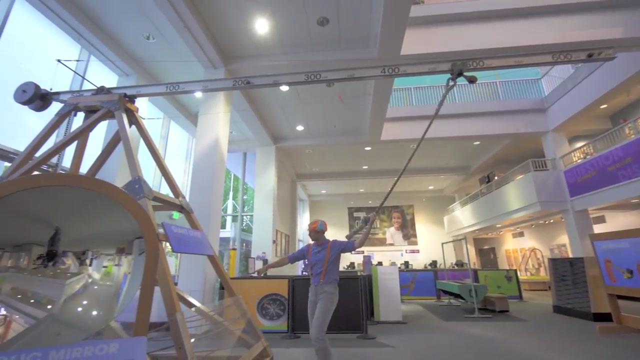 I love making bubbles, Ooh. and you know what else I love Is taking a giant lever and seeing how distance way out here makes it really easy compared to to lift up this weight, compared to down right here- See watch. 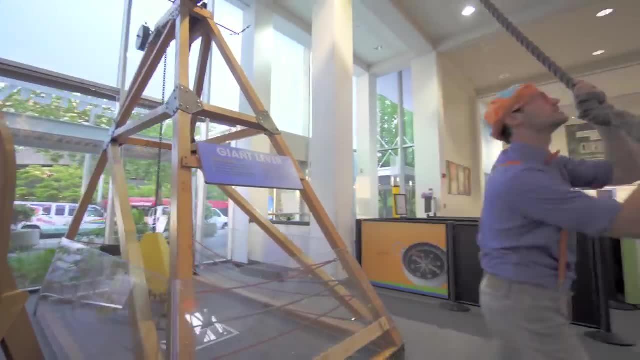 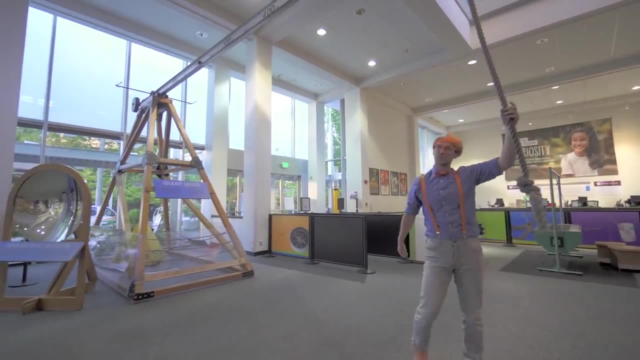 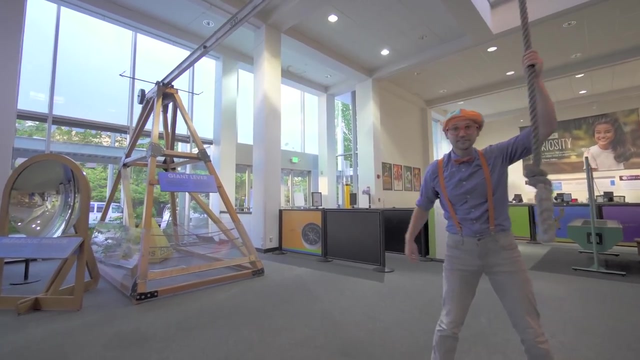 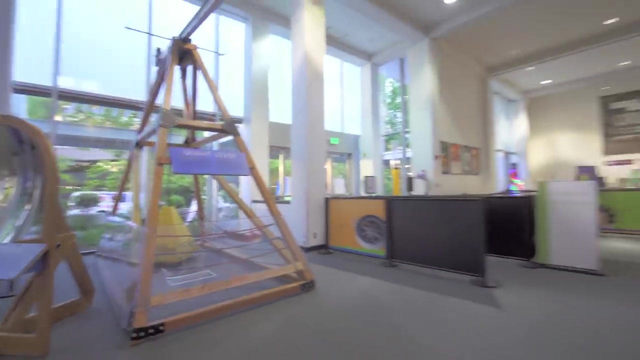 Huh, interesting. All right now, let's move it way out here. All right now, I'll do it with one hand. Yeah, did you see it? Look, I'll lift it up. Whoa, that's pretty interesting. 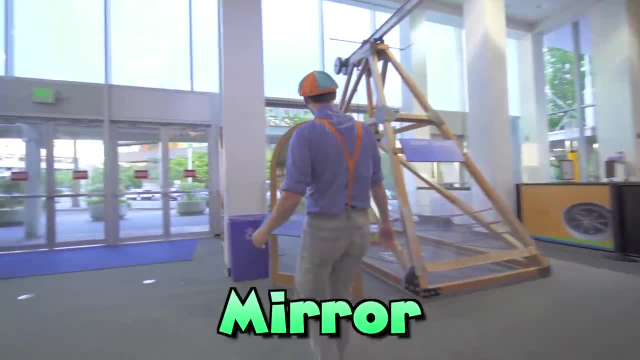 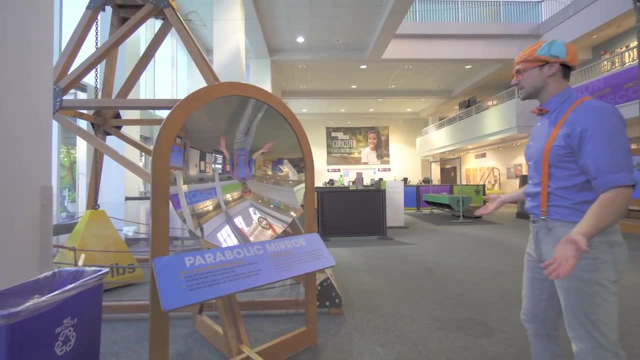 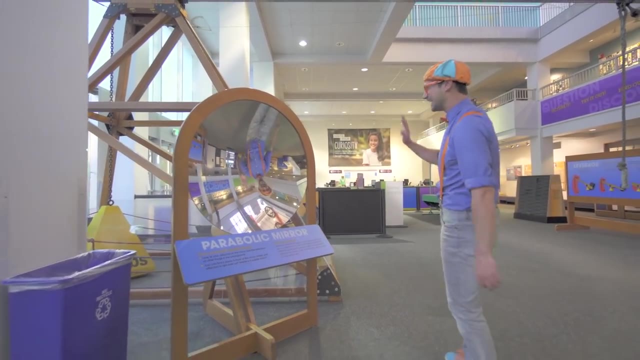 Whoa, hey, a cool mirror. Another one, Hey, hello. This is interesting, See, I'm upside down, But in real life I'm right side up. Hello, Hey, I see you. Whoa, Whoa. 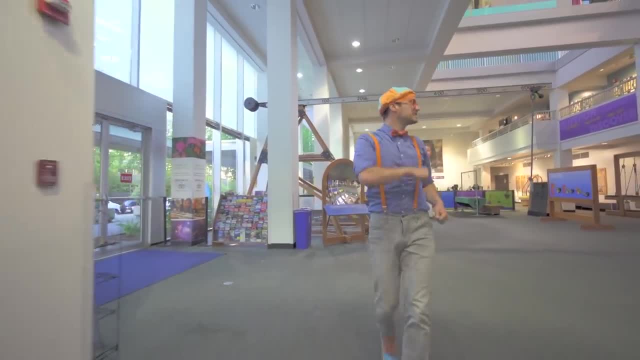 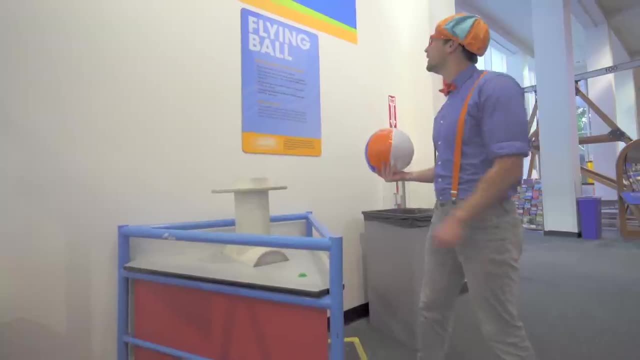 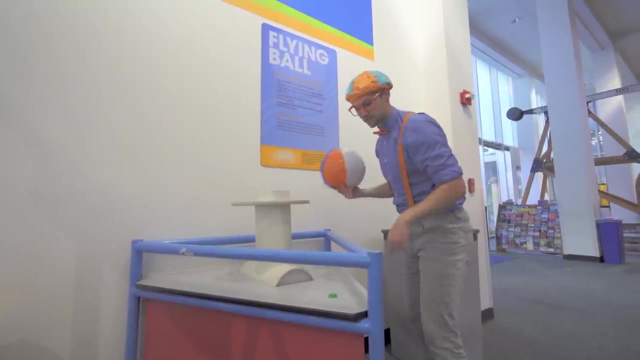 All right, let's continue on. This place is so cool. Hey, what's this? This is a beach ball. What's it doing here? Flying ball, Flying ball, It's the power of air in motion. Huh, interesting. 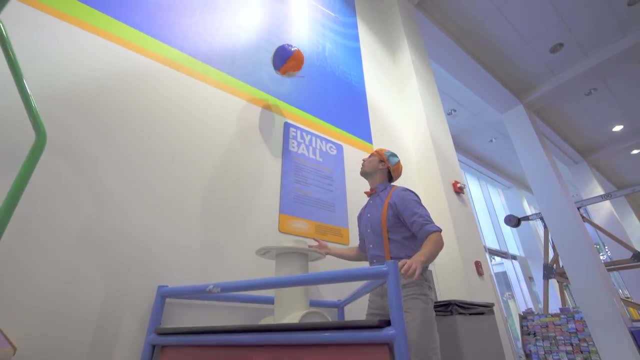 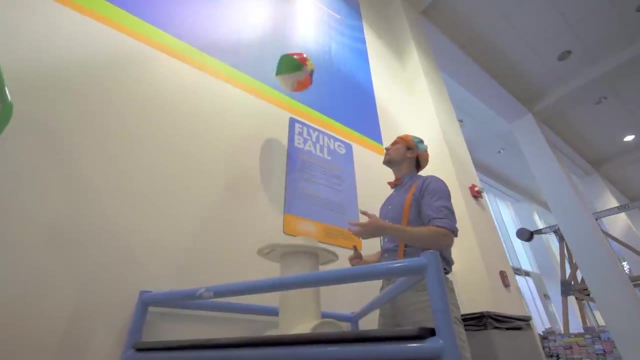 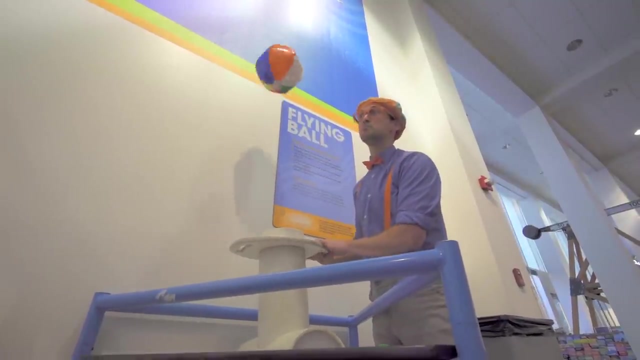 Let's push this. Whoa, I wonder what happens when I plug this hole that's shooting up all the air. Whoa, did you see that? All right, Now I wonder what happens when I move it? Whoa, Oh, look, the ball's way over there. 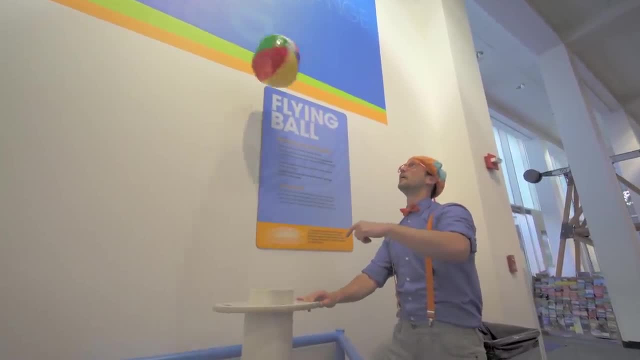 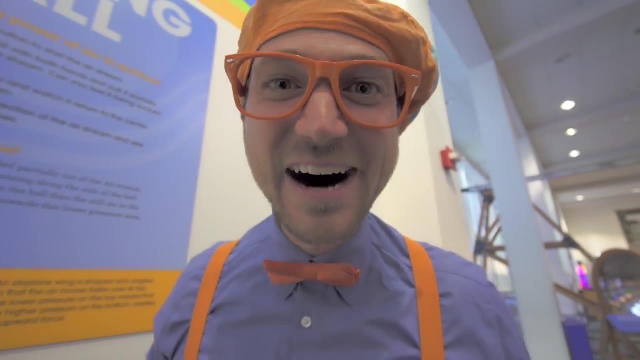 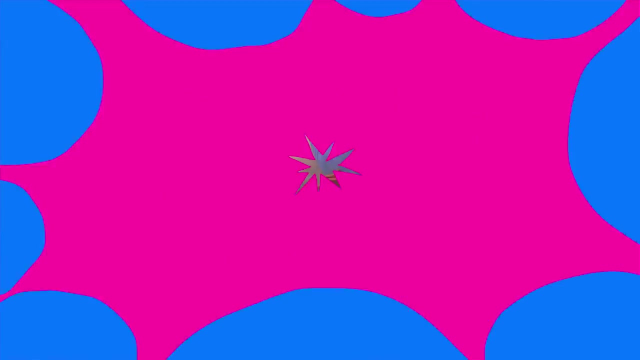 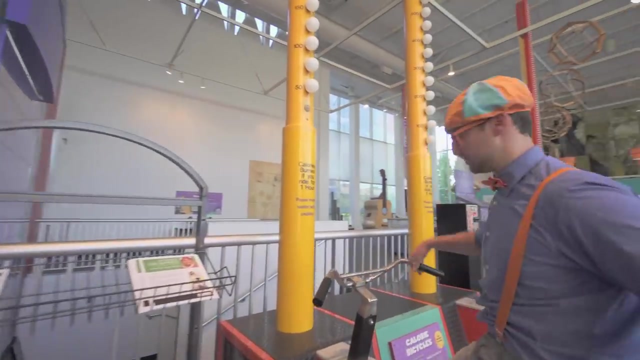 All right, Here we go, Ready, Whoa. Yeah, That was awesome, Ah yum. I just hydrated my body with a lot of water because what I'm about to show you takes a lot of energy. I'll show you. 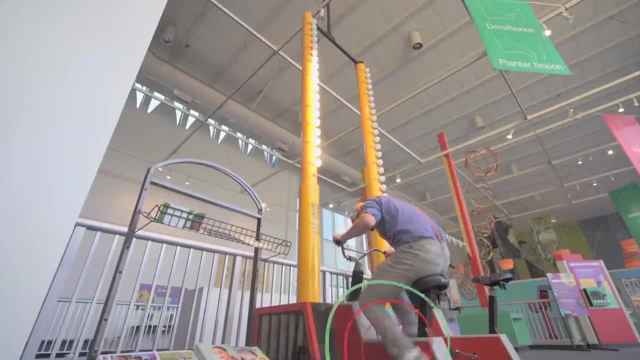 My Lance Armstrong water bottle. Lance Armstrong hill climb- Woo-hoo, That was awesome. Well, this is the end of this video, but if you want to watch more of my videos, all you have to do is search for my name.